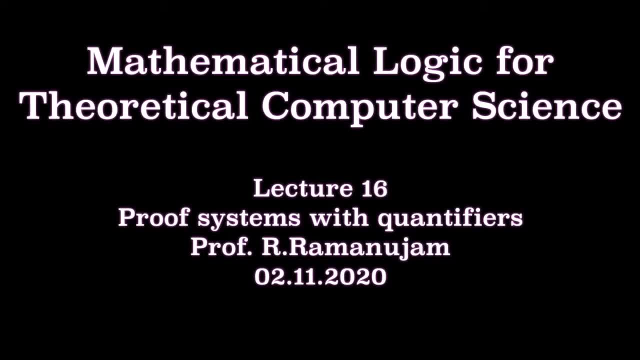 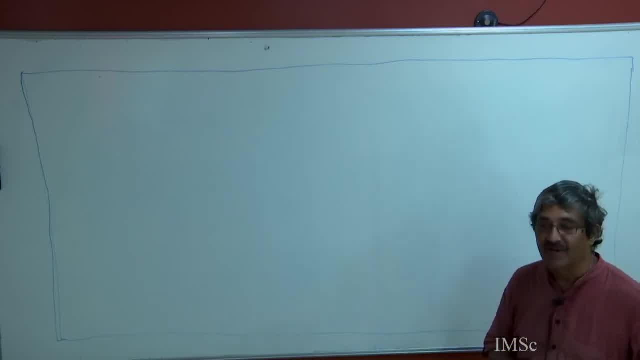 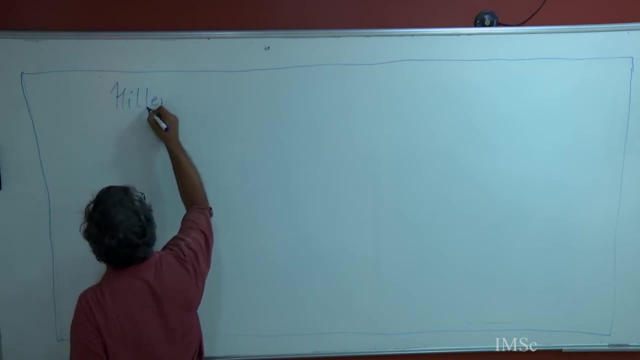 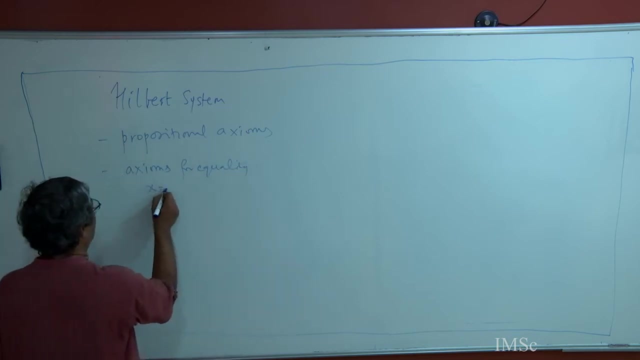 Yeah, so we were talking about proof systems with quantifiers and I'm going to continue that. Last time we saw the famous Geerdel completeness theorem. So this is the Hilbert system, where you have the propositional axioms and then axioms for equality, which is x equals x. 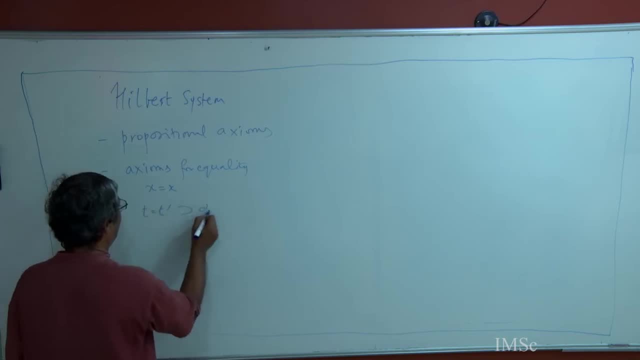 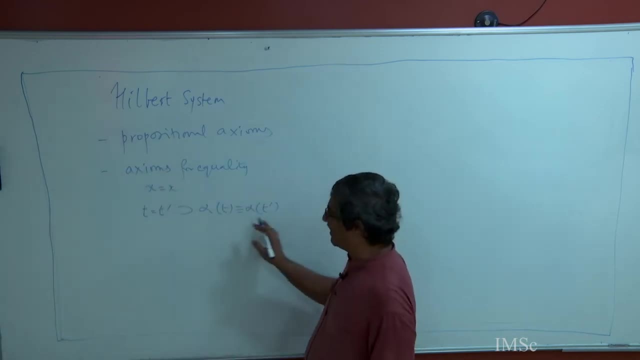 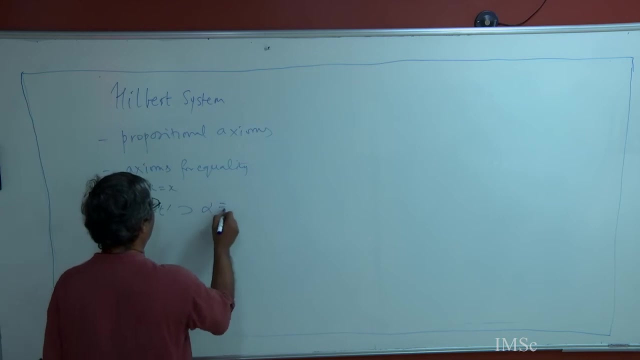 And t is equal to x. t equals t prime implies alpha of t is equivalent to alpha of t prime. This is the notation, but actually what we have in mind- and that is how I prefer it- is alpha equivalent to alpha prime, where alpha prime is got from alpha prime. 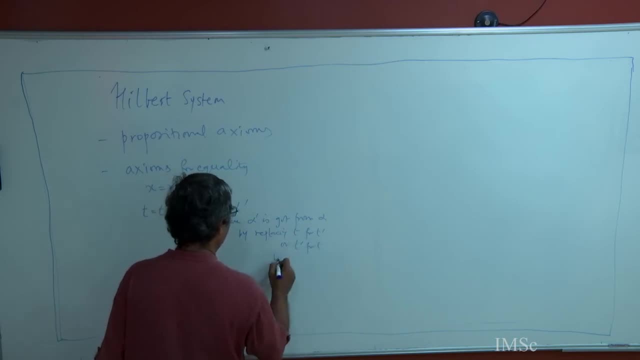 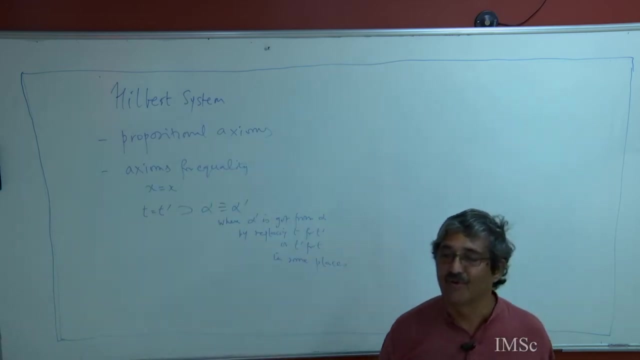 or t prime for t in some places. And this is important because you do not have to uniformly replace right. The substitution of equals for equals you can carry out everywhere, anywhere. Remember in school this is what you do: LHS and RHS. you find substitutions, you find equivalent. 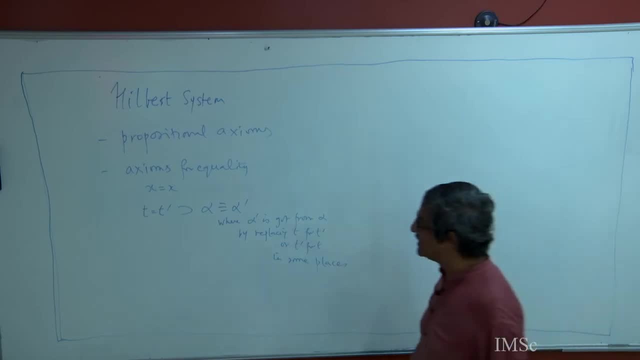 expressions, you substitute them anywhere. So that is the and this is the, with two of the, The, these two. 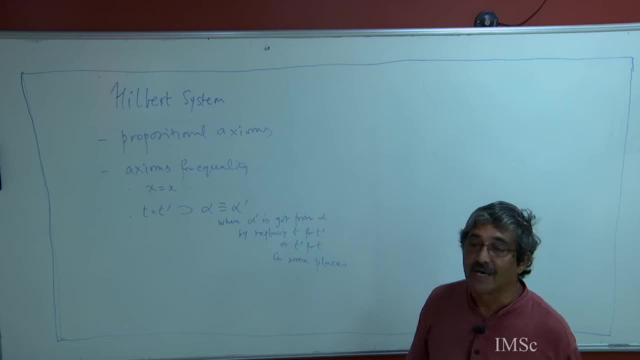 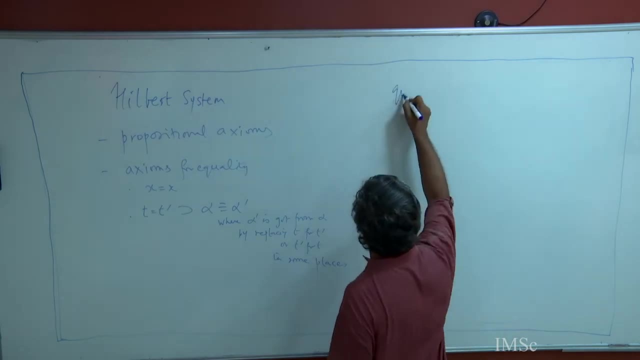 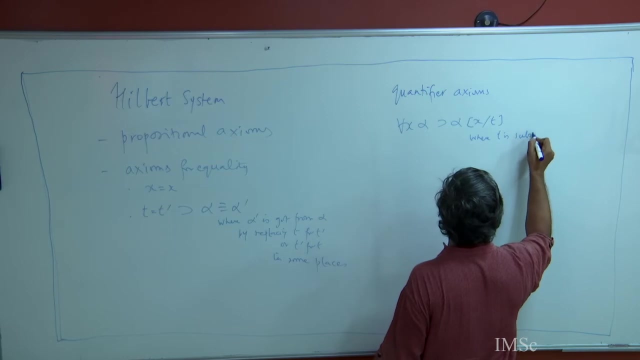 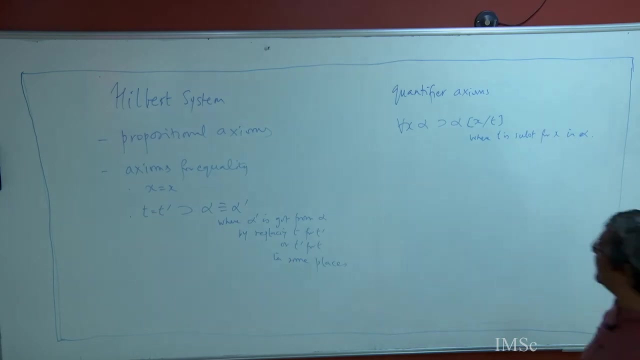 axioms you can derive whatever you need, especially to show that the equality is a congruence in the completeness proof And then quantifier axioms. So this is for all x. alpha implies where T is substitutable for x in alpha and alpha implies for all x alpha when x has no. 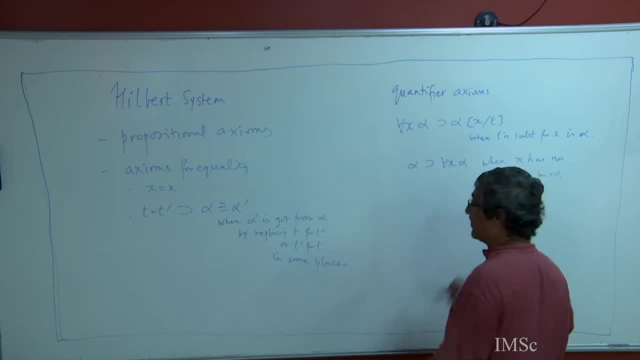 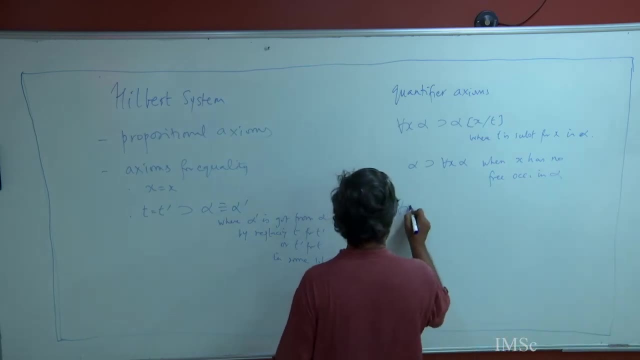 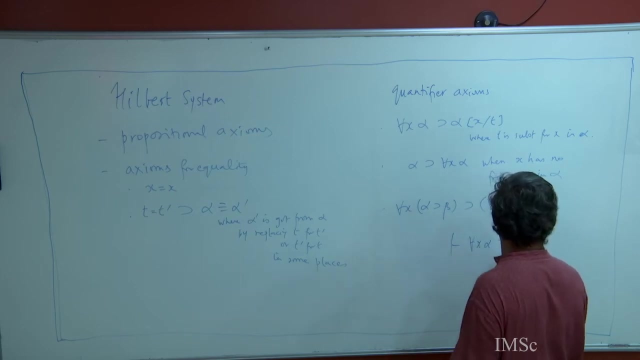 free occurrence in alpha. if x is not occurring, free alpha will imply for all x alpha, Thank you. and then distributivity for all x. alpha implies beta, implies yeah, And, as we saw, all these are actually used to derive something which is fairly innocuous but which is really bound. 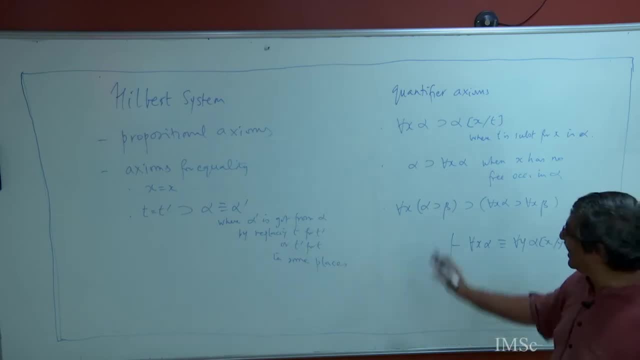 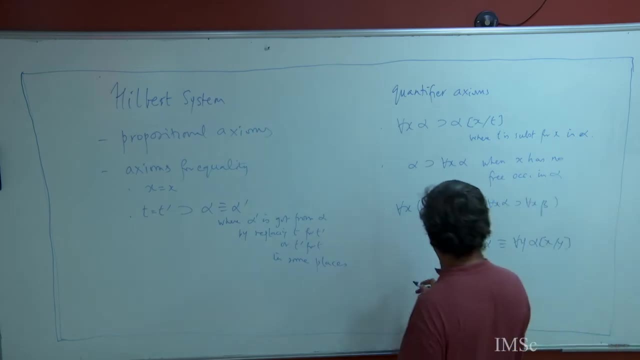 variable renaming right. To derive this, we used all the three axioms and from that then we actually show that whenever gamma derives alpha, with x replaced by y where y is new, then yeah, this is the generalization from constants, but written for variables, and that is it. and 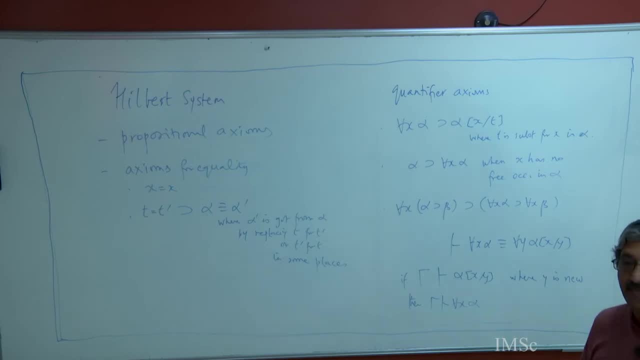 with that we can actually do the completeness proof So well. last time I went through it, I mean, the Gerl completeness theorem is a big thing, But I thought, since we are really seen the proof of the compactness theorem in some detail and it is pretty much the same argument, Everything repeated wherever we were doing for FinSAT. 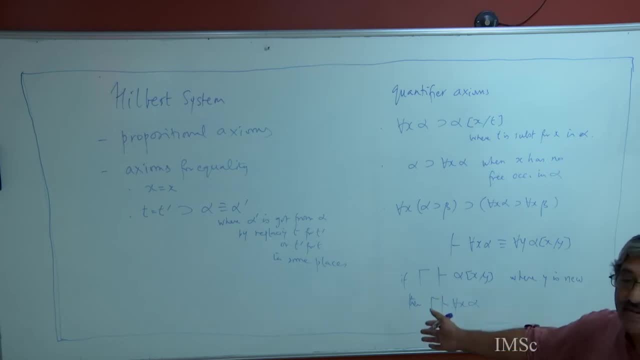 you are repeating it with consistent and now, of course, you have to show derivations and that is it. with this u, the whole thing goes through ok, And the only different way that I did it was that, rather than expanding the language and working with constants and so 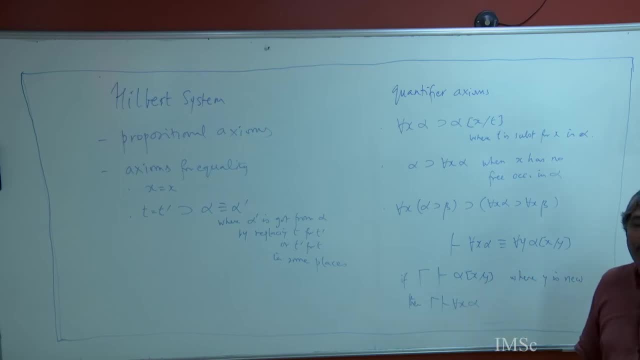 on. you can simply use variables right. So for fulfilling, for witness fulfillment, you just make sure that if there exists x, alpha belongs to gamma, then alpha with x replaced by y belongs to gamma, where this is a new variable. How do you ensure that new variables? 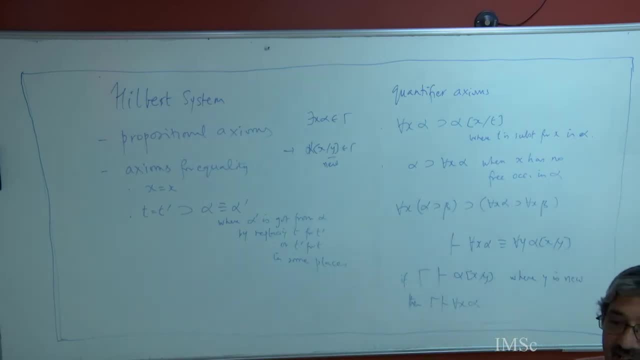 are available. You start with whatever given consistent gamma, rename all your variables so that you have countably many variables available and do that, And you have to show that that is consistent where your little bit of trickery is involved. but then everything goes through smoothly. So this was the message of last time and so this proves the completeness. 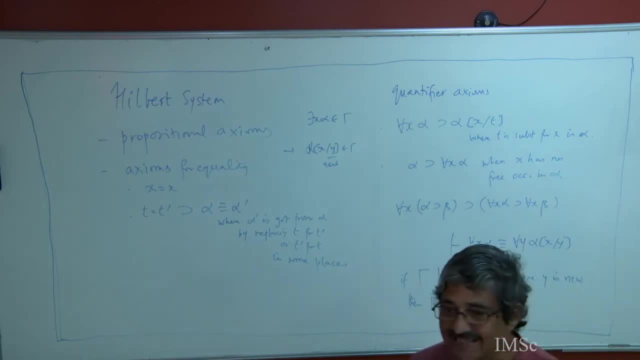 of this system and but, as I said, you know Hilbert systems, doing proofs is always problem, and, And with quantifiers, of course, it is even more of a mess. What I want to show you is to how we would take up all these things with natural reduction and sequent calculus, and 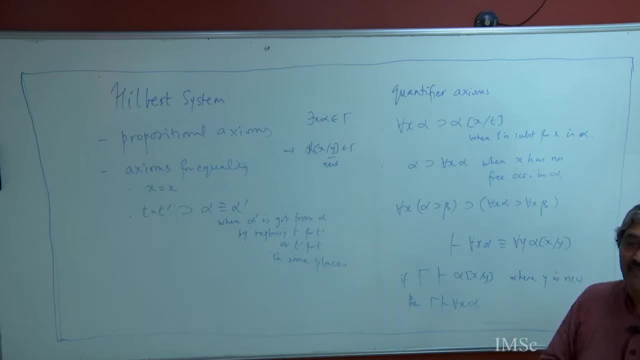 also resolution, which is: these are the things that we did for propositional logic. So I want to show what: how quantifiers, how all these proof systems, work with quantifiers, With resolution towards the end of that lecture. So I talked about how you do it with quantifiers, but I am sure that was you know, it is just. 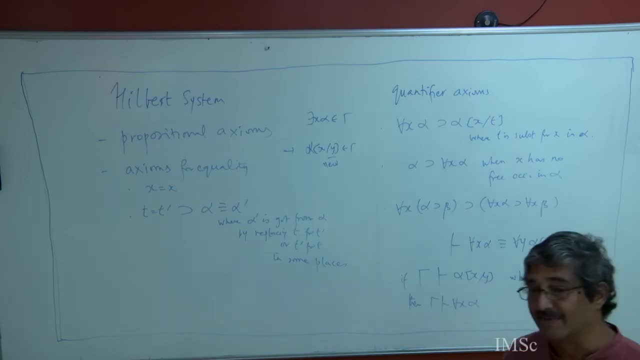 a zip through, So we will do it a little more slowly. the but because that is a fairly interesting and important thing and normally not discuss much in mathematical logic, but for automatic theorem proving, that is perhaps the most important engine. ok, So let us look. 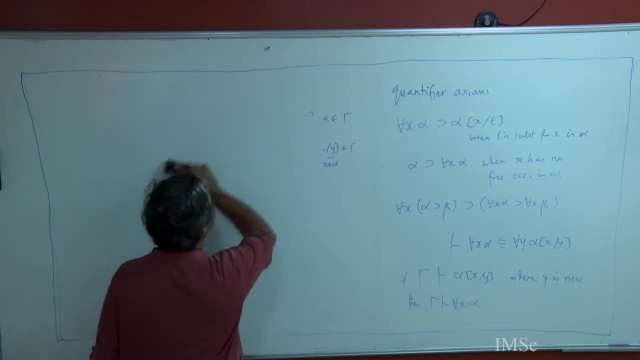 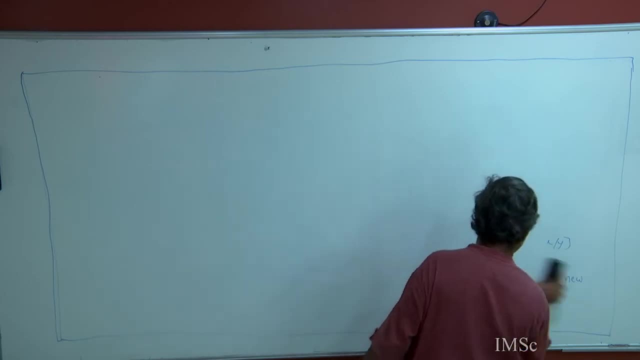 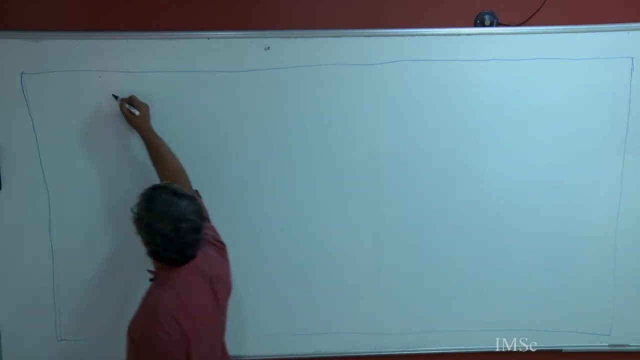 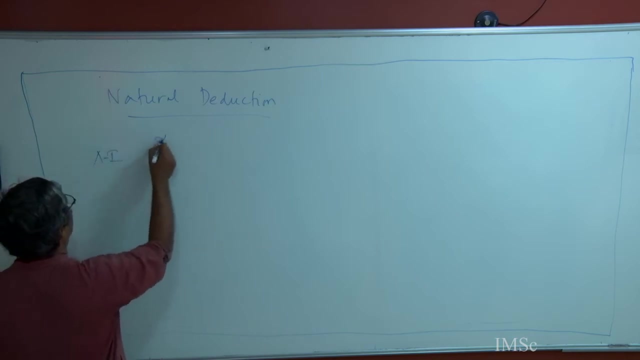 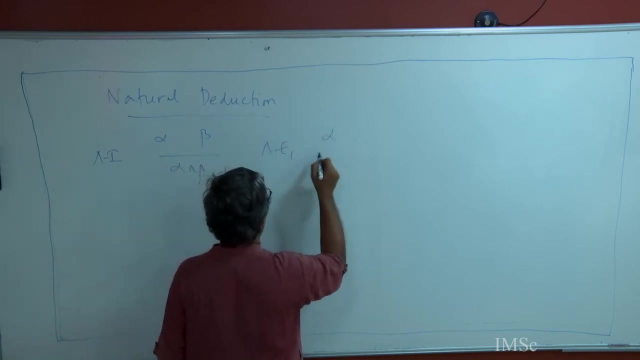 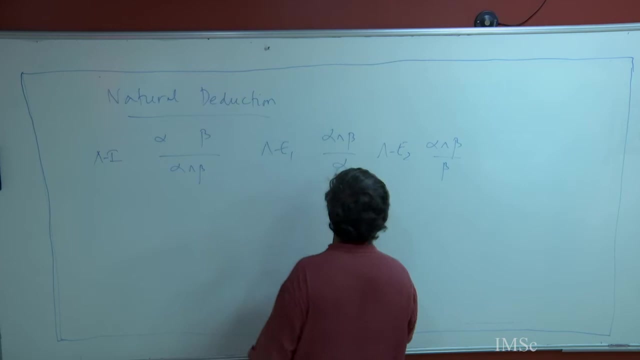 at natural reduction first. OK, What are the rules for the natural reduction? You have introduction rules and elimination rules. Yeah, natural deduction. and what are the introduction rules? and introduction? if you have got alpha, you can get alpha and beta and elimination 1 and elimination 2, right, fairly obvious. 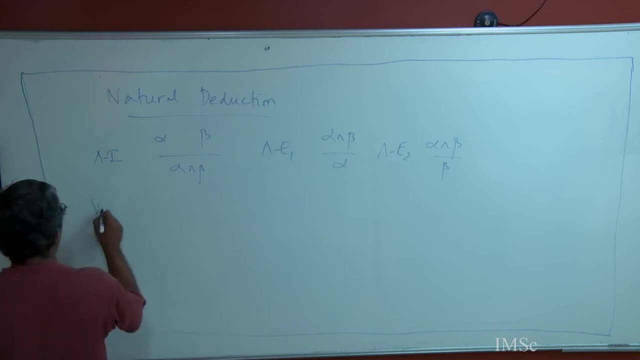 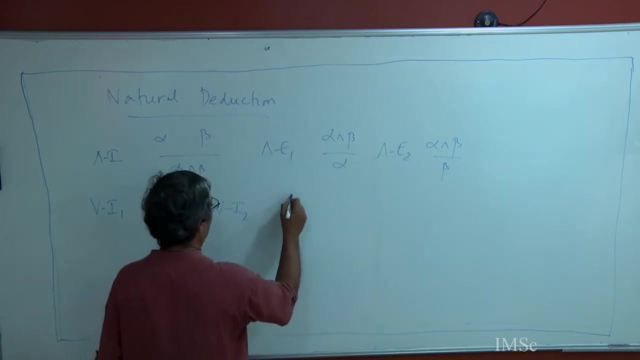 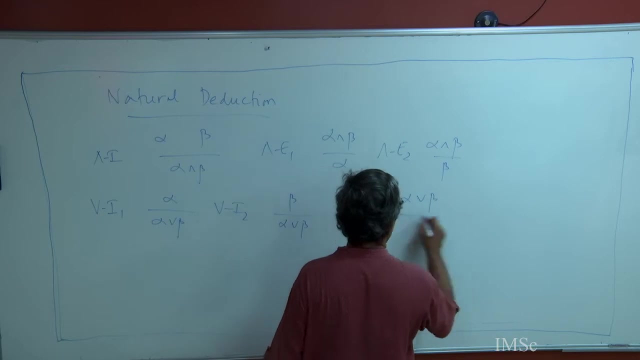 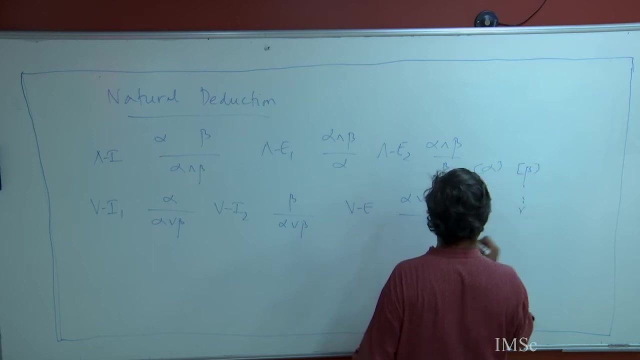 And then for disjunction you have two disjunction introduction tools- not alpha, of course, but alpha- And then disjunction elimination. is slightly weird: if you have alpha or beta. from assuming alpha, if you can derive gamma. assuming beta, if you can derive gamma, then 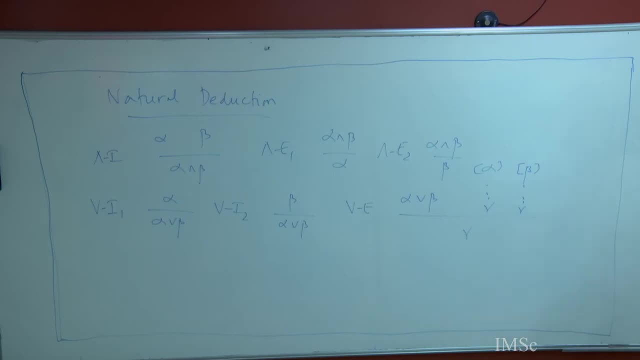 you can derive gamma. yeah, This is the disjunction: elimination and natural reduction. And, like I said, you think of this as case analysis. consider the case where beta is not alpha. You say either alpha holds or negation alpha holds. In the first case, I show gamma and 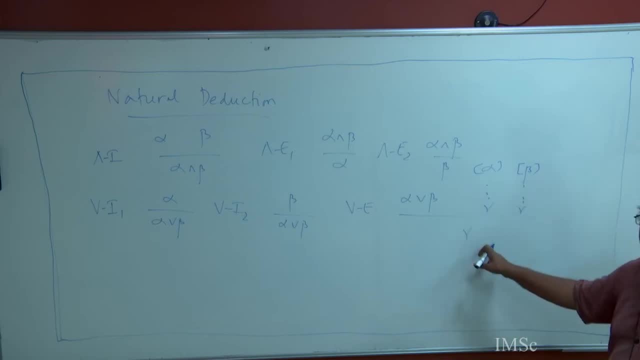 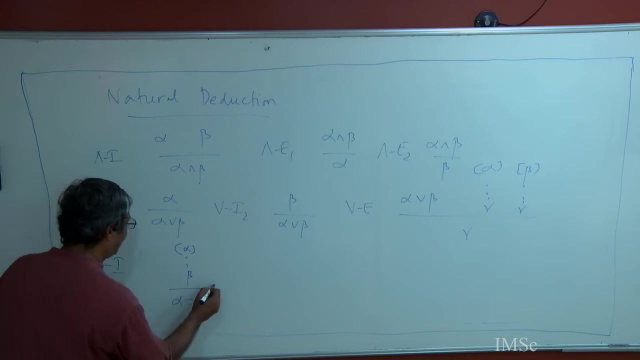 in the second case I show gamma. So in all the cases gamma holds therefore right. This is the justification for that And, of course, all these rules are sound Implication introduction. well, if you assume alpha and derive beta, then you can derive alpha and beta discharging. 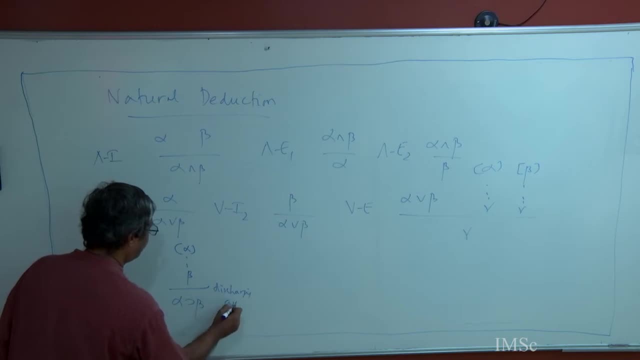 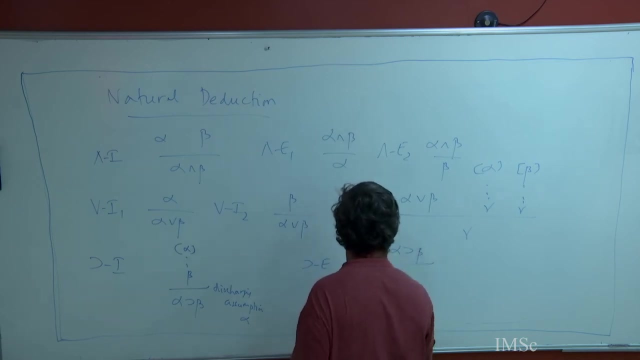 assumption: Yeah, partnerships, Just like mid descent. You make an assumption and you discharge it by introducing implication, and implication elimination is the same as modus pon�. if you have got alpha implies beta. whenever you have derived alpha, you can also derived. 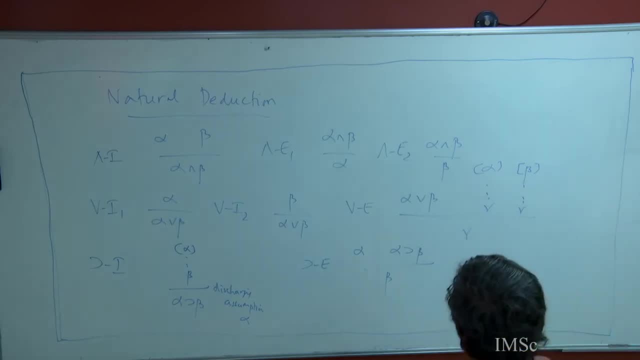 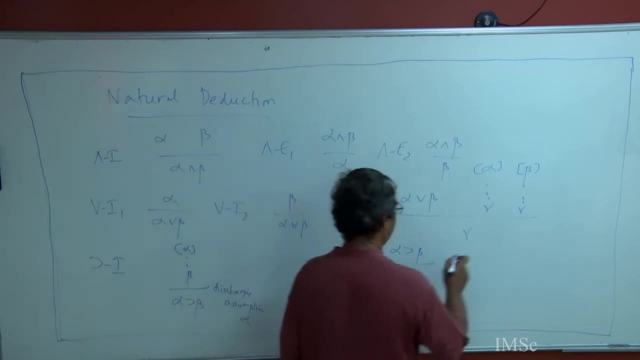 So that is the. and then you have negation. So negation introduction, negation elimination, maybe I can get that right. Subjection subset, Subjective subset, sorry, Subjective subset of knowing, andťáота, maybe I can write it here. What is negation introduction? Well, I do not even remember. 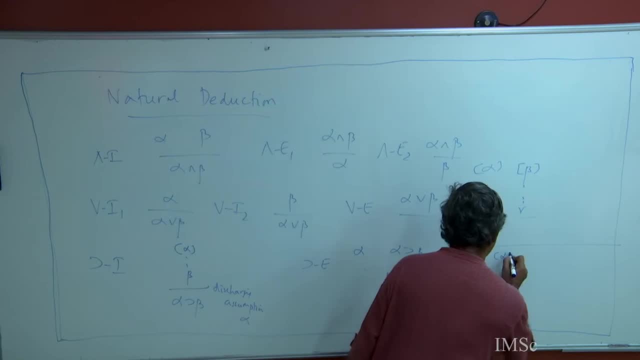 in what form I did it. If from assuming alpha I get beta and assuming alpha I get not beta, then I can have not alpha, not elimination. assuming not alpha I get beta, assuming not alpha I get not beta. Basically, once this is the reductio ready, Reductio ad absurdum. 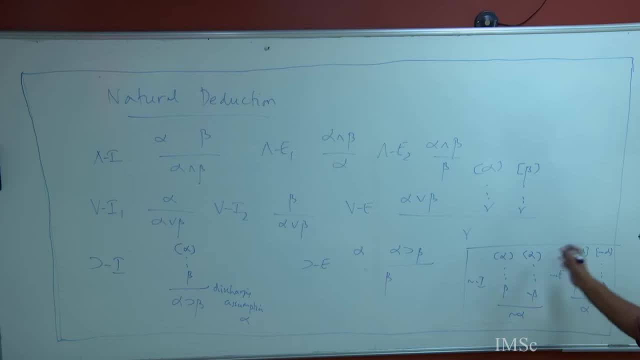 Assuming alpha: if I can get a contradiction, I can get negation alpha. assuming a negation alpha: if I get a contradiction, I get alpha. yeah, So this: negation introduction, negation elimination. So these are all the rules that we have seen. 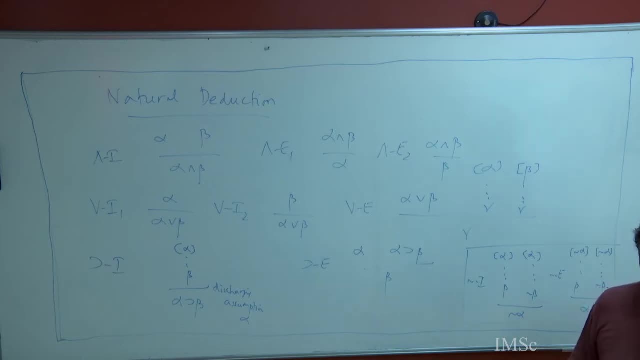 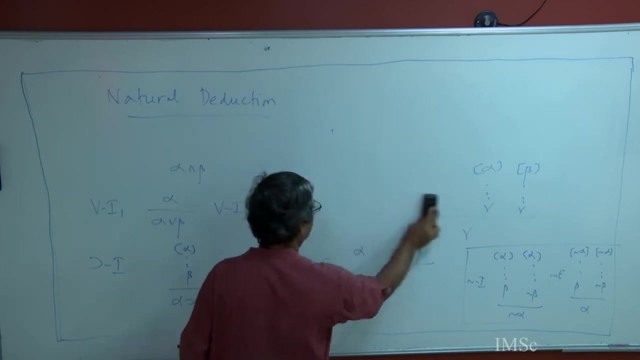 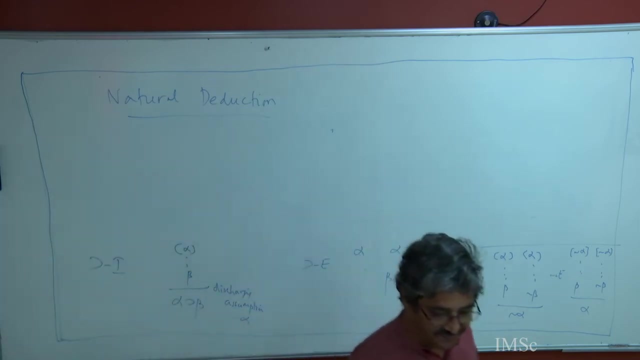 Now, what about quantifiers? So quantifiers, of course you will have for all introduction and for all elimination. there exists introduction and there exists elimination, yeah. So how do we expect this to go? Yeah, So what would be for all introduction rule? If you want, I will write the quantifier axioms. 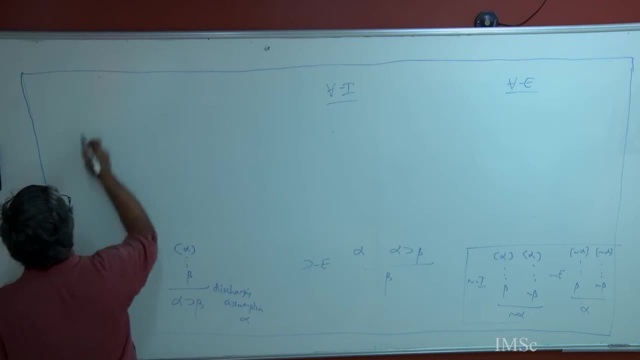 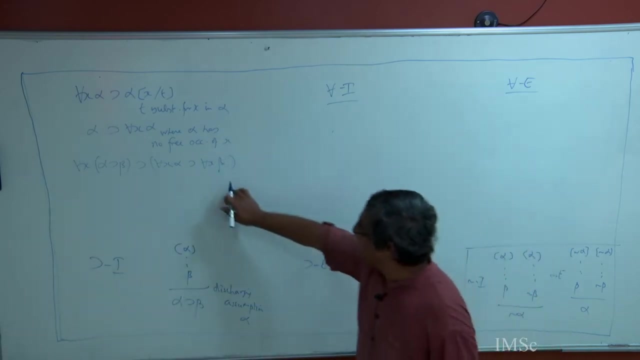 to remind you. So what were the quantifier axioms? in Hilbert style? Yes, Yeah, Yes Yeah. alpha implies for all x, alpha where alpha has. and then Now the third one is really a thing with the Hilbert system, right, because you have got a Hilbert system and your modus. 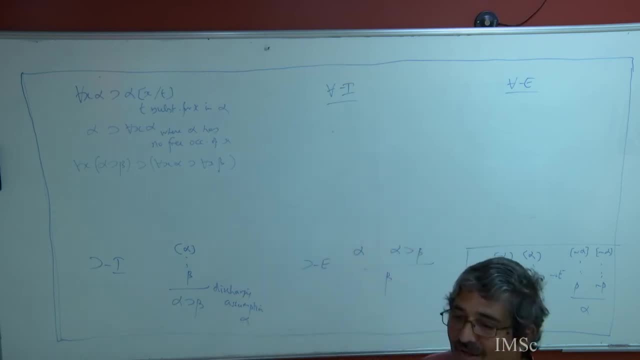 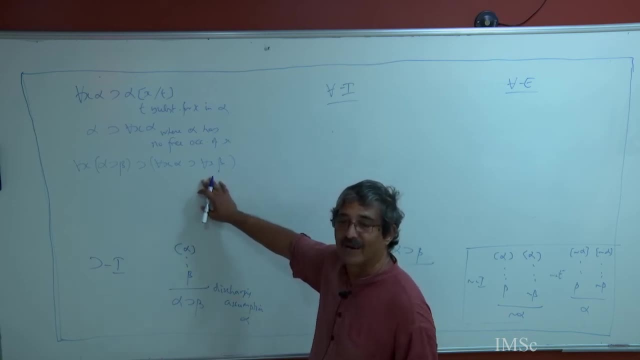 ponens is only your inference rule. you are writing it in an implicational form. you have to have some way of doing this really right. This is an instance of because you are having the Hilbert system, you are having axioms, you have to write it, Otherwise you do not. 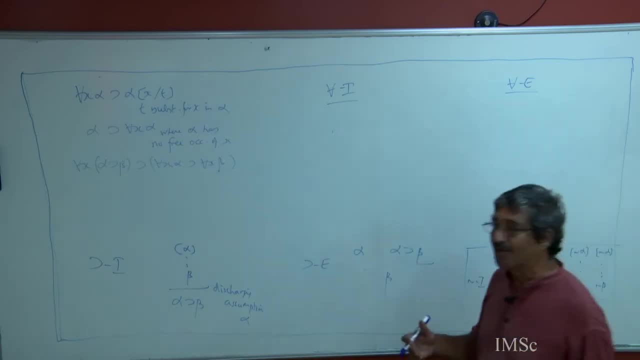 really need this when you are working with inference rules. If you remember, I also talked about having these as an inference rule right. This you could have as an inference rule right because, you remember, in proofs we always allow generalizations, right? I hope you remember. 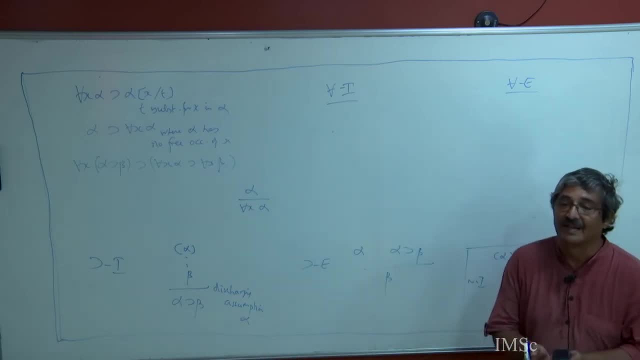 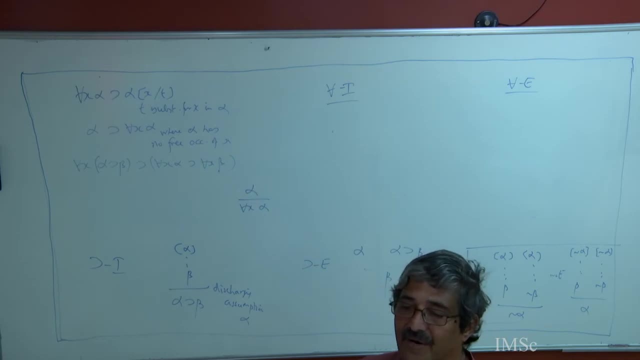 this that we talked about, that the notion of proof in a Hilbert system with quantifiers is that axioms are schemas everywhere you can substitute. take substitutional instances in proofs and you can throw in any number of universal quantifiers. right, And that is. 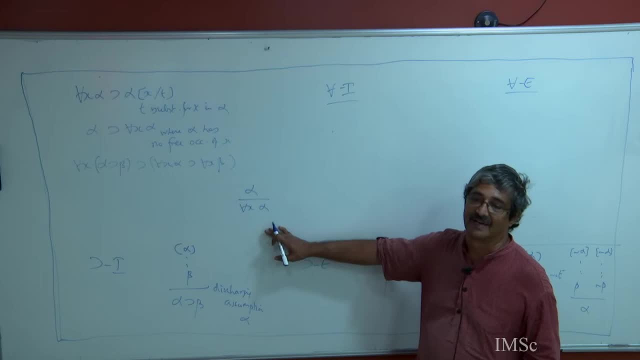 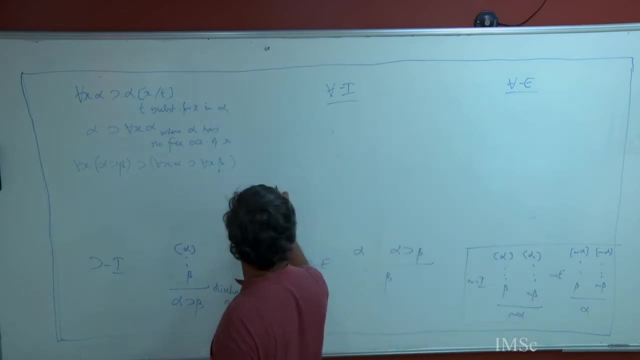 because if alpha is valid, of course, for all x, alpha is valid as well, right? I hope that is clear. Yeah, And therefore you can also have rules like this. In fact, this is a weaker rule, and it is very interesting to use this rule instead of generalization, right? And this axiom is: 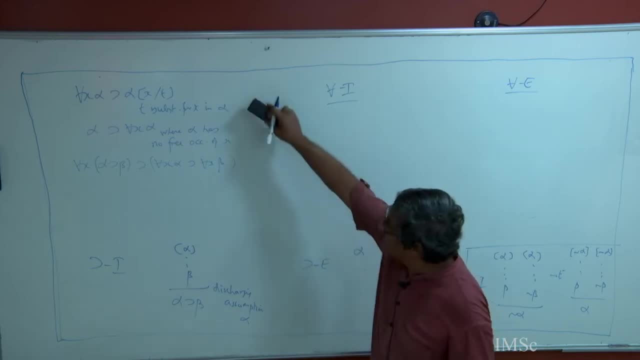 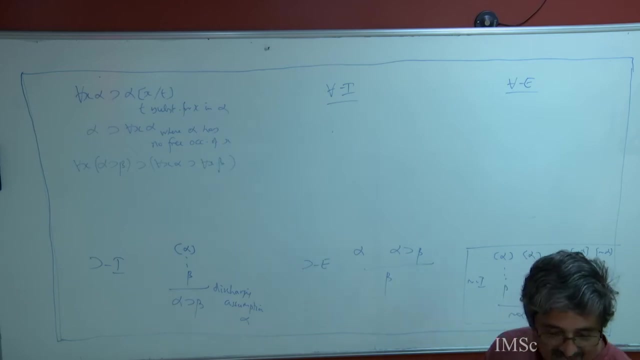 capturing precisely that, But this is where all the work is being done, and I hope you can see that this is basically a case of for all introduction and for all elimination. right, that is what is going on. Yes, So can you guess what the for all introduction and for all elimination rules would be? Can 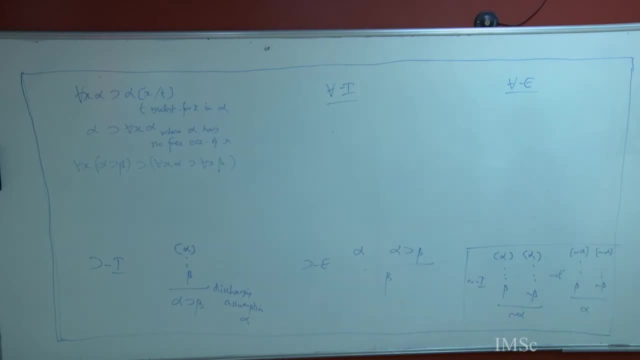 somebody tell me What would be a for all elimination rule. Well, for an elimination rule, what is the structure of an elimination rule? what should be on top and what should be below? Done, Done, Done. So let us write for all x, alpha. So what should be the thing below? 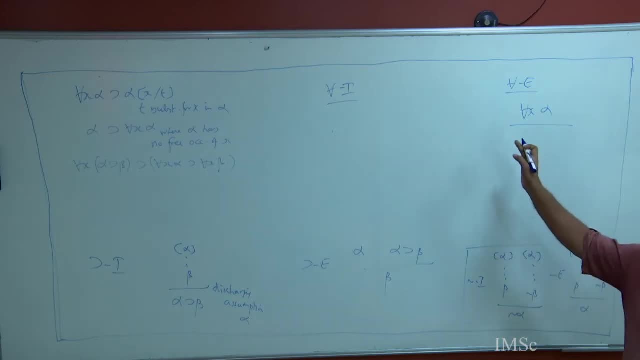 Not some variable, which particular variable We are eliminating for all x? So alpha with that is it? I mean it has to be this. That is my point. You do not have. this is the thing about natural reduction. You have to eliminate the quantifier. How do you eliminate? 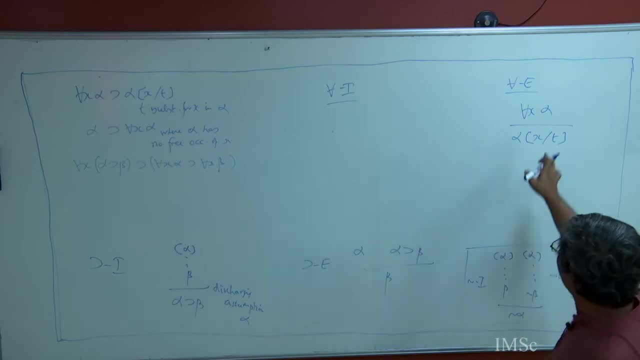 the quantifier By choosing an instance. If you have shown that for all x alpha is a valid formula- And this is the point- If it is a valid formula, then you can substitute any term for it. But what kind of terms can we substitute? We know that where T is, whatever, Yeah, If T is. 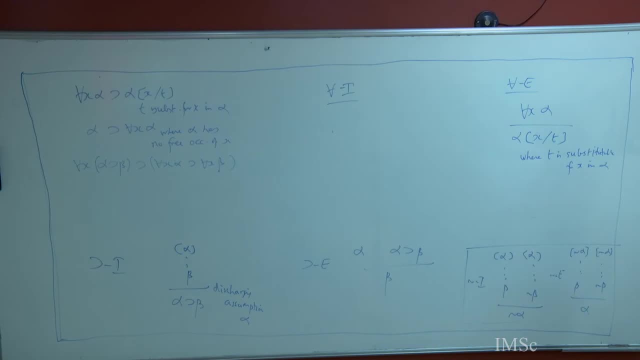 we know this business. We went through this in painful detail in semantics. Assume this is valid. suppose this is not valid. there is a particular model, right, there is a particular model which makes it false. Now, because t is substitutable for x and alpha I can transfer. 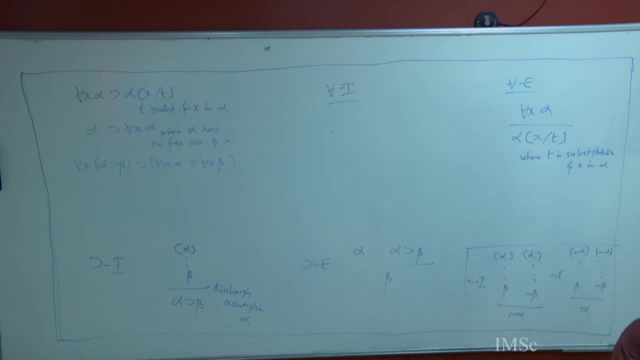 it to the left hand side. You know that in that model, consider the. in that model, look at the valuation for x with whatever pi hat of t alpha is not true in that model. But then we have been told that for all x alpha is valid right. Therefore, for all x alpha. 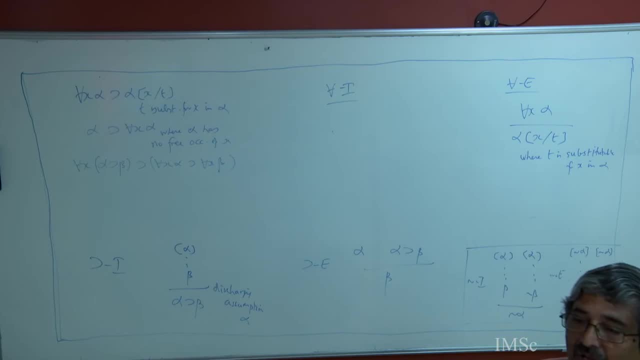 as true in that model, and that is a contradiction. yeah, So this is the for all elimination. What about for all introduction? Again, there is not much choice. How will for all x introduction look? For all x alpha should be the bottom right. 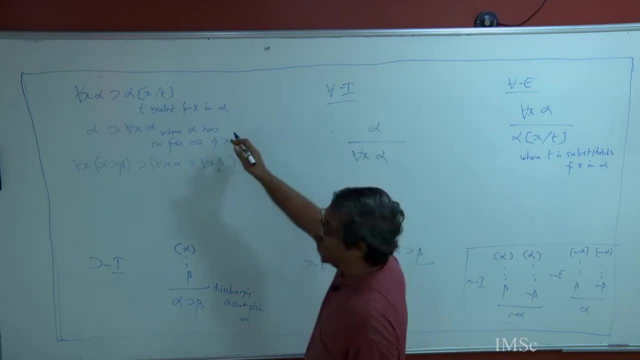 half point, But there is a condition here. So what should we have For all x? alpha should be the bottom right half point, But there is a condition here. So what should we have For all x? alpha should be the bottom. 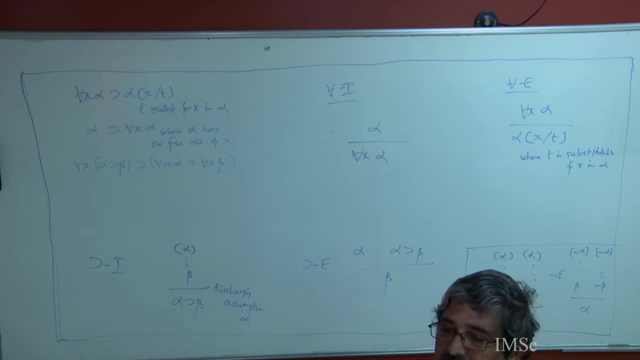 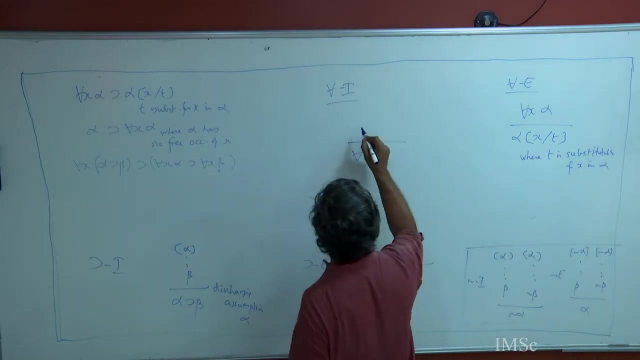 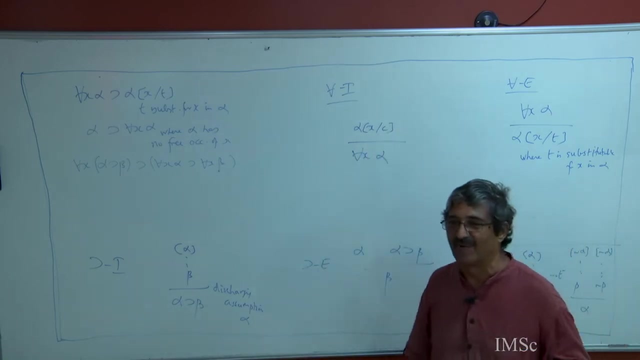 Yes, That x is not free in alpha, X should not be free in alpha. but so now, natural deduction is usually stated in a slightly different form, and you will see why. and so this is how it is. You could do with terms. let me not do it with terms is more complicated. you have to worry about other variables and 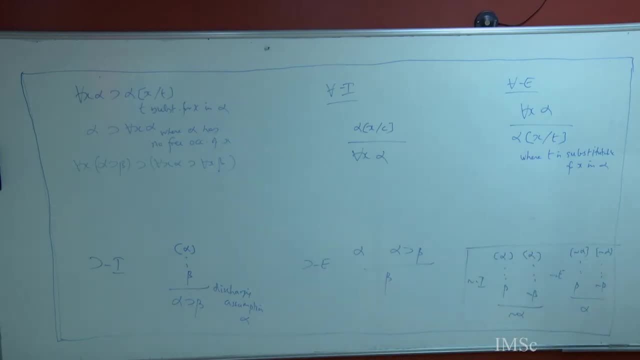 so on. but let me just choose a constant symbol, right? So let C be a constant. you have this, provided C does not occur in alpha or in any REDEFINED ALPHA. that is a side condition. This is basically our proposition of generalization from constants. 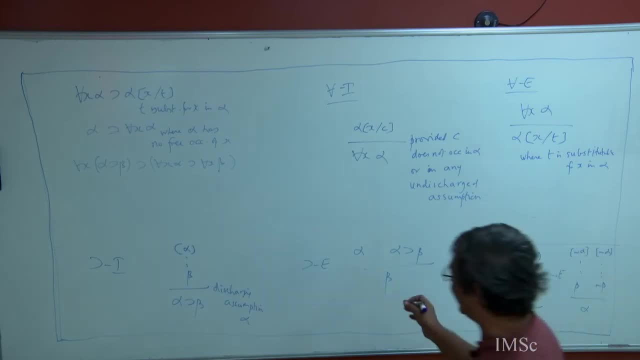 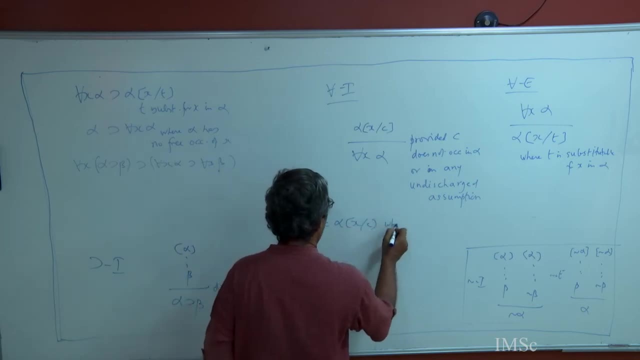 You remember what was the generalization from constants? I just went through this. If gamma where c is nu, then yeah, remember that this is the one that I have, that we got all the Paisavas soul for right This proposition and that is the form in which it is used, because 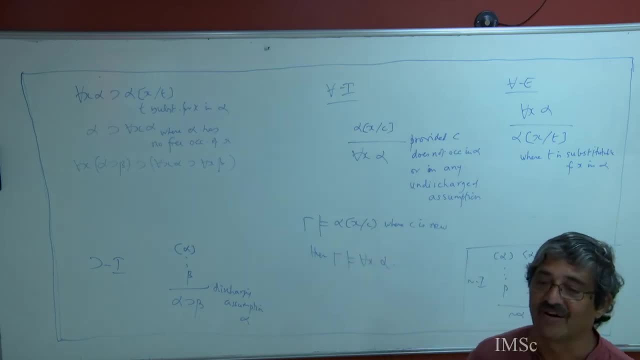 you can directly use it right, So you do not have to worry about free variables and so on. This includes the case where x is hyperbolic, So you do not have to worry about free variables and so on. This includes the case where x is. 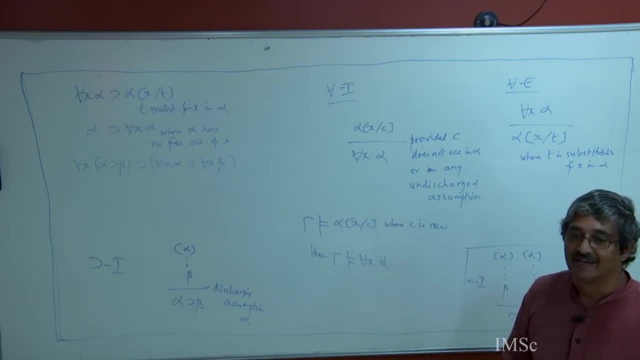 occurring free. I am not worried about it, right? yes, Shwapnil, you get the point right. You could have. this is an axiom. What is the difference between axioms and rules? This is a very important thing to understand. Axiom says it is valid. Take any model, if the model 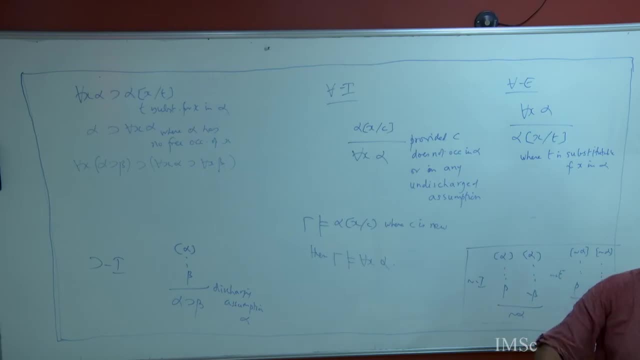 makes the left-hand side true, that particular model will make the. this is all operating within a single model. When you have inference rules, you are saying: if this is valid, if this is true in all models, this is true in all models. 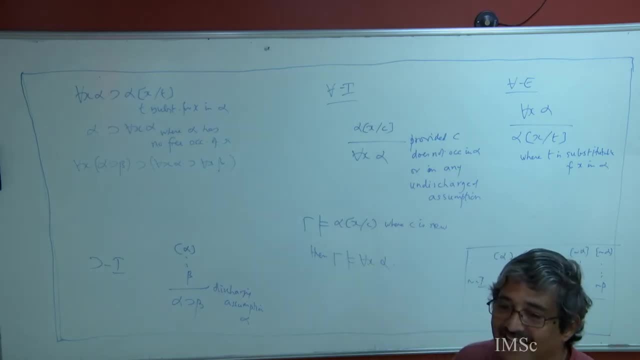 You are not relating it in a single model, right? Of course, if you can relate it in a single model, you can relate it in across models also. That is a much stronger condition. So this is the main duality from between axioms and inference rules. 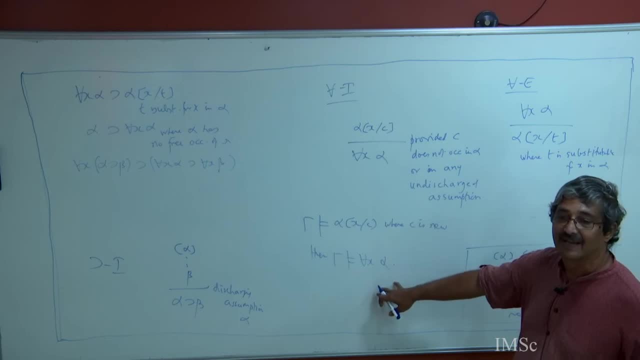 And here, since we have this proposition right. and what is this idea of this being new? This being new means it is not used in alpha anywhere And it is not used in gamma any of the assumptions. But as far as natural deduction is concerned, 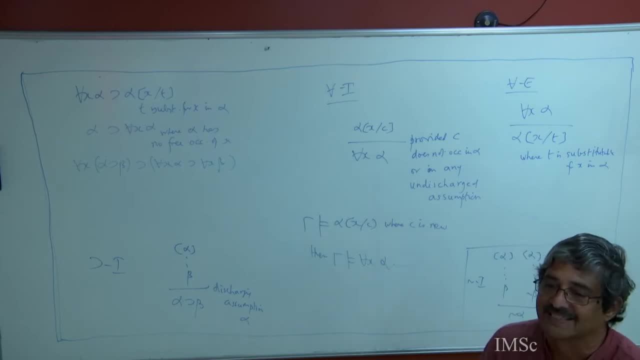 which are the assumptions that you must worry about? The undischarged assumptions? right, They are the active assumptions. Any assumption that has been discharged, you have converted it into an implication anyway, So who cares? So this is the proof, theoretic analog, of the crucial lemma. 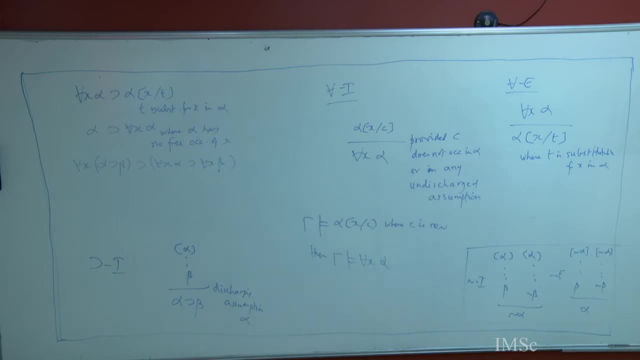 that I keep coming back to right: Generalization from constants or in the form that I stated last time, which is generalization from new variables, Right, New syntactic elements, right, And that is the spirit of the universal quantifier. 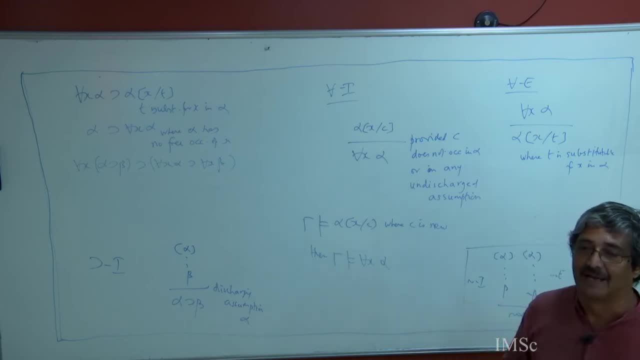 And once you understand that, you can do proofs very, very well, And usually this is what is not well understood. So many authors for symmetry would write with C. Then you do not have to worry about T being substitutable for X in alpha, and so on. 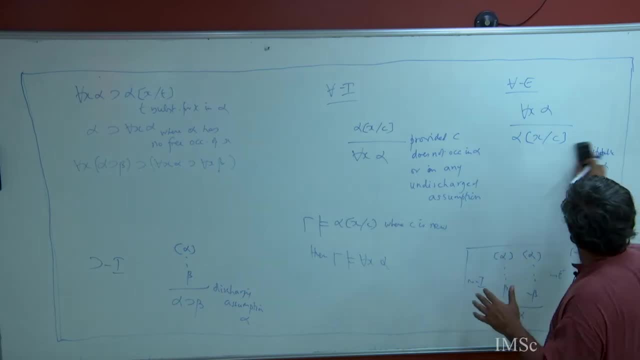 Remember, a constant is always substitutable, right? So you do not have to write it, So they will just write this, Okay? So this is typically the proof. This is typically the form in which a natural reduction is stated. okay. 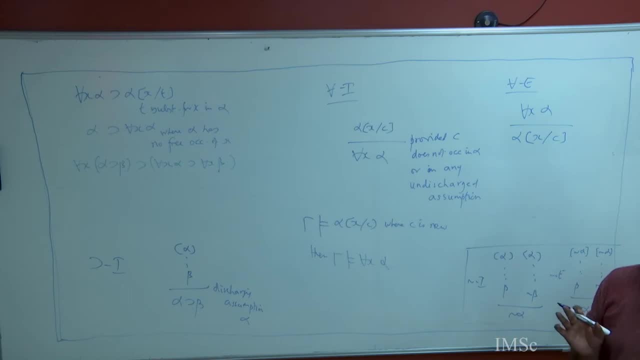 Is it clear? Ananya? Yes, Yeah, Okay, No problem, Yeah, So now, if this is clear, let us look at what will be the rules for existential quantifier. There exists introduction. There exists introduction. There exists introduction. 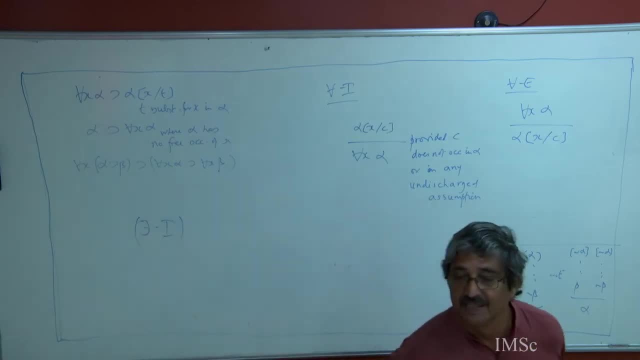 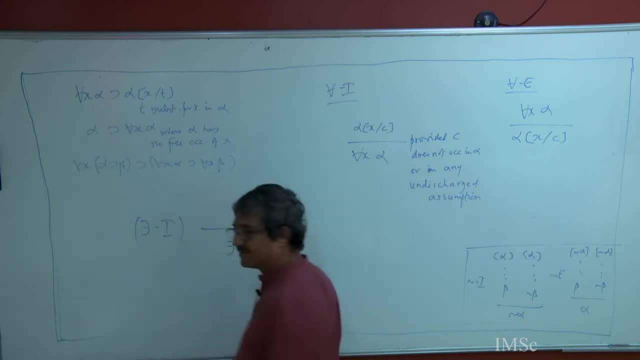 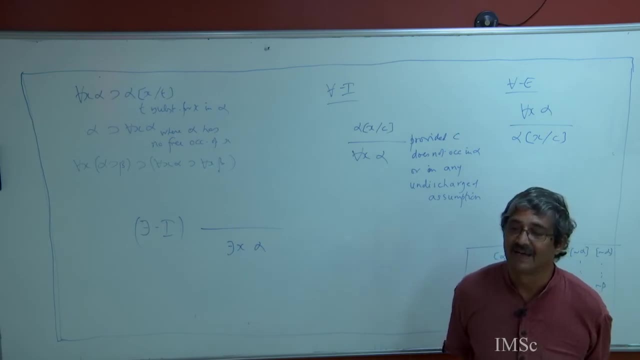 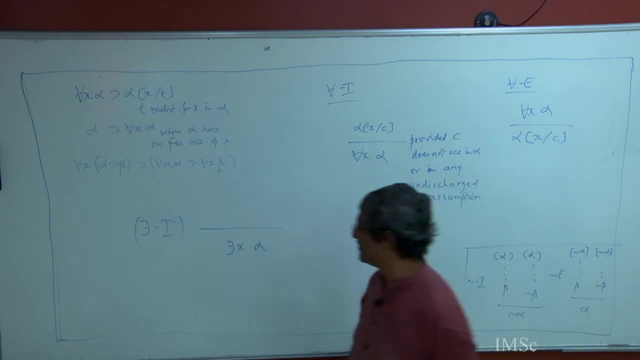 I want to conclude: there exists X alpha. There exists alpha. There exists alpha. When can I conclude there exists x alpha? Yeah, That is it Here. there is no condition, nothing. If you have shown alpha with x replaced by some element, some constant. 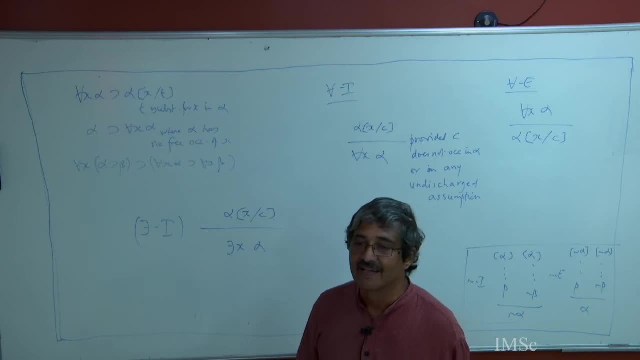 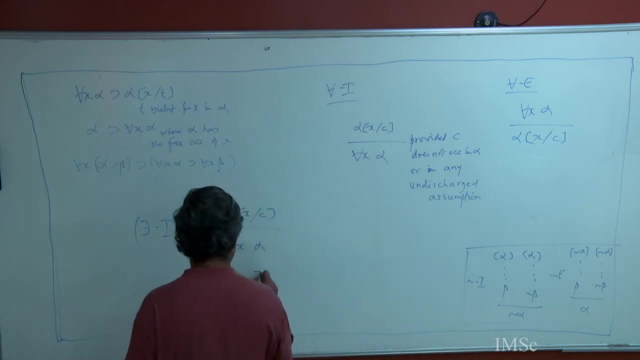 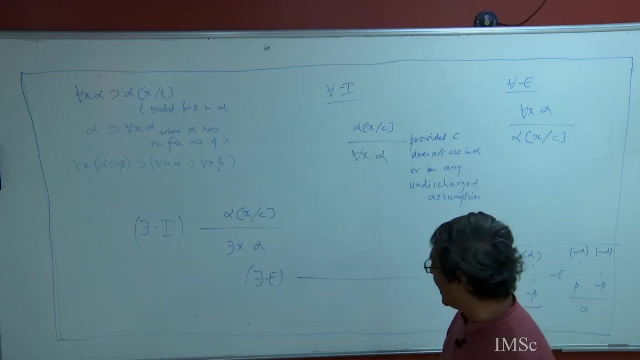 then surely you can write that x is x alpha, Right? Is it clear Right Now? what about there exists elimination? How do you eliminate an existential quantifier? You have got there exists x alpha above the line. How do you expect to get rid of it? 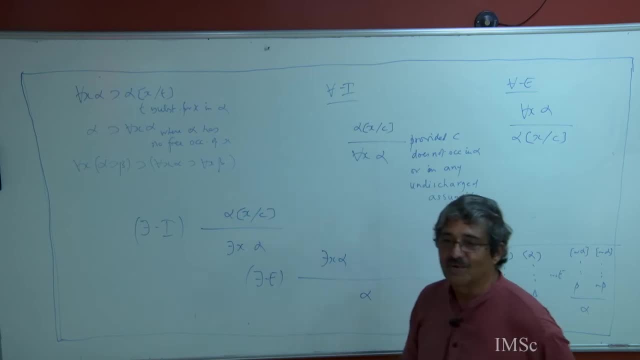 I want alpha below Right. Right, This sounds like a fairly impossible thing, Right? I mean from a universal quantifier, you can specialize, No problem. But from an existential quantifier, how can we? Well, that is true, You can do it. in that case, 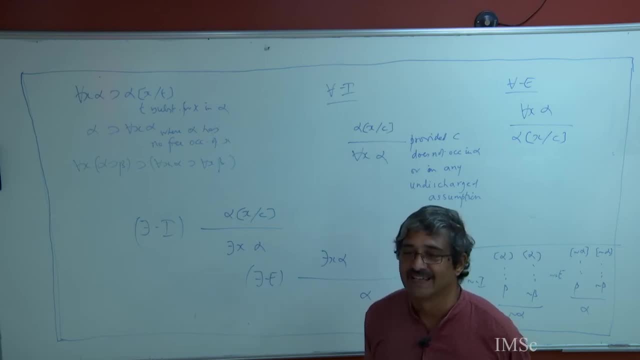 But it is pretty useless. No, In that case I have some other rules. For example, if I write some there exists x, p, x, Gayathri, Okay, Suppose I write some there exists x, p, x, And then I want to go get rid of the existential quantifier. 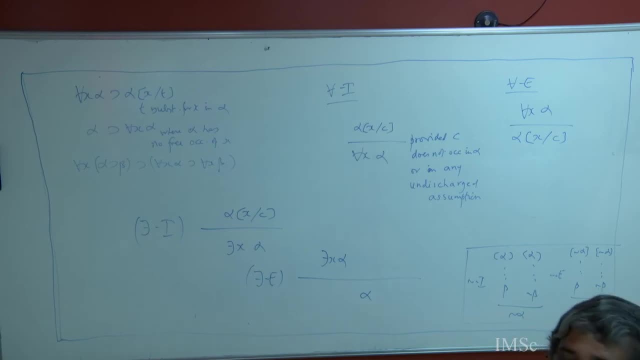 You are not helping me. Okay, Remember semantically what is the relation between conjunction and the universal quantifier. You can think of the universal quantifier as a kind of a giant conjunction, But what is the relation? What is the relation between conjunction and the universal quantifier? 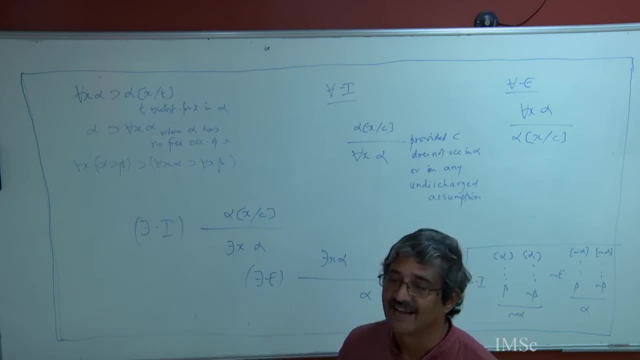 That is an un-unless. you want that. Right, That is the un-unless. you want that? Okay, conjunction, right. if only you had names for all the terms. right, if you are allowed infinitely conjunctions. right for all. X is actually conjunction over. 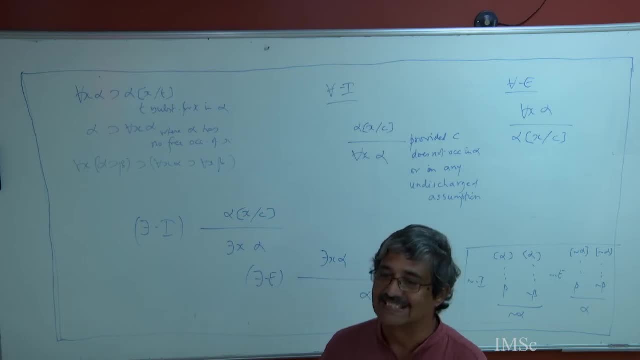 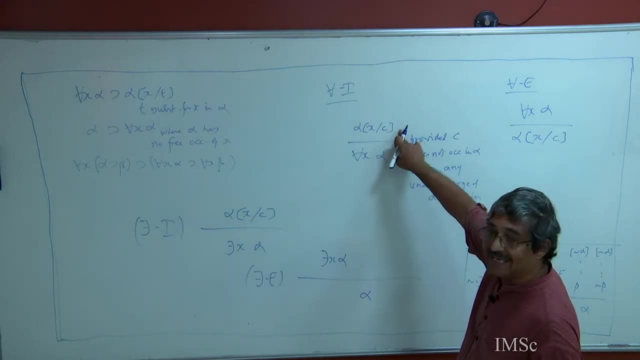 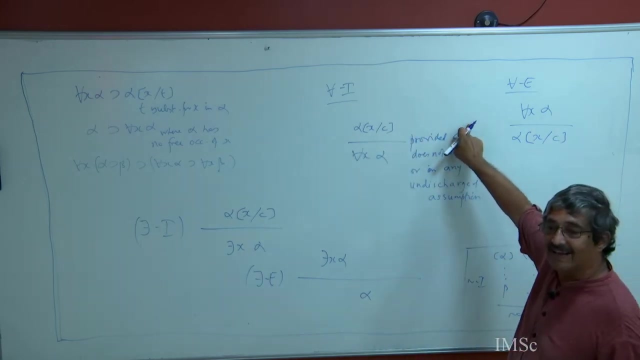 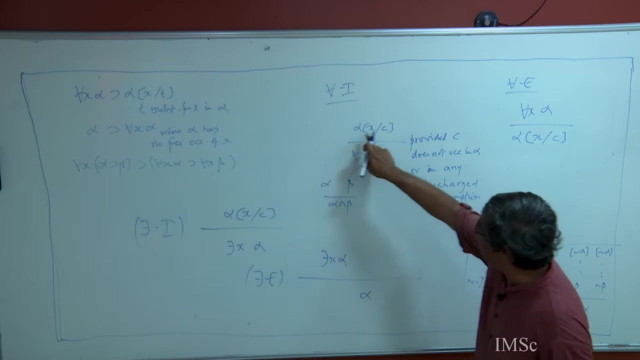 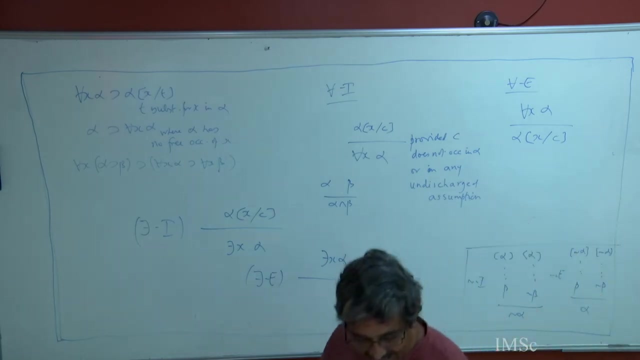 all possible X. there exists X. is this junction over all possible X? right, so for all. introduction is like conjunction introduction if you think of this as whole lot of premises, right, what is? and introduction: alpha, beta, alpha and beta. so this one actually stands for lots of premises and similarly and elimination. 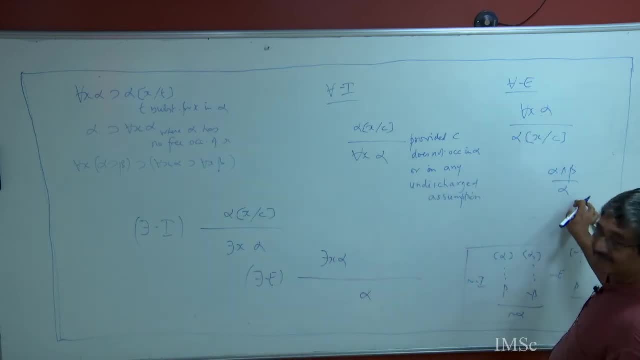 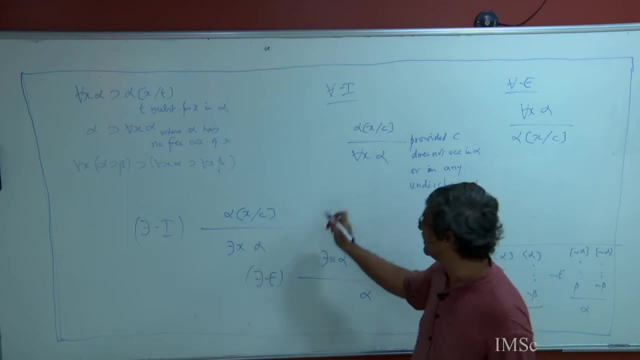 looks like this for one of them. right, if you take the analog of that, this is disjunction introduction. disjunction introduction looks like this: what should be disjunction elimination. then remember, disjunction elimination has a special place in natural reduction. it's case analysis, right alpha or beta, if you have. 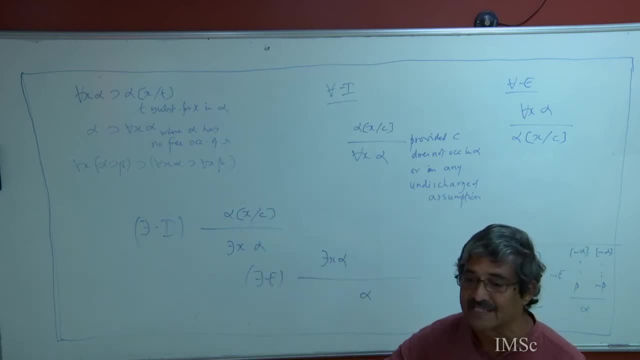 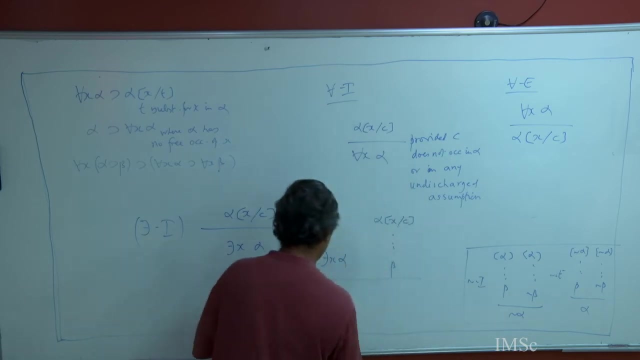 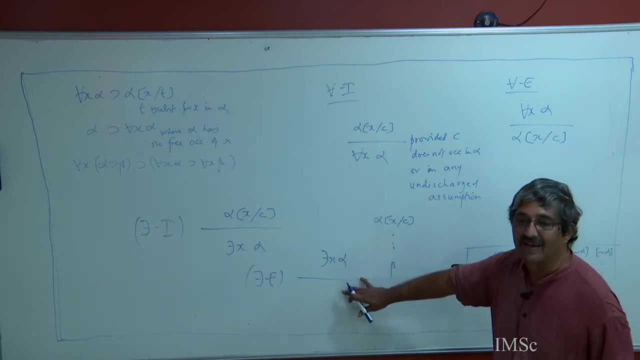 derived alpha or beta from the assumption alpha, you get something. from the assumption beta, you get something. then you can derive that conclusion beta. so what does this suggest? for there exists elimination, going to look like disjunction elimination, right? so, and this is how you do it, if I have derived, there exists X, alpha, and by substituting some X, some C. 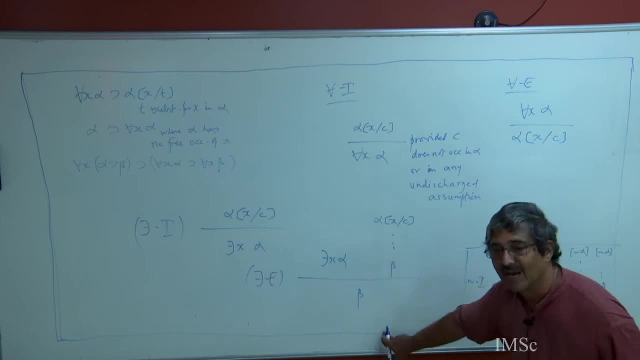 for X and alpha. I have managed to derive beta. then I am allowed to derive beta. right, take us few seconds and digest this. I hope this is clear now. where should I? what is this? there is a side condition here. what is the side condition all that nonsense about? 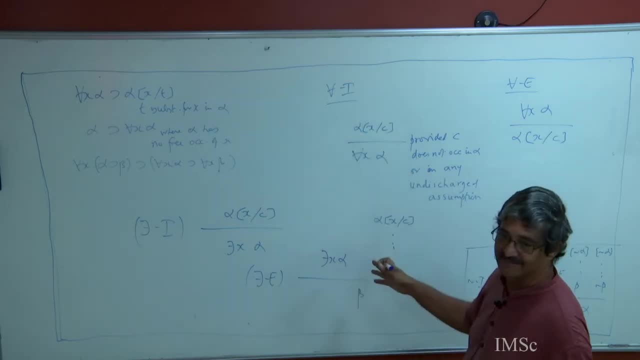 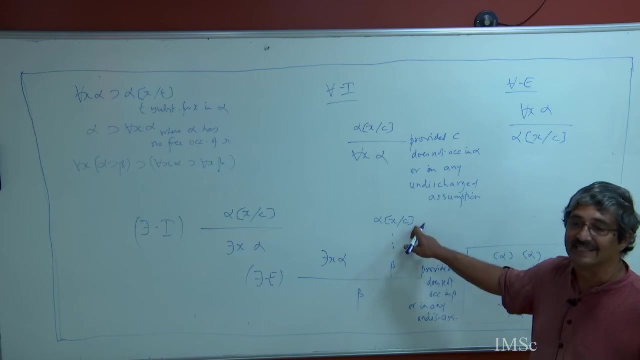 whatever I had for all introduction, it has to appear in there exists elimination, obviously right, where provided C does not occur in beta or beta. Okay, Okay, Okay, Okay, Okay, Okay, okay. So there you have the bottom end of the again of this, the very basic. 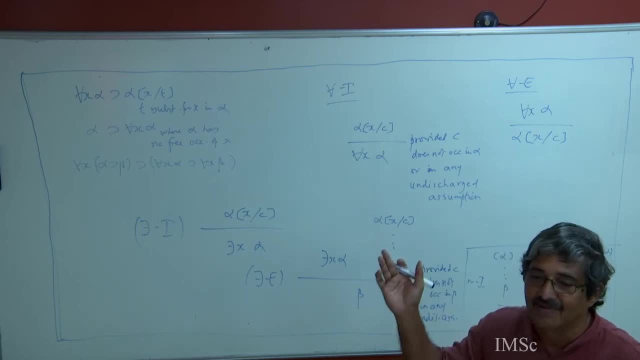 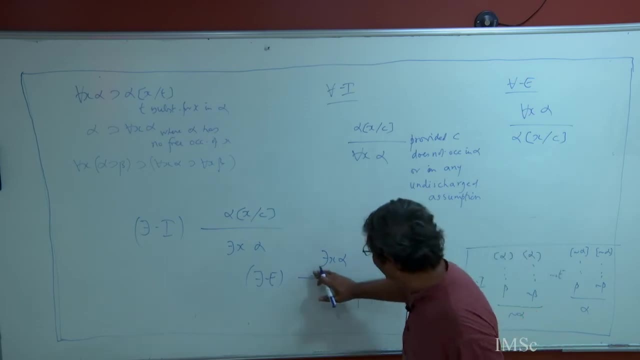 rajohn right set the basis and then other points of the commotion and then over to the lower part of the table. Okay is arbitrary. therefore it suffices. the assumption that there exists x was enough to derive beta. This is what you are saying, right? the assumption of some witness for x for alpha is enough. 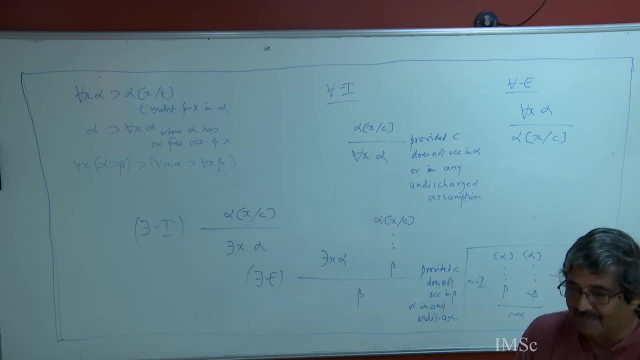 to derive beta right. That means: let k be a witness, let c be a witness for alpha. from that I conclude beta. but the choice of c was arbitrary, therefore beta. This is how you write it in mathematical texts, and this is very important. in mathematical texts you: 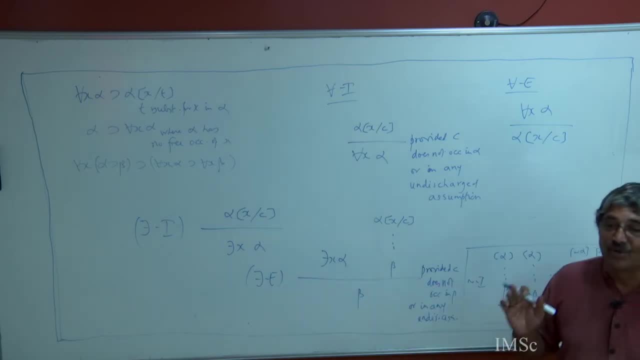 use this arbitrary business in two ways. right, When you want to write something, you want to prove something general, right? You say: consider the statement, take some arbitrary element of whatever structure that I have got. I do the entire proof and you say: but the choice of that element was arbitrary. therefore, 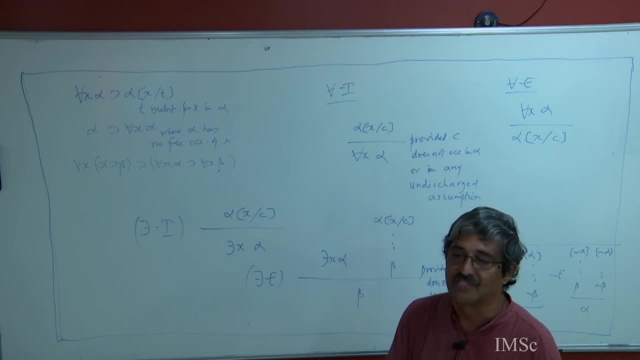 it holds for all elements. This is one universal form in which you use, but you also use the existential form right. Suppose this is true for some element right? Well, consider a particular element c. I do the entire work and I conclude beta and say: but I did not use any property. 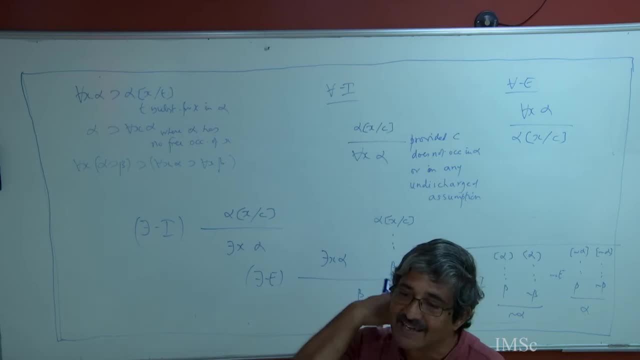 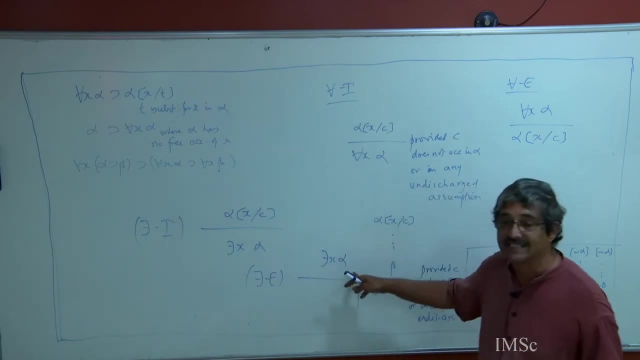 of the element, right? Haven't you seen proofs of this kind? and you say there is no distinguished character of this particular element? therefore, the assumption that there existed one was enough for me to conclude The existence of the such an element is all that I used for concluding beta. So, ok, you. 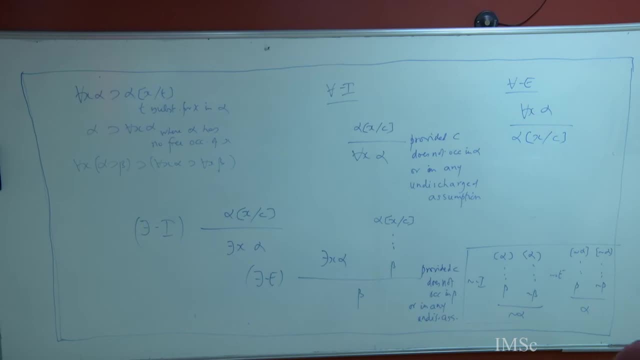 just anyway, this is all in words. you can check that. this is sound, right? That means, if gamma, if this is a consequence of gamma and this is a proof, then this is a consequence as well, right, and that is something that you can actually sit and do: the proof of. 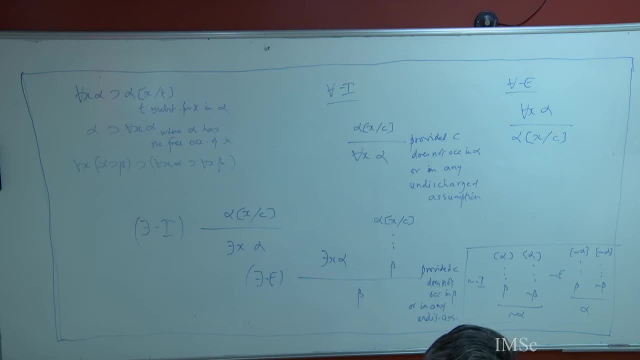 Sorry, I did not understand. Sujatha. there is some comment, So I just wanted to make this comment that if it is alpha bracket, square bracket x by c per bracket, there should be a bracket outside. it is not it because it is an assumption. 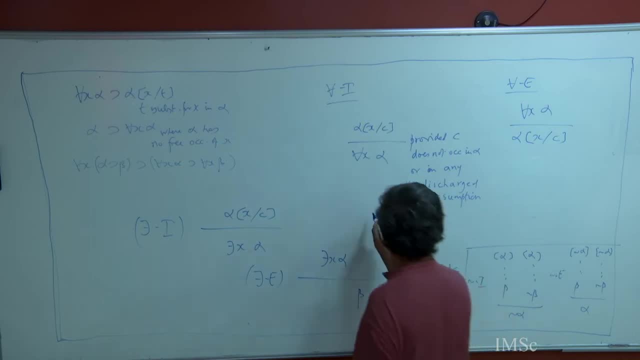 or I might. Oh, you are saying that this: There is a bracket outside. This is the assumption. Okay, I think it is the assumption. Is this wrong? Is this This? Yeah, is that what you said? Yeah, sure, This is an assumption, exactly like I have written all these. Yeah, thanks. 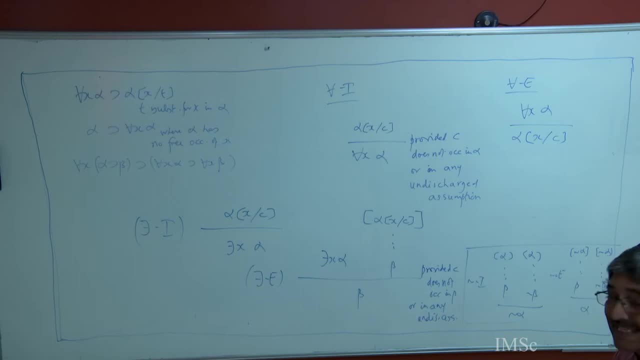 Is this an assumption discharged? See, the thing is, the question that you are asking really is: when I apply this rule, am I discharging this assumption right? Actually, you do not need to. You do not need to discharge the assumption Because, as it happens, this is the one that 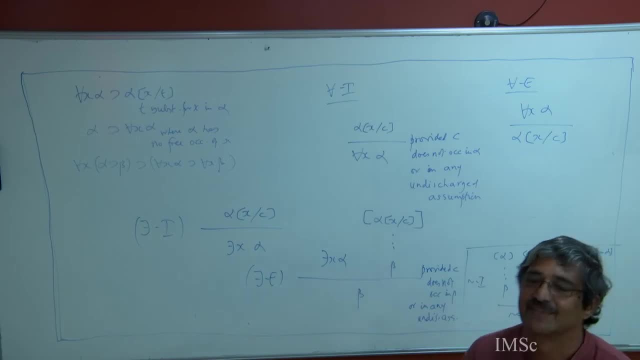 you are discharging right, But it is not an assumption in the natural deduction sense. None of these are assumptions in this sense. These are assumptions, So you do not need to put this in. okay, Yeah, Anything else? Okay, I have got some examples And well, these are all proofs. As usual, there will be some. 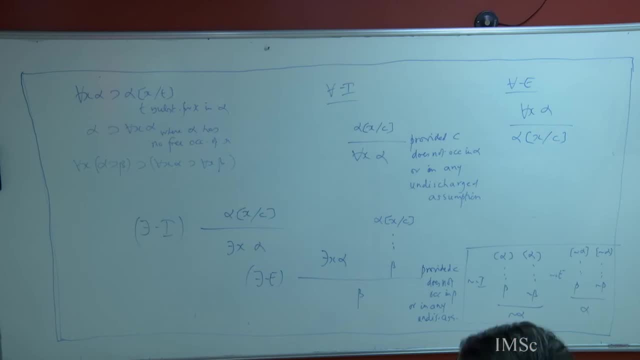 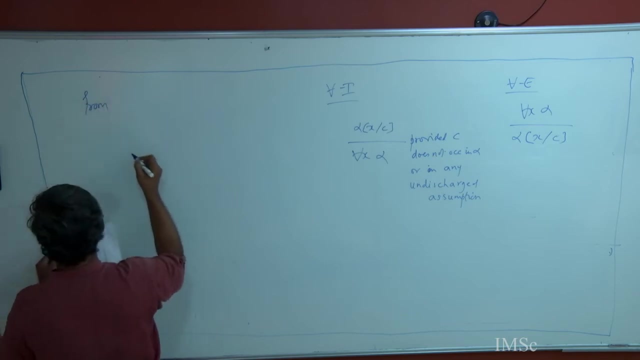 Okay, Here is something for the universal quantifier. Any question about the rule? So can I get rid of them? Okay, Let me keep the universal. Okay, So here is the. what we want to do is something fairly obvious from for all x. 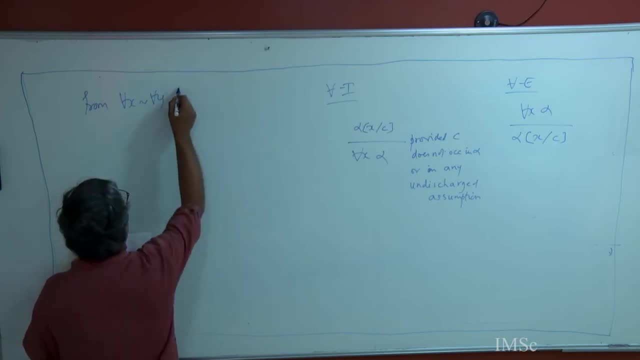 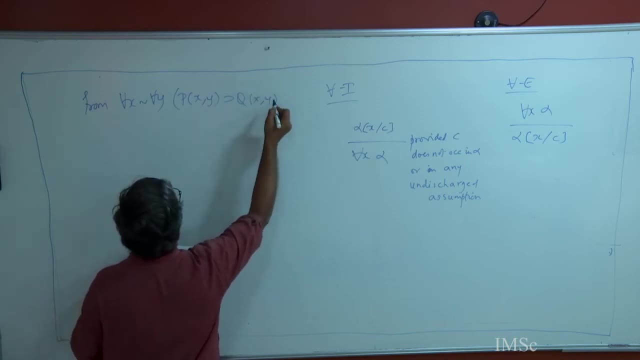 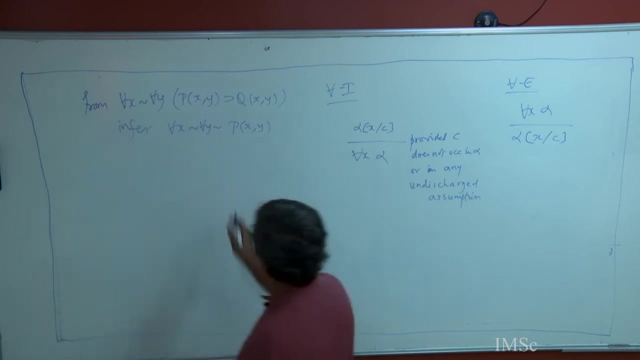 x, not for all y. p x, y implies q, x, y. We want to infer for all x. I mean, of course it is, there exists y, but in whatever form you are given, you have to derive, right, So okay. So what is it that we want to derive? 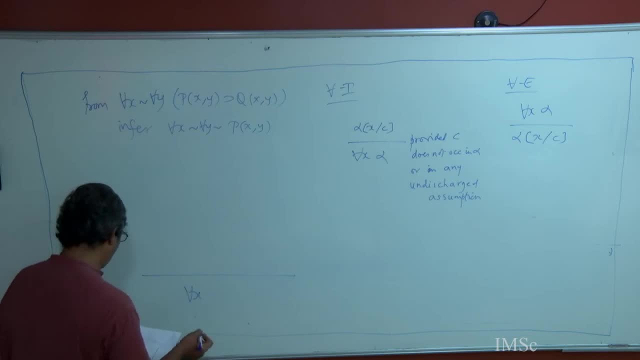 Remember, in natural deduction you always start or sequent calculus. you always start from the bottom. So this is a goal right, And you have got a for all x here. So the only rule that you will apply is: 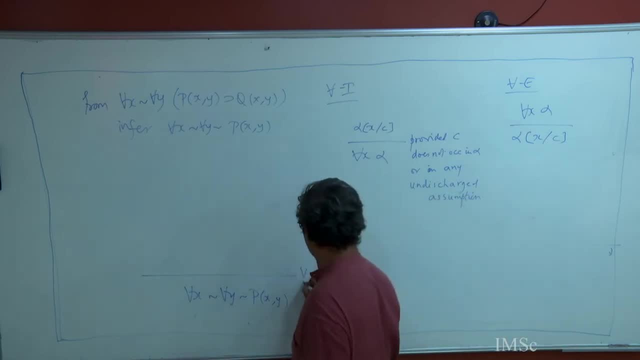 the only way you could get to this is by a for all introduction rule. Yeah, I mean, this is how this goes right. Okay, Because I want to derive this, and the primary connective that we are looking at is the universal quantifier. 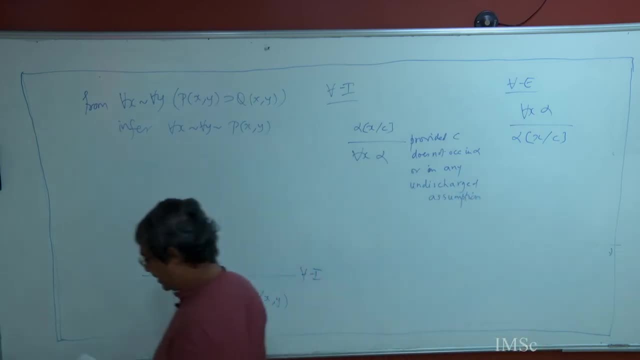 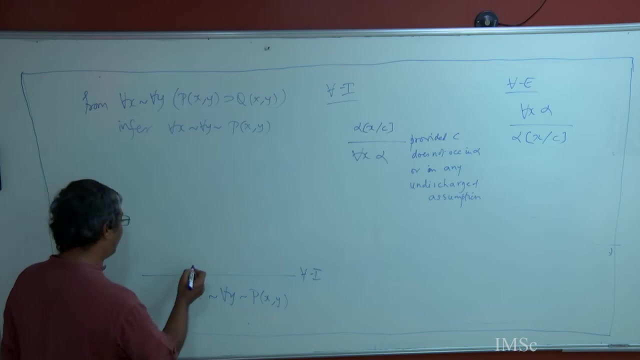 and that is below the line. So I have to use a for all introduction rule. So now, so I must come from some instance of this, So let me write p, a, y, Okay And okay, And this is what I have to do. 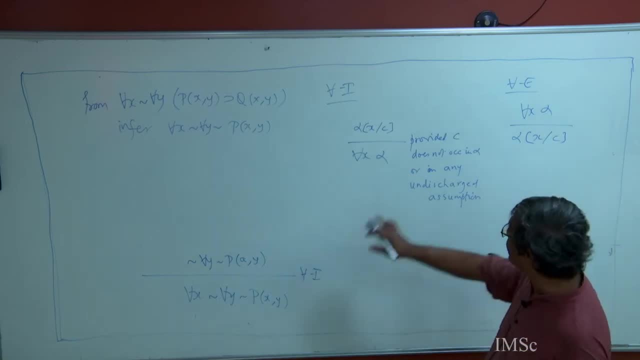 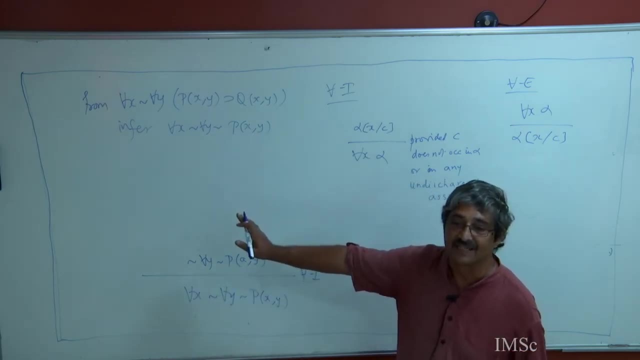 So I will have to make sure as I go up that this a is something. a is not occurring here below, and I will have to make sure that it is not occurring anywhere in any undischarged assumption. right, This is what it is about. 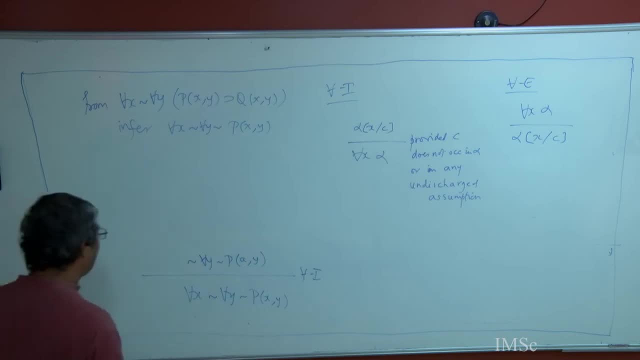 Now this is of the negation form, So I need to use negation introduction, right. So that means from some I want to get a contradiction, and the contradiction I am going to use is this: It is since it: 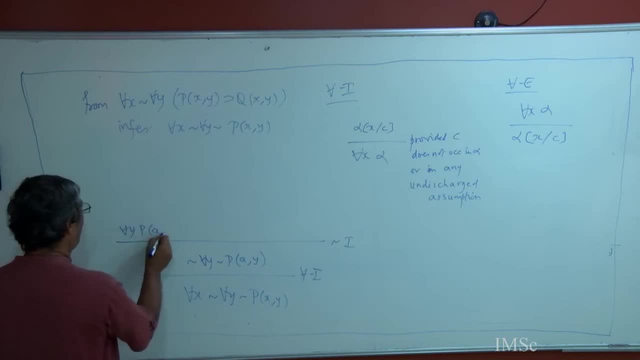 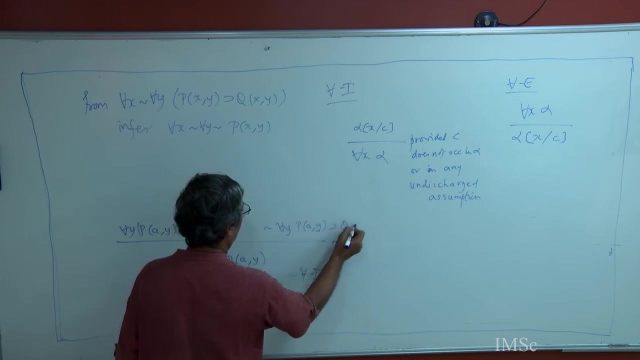 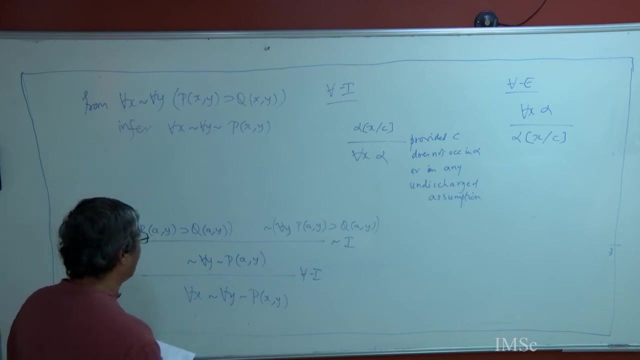 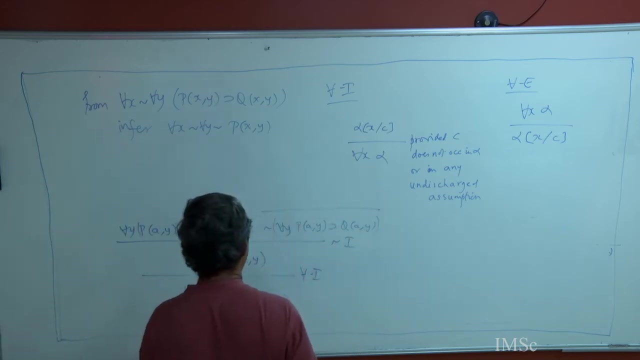 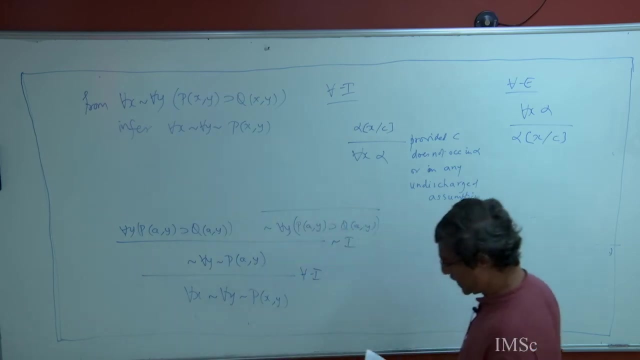 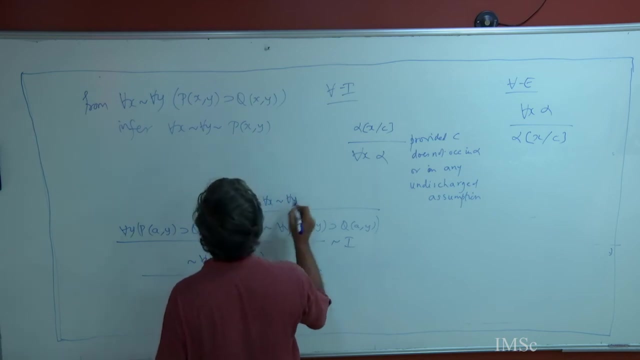 is sitting here for all y, P A y implies Q A, y, and I will have not for all y, and then by negation introduction I can come here Now, here, So. So here I am directly given, so I can, yeah, So. 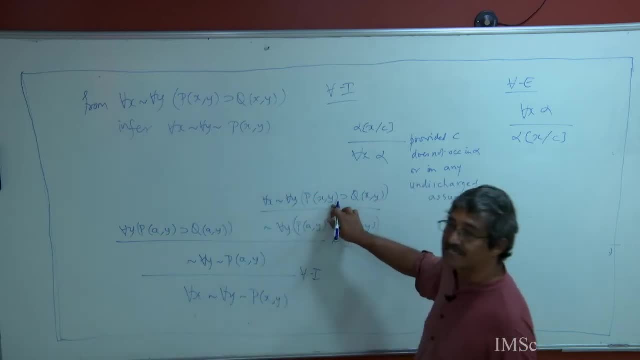 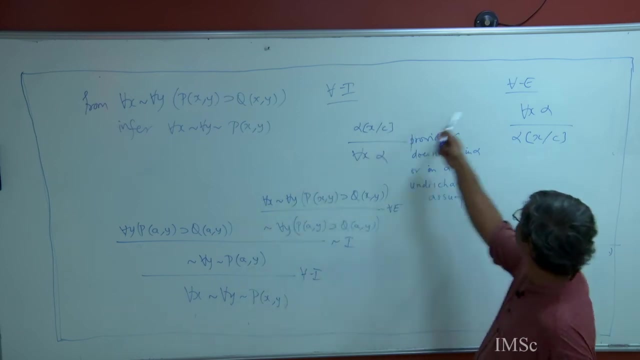 So here I am directly given, so I can. yeah, This is an assumption, and now I can use for all elimination, yeah, to get this. Is this step clear? This is directly given. I know that for all x alpha is here. Therefore I 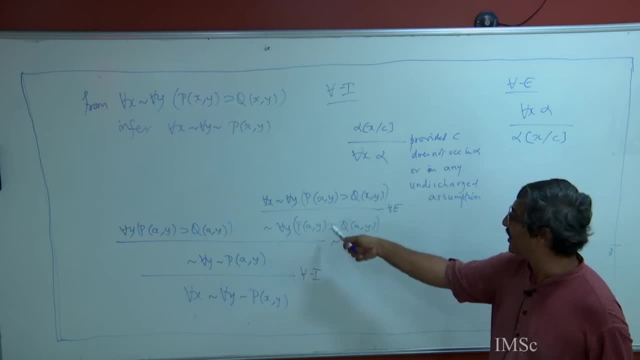 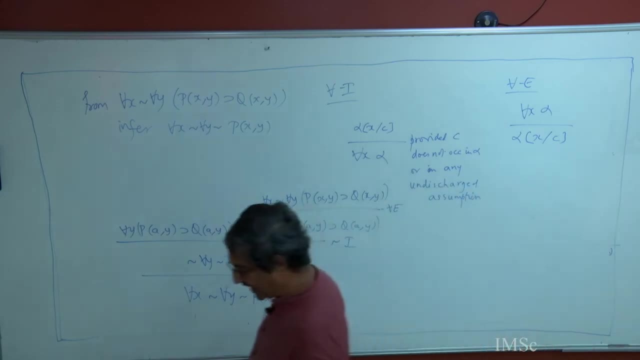 can always substitute some element for it. If I substitute x by A, I get this. So this part is easy. What about this one? I have to somehow get this. Yeah, What about this one? Yeah, I have to somehow get this. ok, So this has to be a for all introduction rule, because 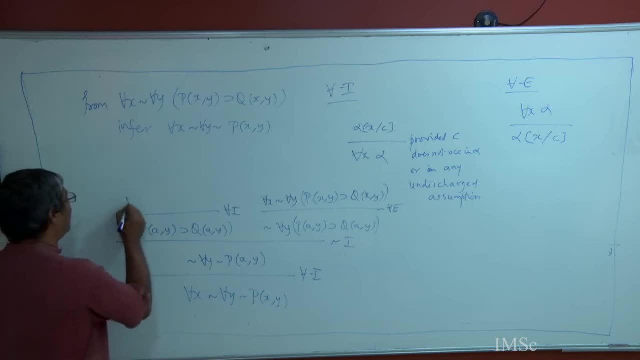 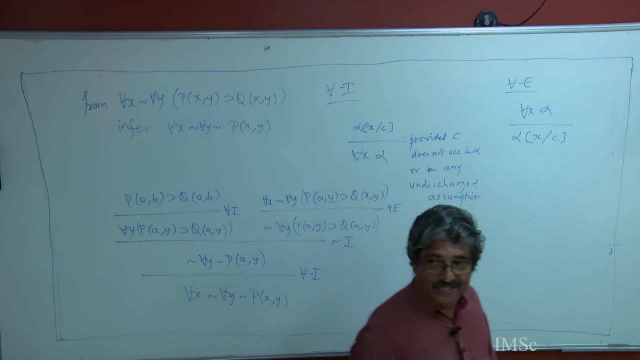 there is a for all setting here, So I will throw in a P A B implies Q A B, some substitution. Once again, as I move up, I have to make sure that. remember that B is not occurring anywhere below, So that is clear. 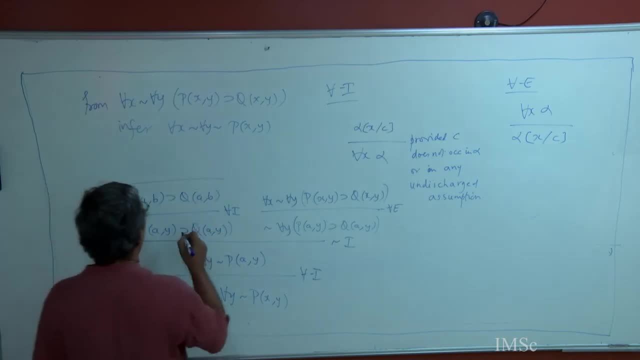 And now I can use a. yeah, I will do an implication introduction. I will. so P A B has to move up. This is the problem with natural deduction. I never know how to plan this. yeah, So somewhere I will make an assumption: P A, B, And from that I. 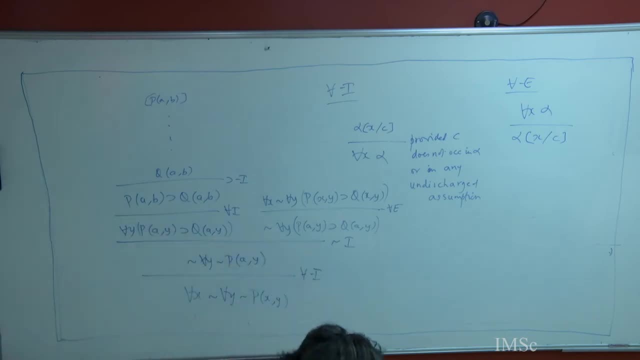 have to get Q A B. yeah, Ok, So from P AB. so, except that I am going to do it in a, what I will do, I will get a, not P AB, for which I can do an assumption for all y, not P A, y, from which I can get Q AB. 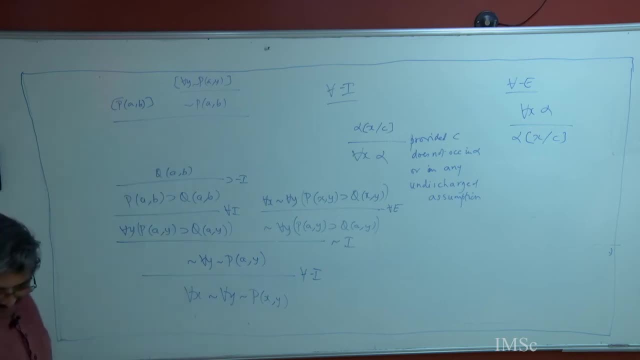 Yeah, oh, I did not have to climb so much, sorry about that. I can bring it down right, yeah. What is very nice is now I have discharged both the assumptions here. yeah, So P, AB is discharged as well. as for all y, not P. 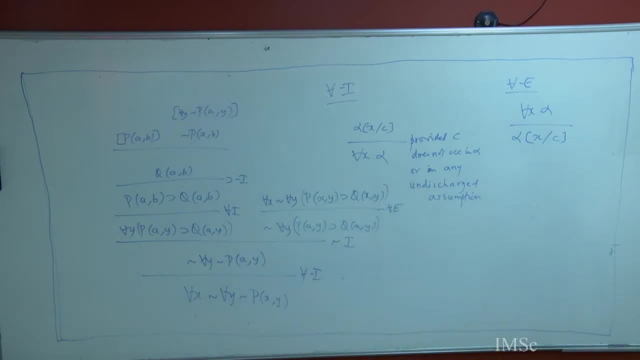 A. Yeah, A y is discharged And there is no. so there is no discharged assumption, undischarged assumption that is using A here. So this is important, So A can be used. yeah, So, for all elimination- and this is a negation elimination. yeah, So, yeah, so, as I am doing. 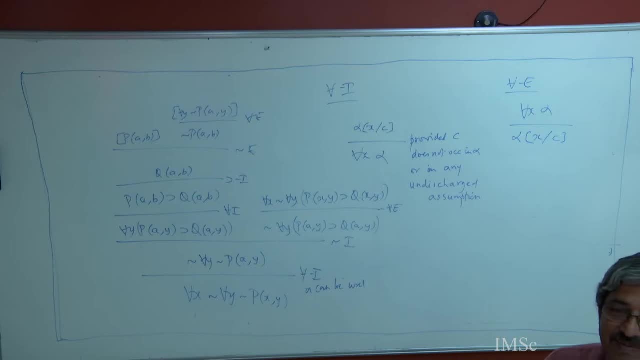 this to show that you have to- of course, I did not do it precisely the way I showed you right. Some part of it you do this way. some part of it, you guess, from top. ensure that it all meets up and make sure that your proofs. 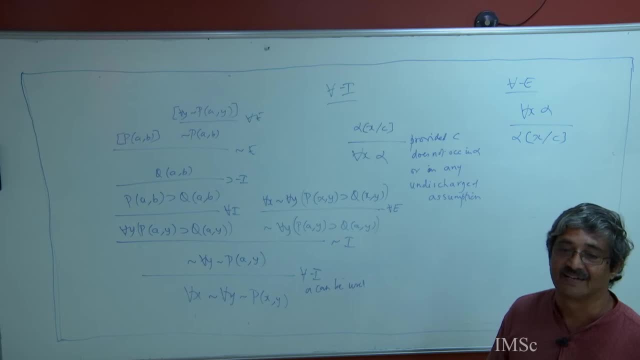 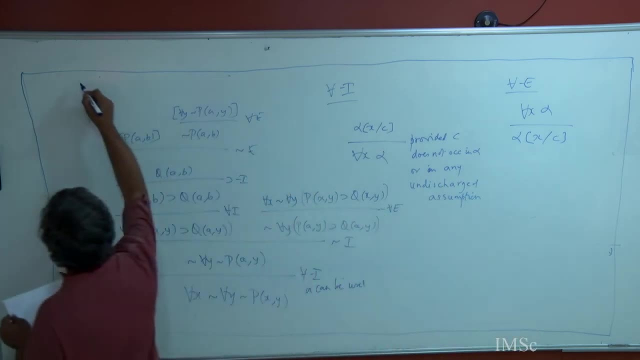 Yes, The side conditions are met carefully. right, This is what you have to do and you have to plan it out a little bit. And the plan, really, as I said, you look at the form in which it is given. right, Given is for all x, not for all y. P. xy implies Q, xy And to prove is for. 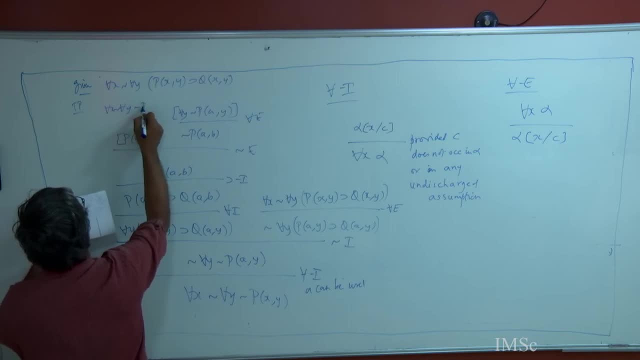 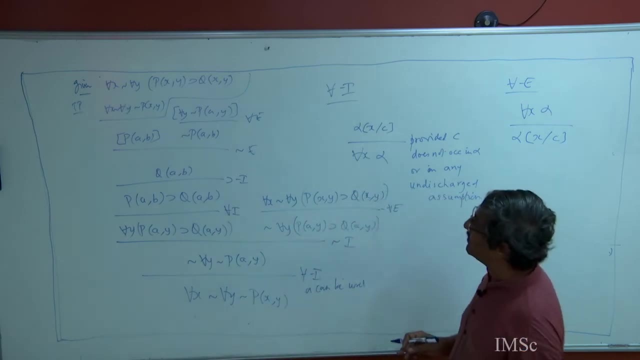 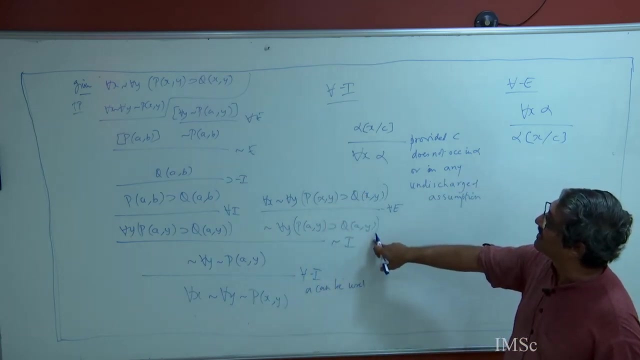 all x, not for all y, not for all y Right. So, as I said, the one part you can try to get directly by applying which from the assumption directly you can get, And then you realize that somehow you were to get to not for all. 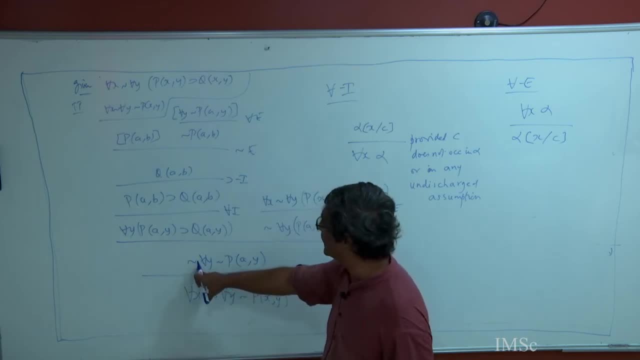 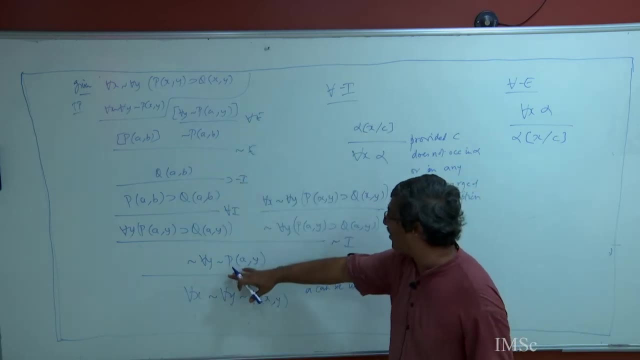 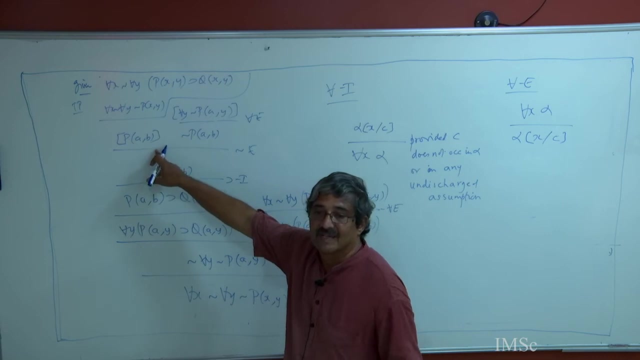 y not right, So introduce a negation. I have to somehow get a contradiction from for all y not. Yes, Not P a y right, And you have to make an assumption. When you have to make an assumption for it, you might as well assume P a, b or for any particular constant as well and get rid. 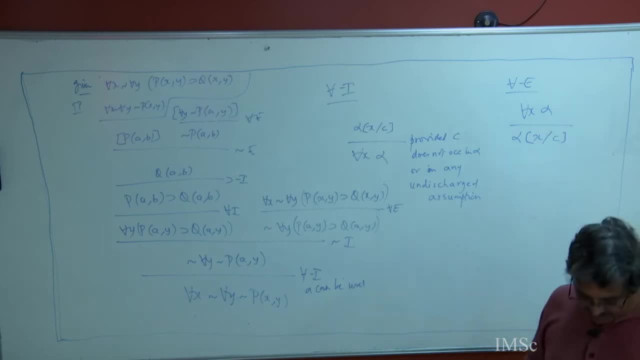 of it as you go down. yeah, So, yeah, at least is this proof clear How it works. Any question related to that? Yes, So remember that P a, b is discharged here and this is discharged here. yeah, And so. 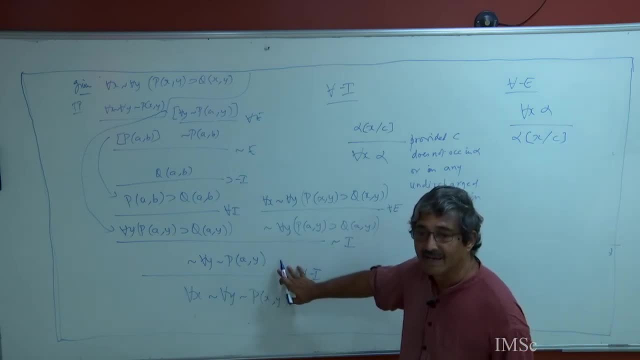 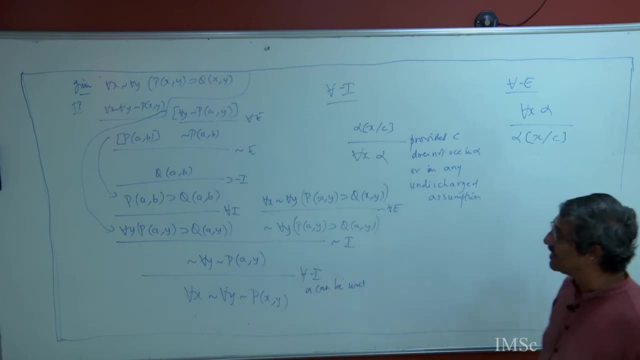 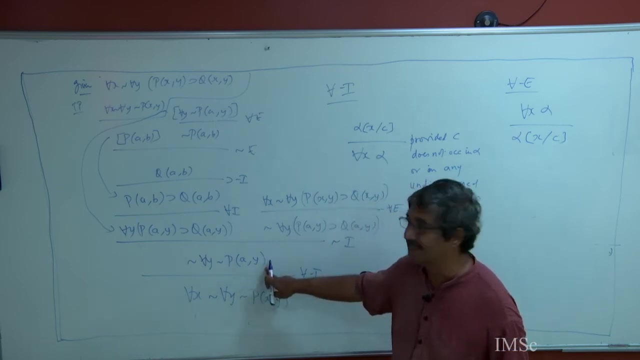 that is important because when you are here you have to make sure that you know. when I do a for all introduction, I have to make sure that the element that I am using is not A, is not there in the conclusion and not in any undischarged assumption. So by the time, 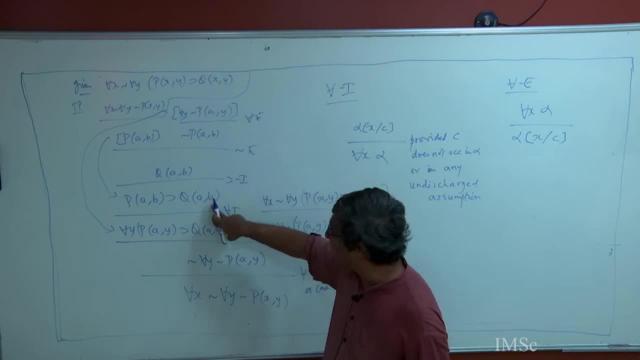 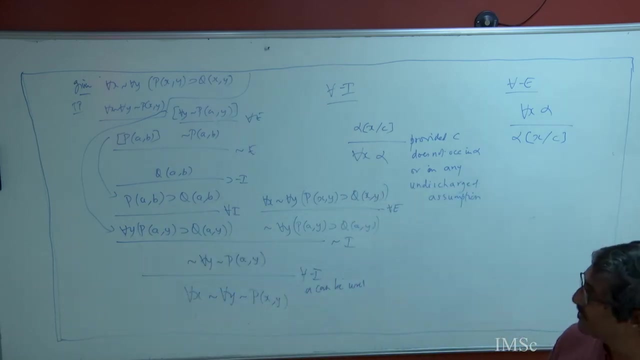 when I am here, for instance, here, I have to make sure that B is a constant that is not used below and that is not there in any undischarged assumption. And there is a point here because it is being discharged right here. yeah, There is no undischarged assumption that is using 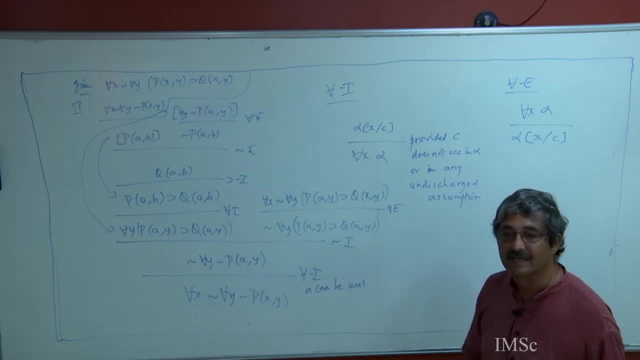 it Any other? Yes, So much of this is basically planning your discharging of assumptions a little carefully. that is all ok. Now let me do one with the existential quantifiers. any question? shall I move on? ok, Yeah, I am doing only examples that are fairly obvious. I am not doing anything. 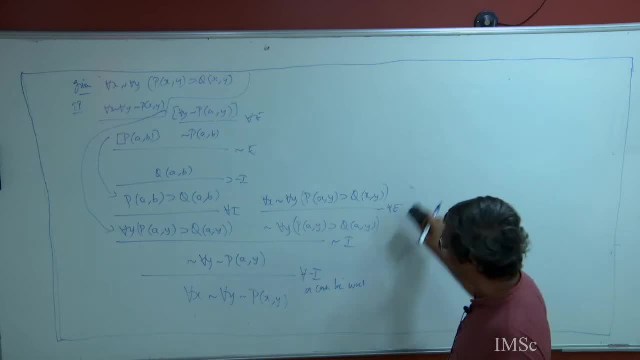 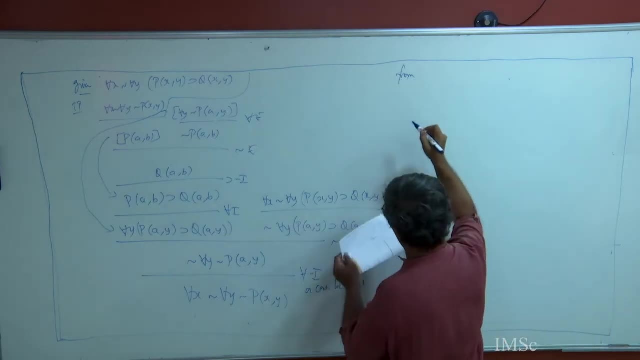 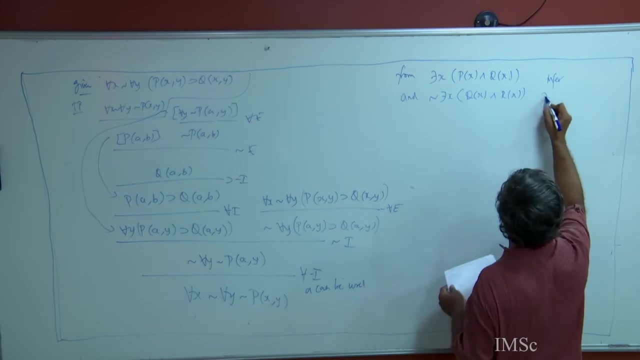 that is difficult in this, Semantically at least. ok, So here from yeah, this is: there exists x, p, x and q x, and not there exists x, q, x and r x. Yes, Ok, or it should be clear that this inference is sound. okay, So I want there exists x. 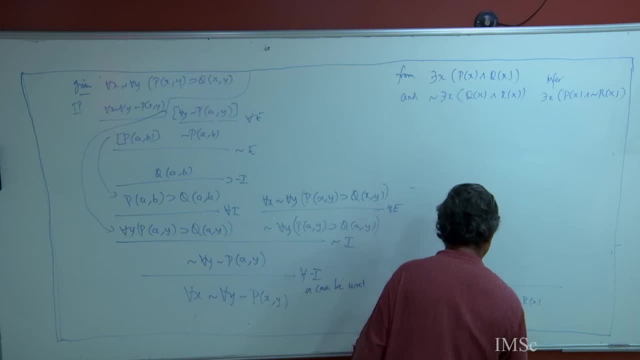 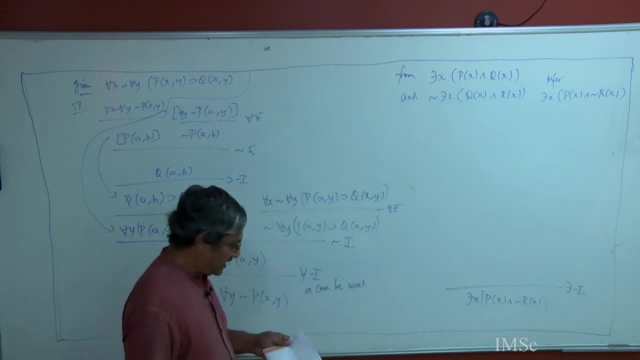 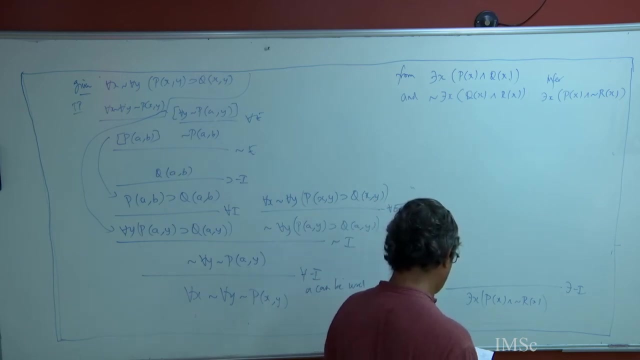 p x and therefore I need a there exists x introduction. So I am going to write this as p x and therefore I need a there exists x introduction. So I have done this with there exists elimination. So that is a deadly okay, Yeah, So this: 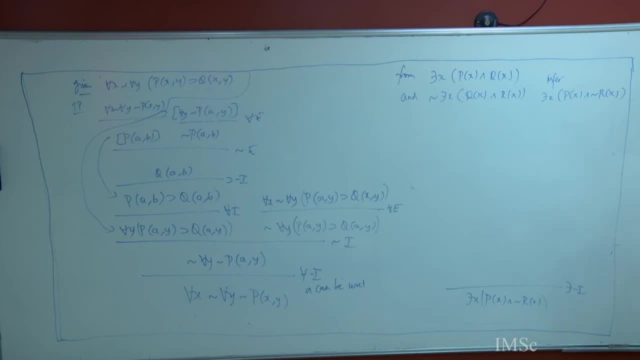 is a fairly complicated proof. Probably you can do a better proof and you do it. I just want to show one, At least a proof, that you would probably not think of. I do not know, Maybe you will, but I do not know. I wanted to show you a proof of this kind, So let us see. So I am going. 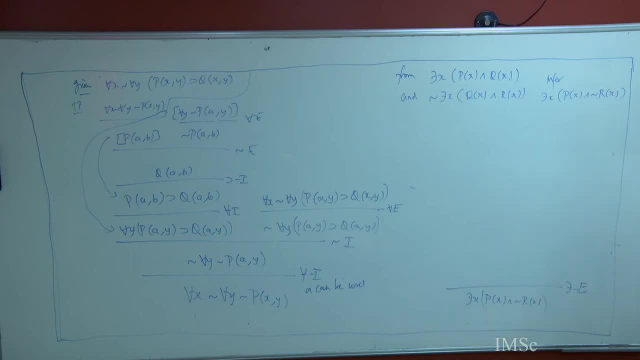 to do this by there exists elimination. How do you think you can do it by there exists x elimination? So what I have is this: So there exists x, q, x, and therefore I am going to write this as p: x. 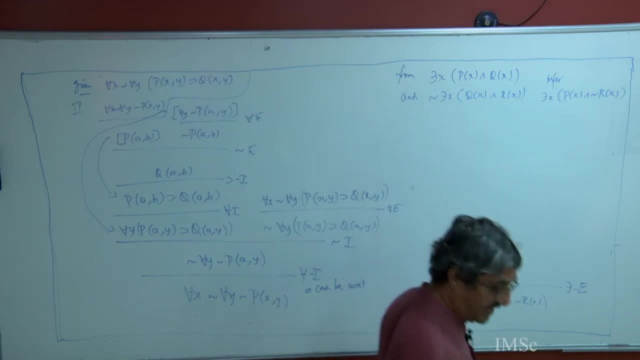 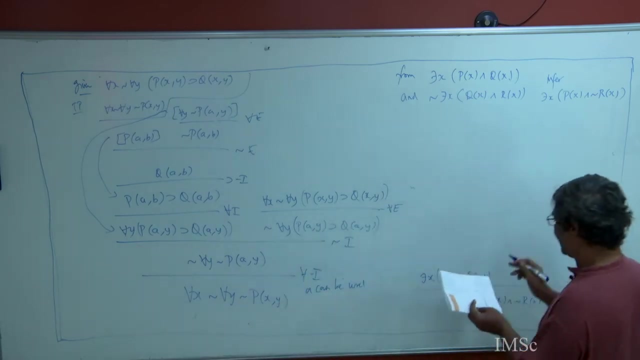 And now this is like p x and q x. So this is one of the assumptions given right I start with: there exists p x and q x And by making a substitution right I am going to derive there exists x, inclusion p x and q x. 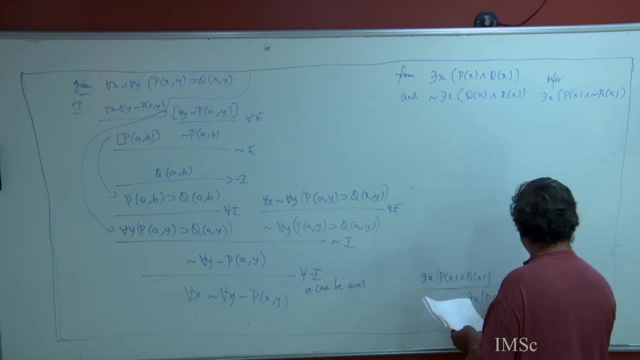 Okay, p x and not r x, by making a substitution, and so the substitution that I am going to make, P a and Q a, an assumption that will be discharged. So let me do the, let me work my way up, So 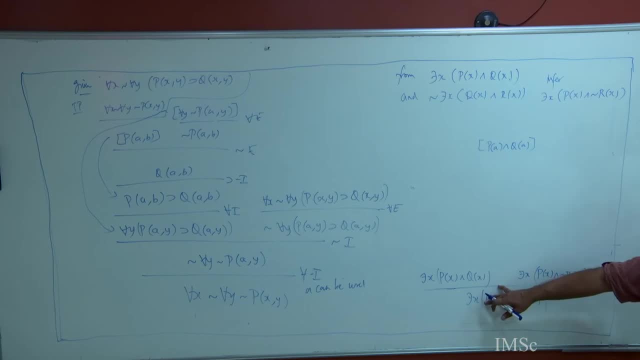 the deal is that I am going to make a substitution and so the substitution that I am going to. So the deal is that I am going to make a substitution and so the substitution that I am going to. So the deal is that- remember, this is the there exists elimination right. If I have got there exists x alpha and I take alpha with some substitution, make this as an assumption. from that I can derive beta. then I am allowed to arrive beta. 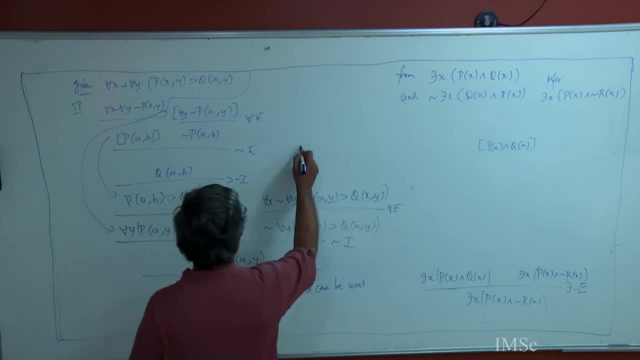 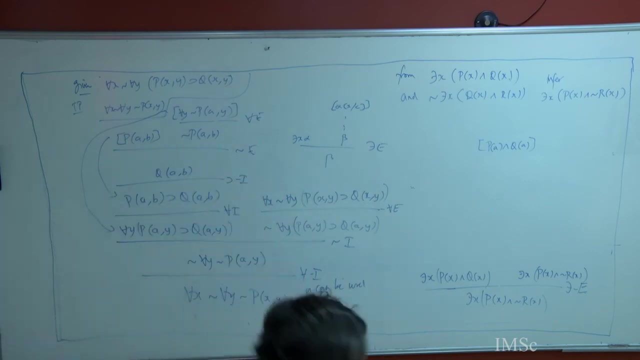 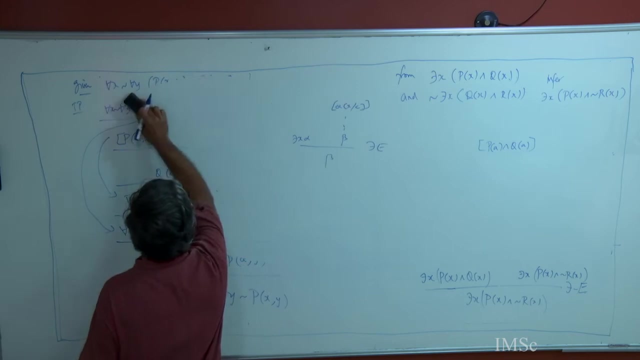 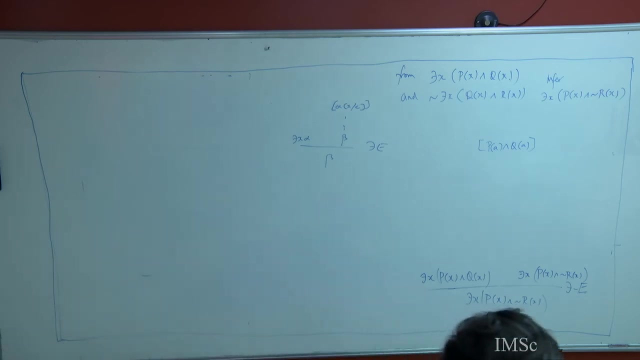 This is the form of the exists elimination rule. right, There exists elimination is there exists x, alpha alpha, with x replaced by c beta. from that I can get beta. So let us see, maybe I should get rid of these. So first here, this is from P a and not r a, and this is a straight forward. there exists introduction, So how do I get P a and not r a? 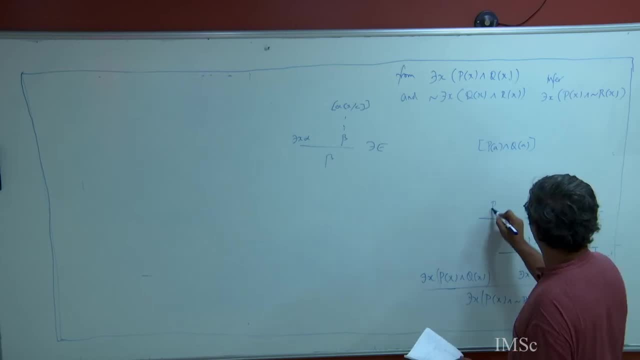 I get P a and get not r a. I get P a and I get not r a. P a is by this assumption, and that is easy. P A by this assumption, and that is easy. Maybe I should. I need a little more space. 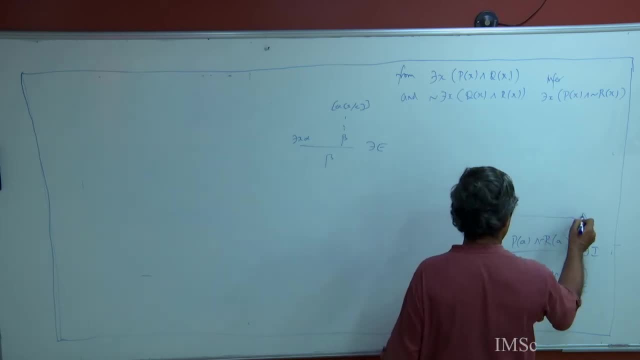 Maybe I should. I need a little more space, And this is from: let me get beta this. And this is from: let me get beta this empty state, sorry, and this is AND elimination. and here I have. I want negation introduction for not. 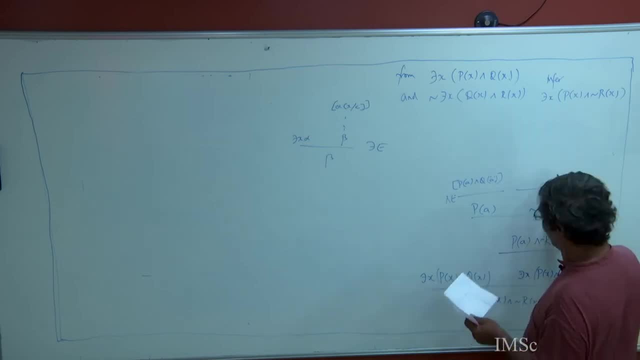 are they? So I have two. I need to get some contradiction. So the contradiction that I use is not: there exists x, qx and rx. This is an assumption that is given. So I get: there exists x, qx and rx. So that will be my contradiction from our assumptions. So 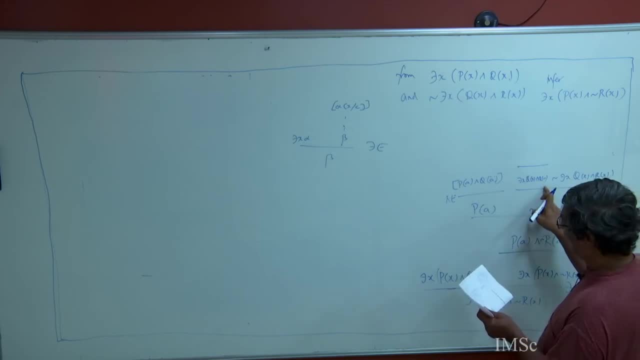 there exists x, qx and rx. This I am going to get by getting Qa and Ra. This is: there exists, introduction. Now Qa I can derive from Pa and Qa. Remember, this is the assumption that I am discharging, that is, AND, elimination. And what about Ra? 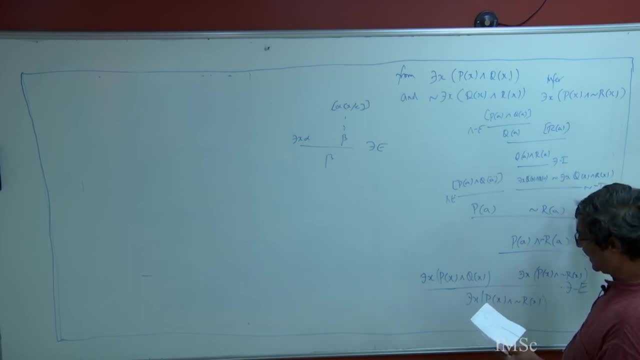 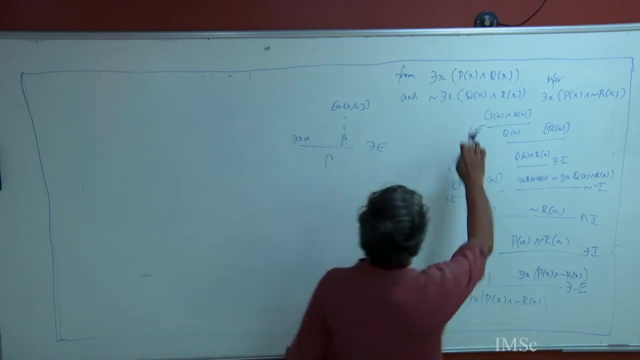 That is an assumption that I can get rid of here. yeah, I have gotten rid of it here, So that is it. so I have used both the assumptions, right. I mean, this is the assumption that I have used here and this is the assumption that is used here. 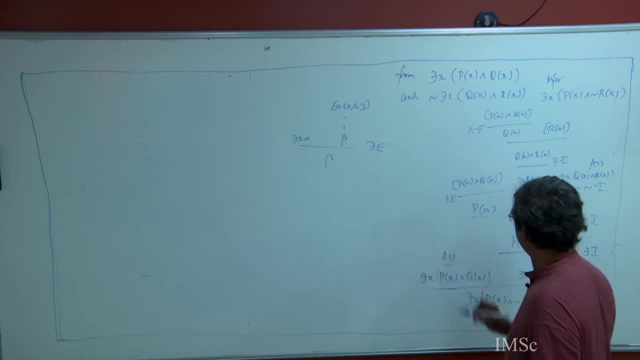 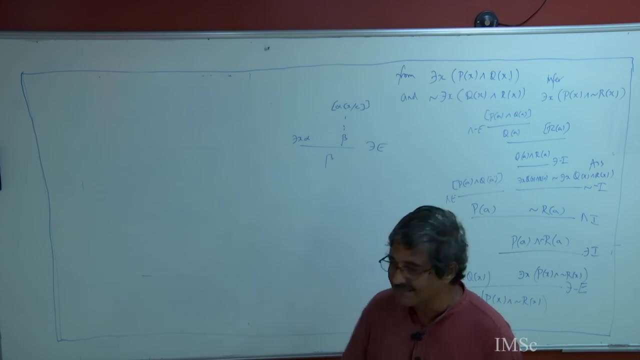 Yeah, So that will be my answer. Okay, Thank Yeah, Thank you. So, as I said, this is only to demonstrate the way these proofs are built and also to show that is a fairly tricky business in natural reduction when you go about, but at least. 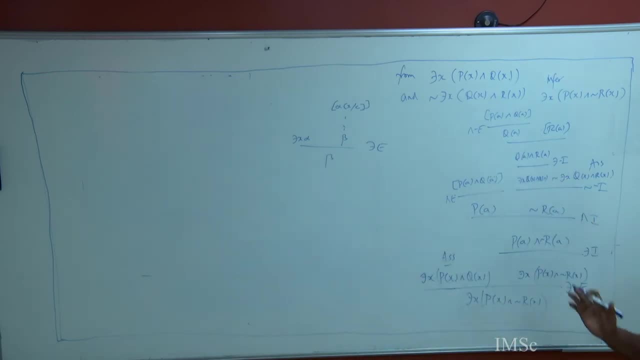 you can use the formula structure to see how- and this also shows how- why- with first order formulas are much harder to reason with than the propositional formulas that we were considering earlier. Mainly- and it is all to do with precisely the problem- that we spent a lot of time semantically. 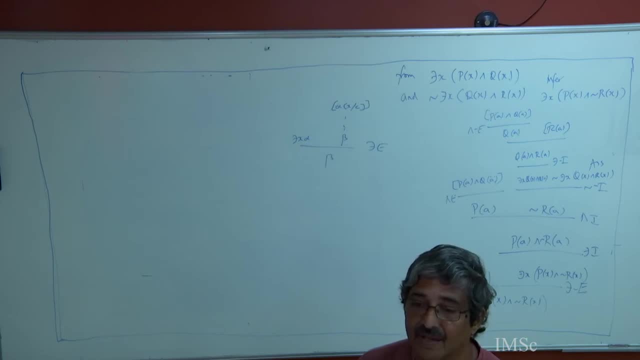 worrying about, namely about variable occurring, free, constant symbol used or not used in the assumptions, from which what you can conclude, etc. Okay, so any questions on this particular proof? As I said earlier, if you have any questions, please do not hesitate to ask. 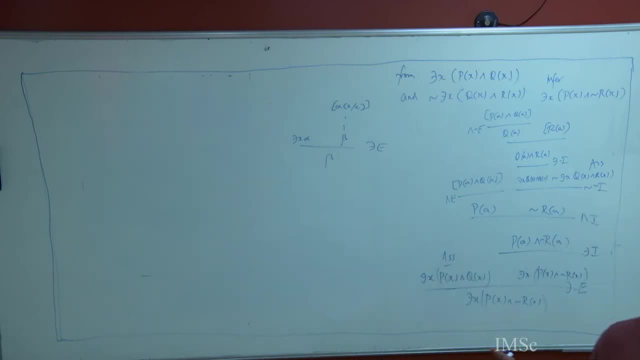 As I said- of course- I have said this many times- formal proofs. if you watch somebody do it, you can only see. you know, you can verify the steps, but it is hard to understand. You have to try out some things yourself and see how these things are used again and again. 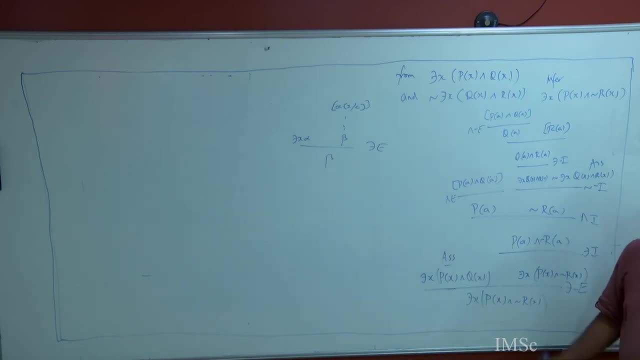 before you get some intuition into this, Any questions? Okay, so then I will. yeah, so that is pretty much it for natural reduction, Sequent calculus. the rules are very similar. Once you have seen the rules for natural reduction, the second calculus, of course, is much, much. 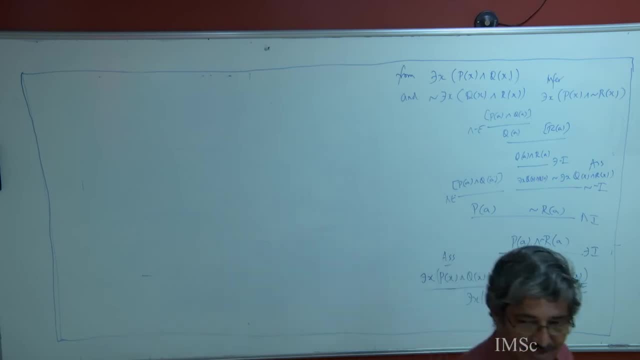 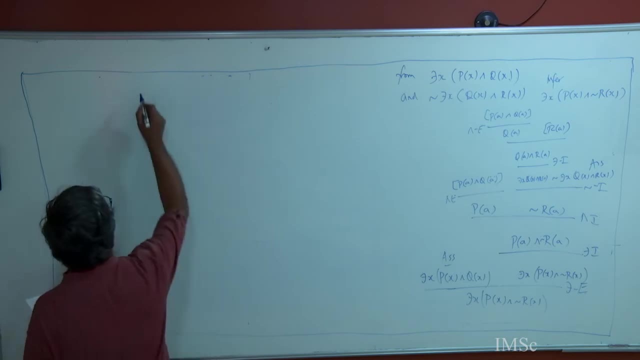 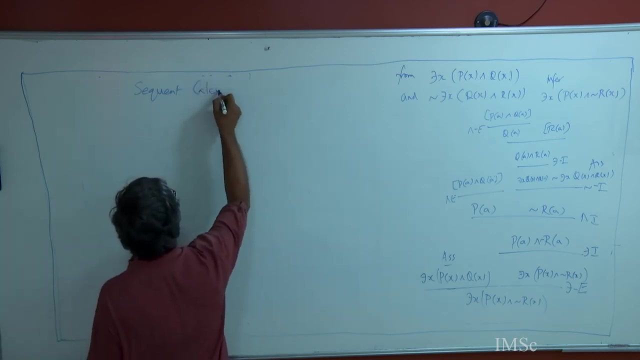 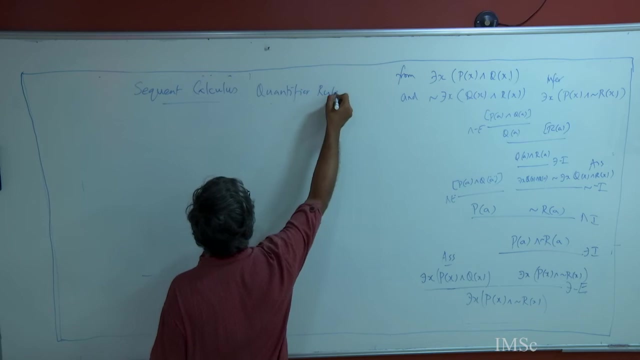 more structured. So it is, the rules almost pop out fairly. you know structurally You do not have to do, you have very few assumptions that you have to write down Sequent calculus, quantifier rules. I am not going to write out all those left rules and 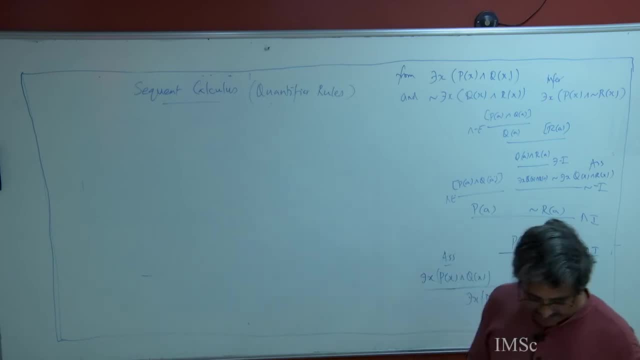 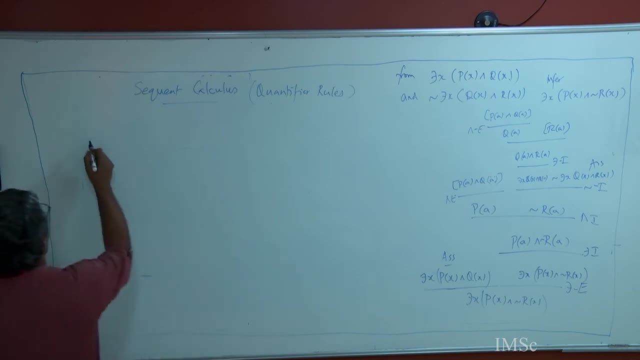 right rules for all the connectives. we have seen them earlier. So here, what are the rules? So you have a for all left rule and for all right rule, and you have a there exists left rule and there exists right rule. So what is this going to look like? 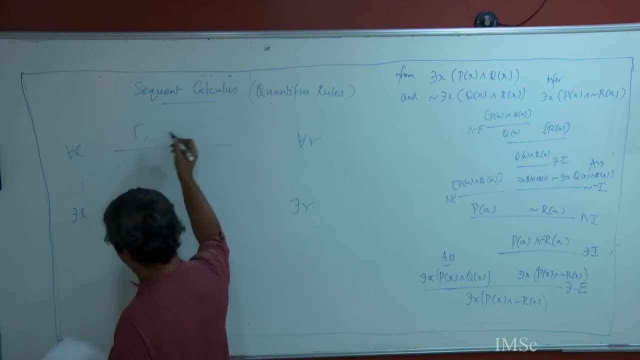 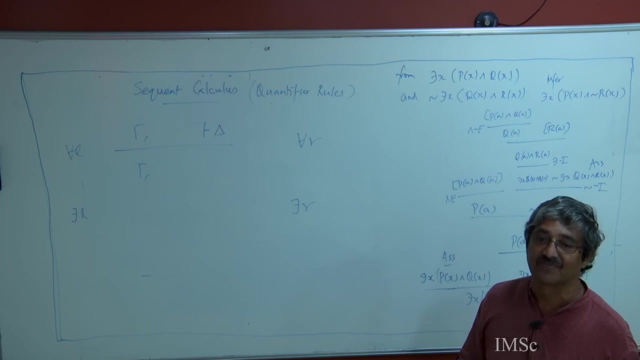 You have a gamma and delta, So you have to have some. so how does this go? Remember that in the sequent calculus, what is very nice is that there is no introduction and elimination right, So the connective that you are looking for always appears below the line. 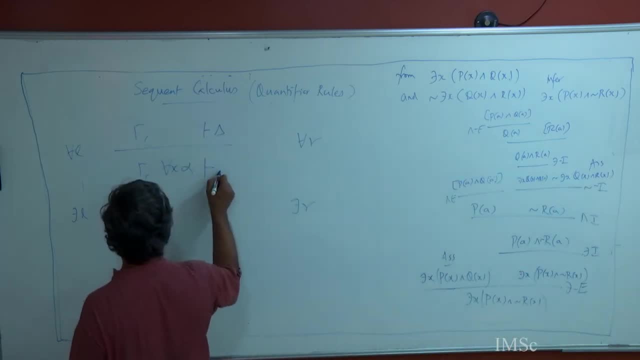 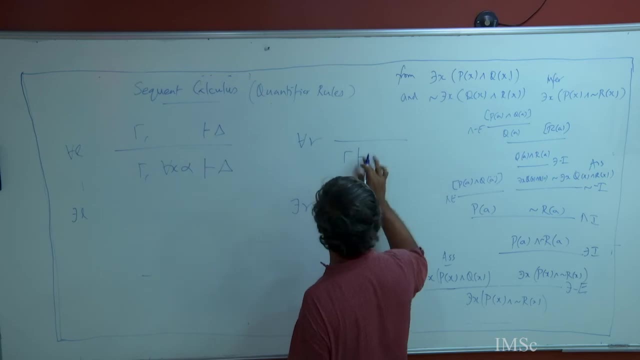 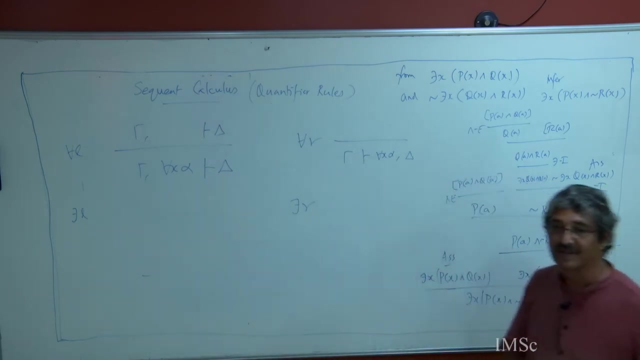 So this is the form in which you have got, yeah, And it is the form in which you appear on the right hand side. oh sorry, yeah, there is only gamma. so, yeah, So it is. So this is one of the most important things that you have got in sequent calculus, right? 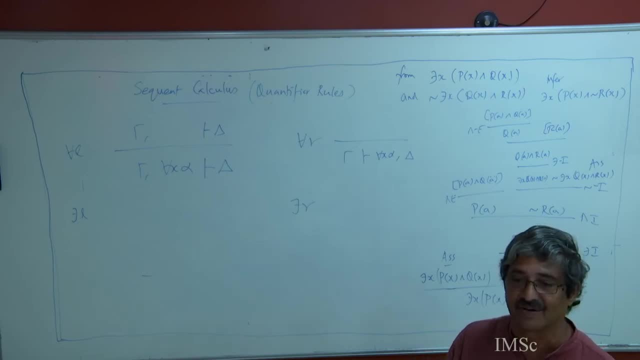 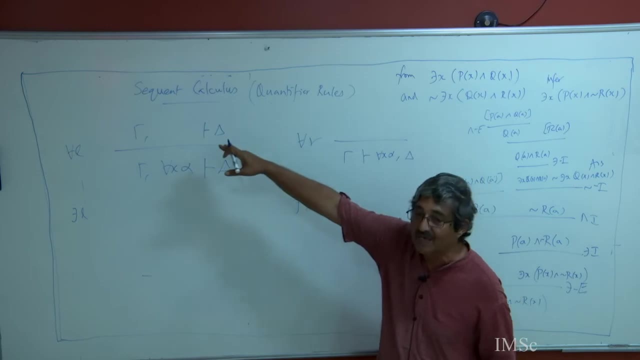 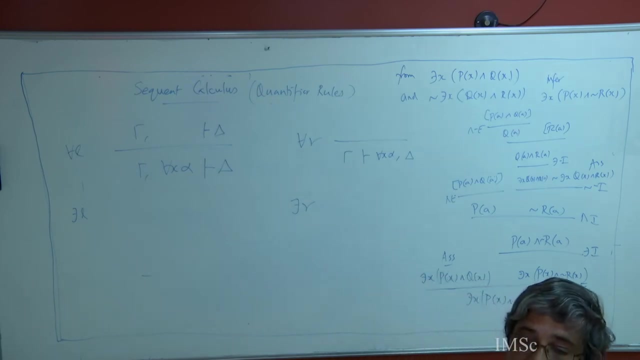 The logical rules have the sub-formula property. What is? you remember this? what is the sub-formula property? Anything that you have got to derive something. you have to look at only sub-formulas of the conclusion formula, right? So this is one of the important characteristics of sequent calculus that I discussed earlier. 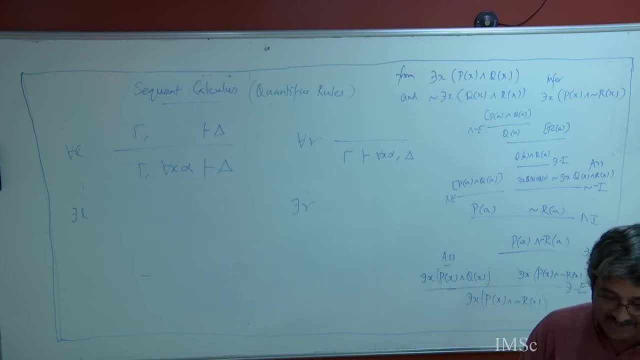 And that is true in propositional logic, and it is true in quantified logic as well. 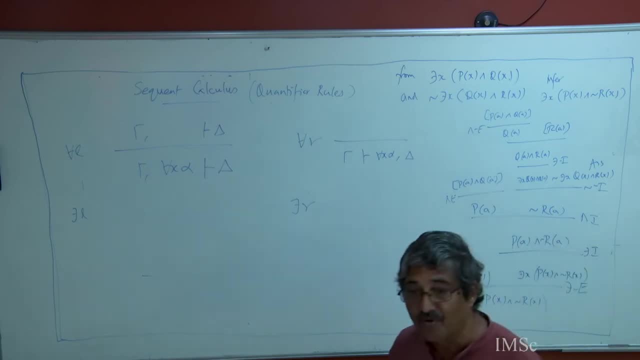 reduce inconsistency it has. it violates sub-formula property, So you look for cut elimination. This is one of the important reasons why proof structure is comes out in sequent calculus. So you know that when you look at for all rule, left rule or right rule, 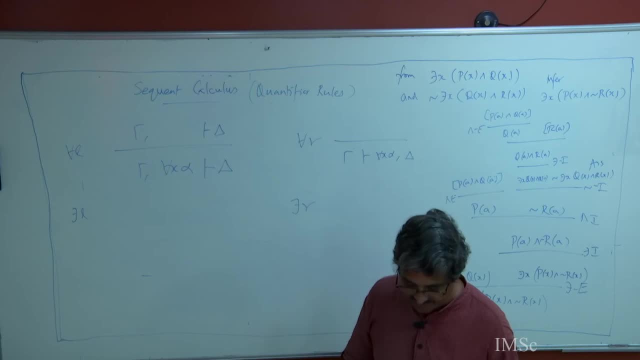 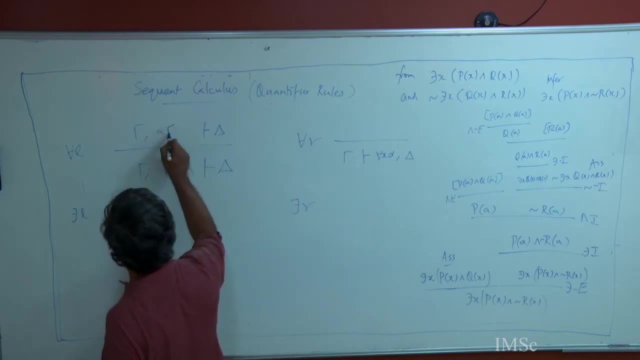 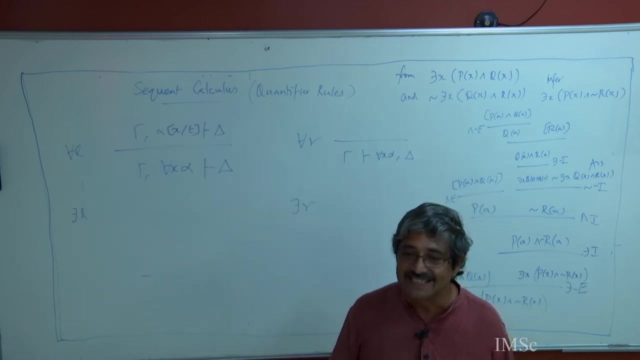 it is always going to look like this. So what is going to be on top? It should be fairly easy. Well, this is. it does not matter whatever term, right, This is the generalization from constants or variables or whatever you have got right, If that is your remember left. 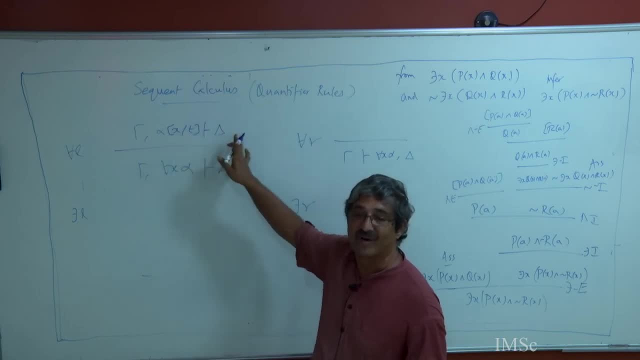 hand side. is your assumptions right? Assuming this: if you have got this, then you have got for all x alpha. And what about this one Where provided x does not occur free in the conclusion? yeah, This is the analog of saying that alpha implies for all x alpha. 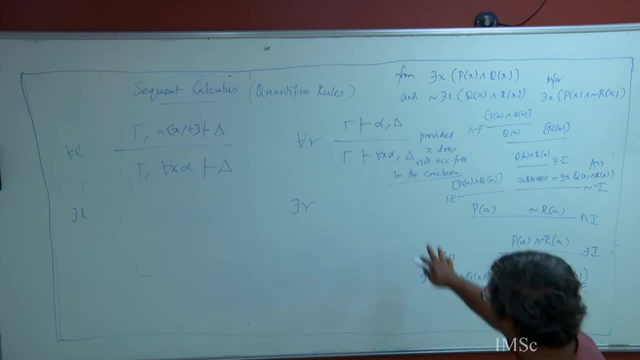 where x has no free occurrence in alpha. Except that now this is in the entire conclusion that x has no free occurrence in gamma, which is x, ok. X does not occur free in gamma. in for all x, alpha, delta, right That? so this is the. 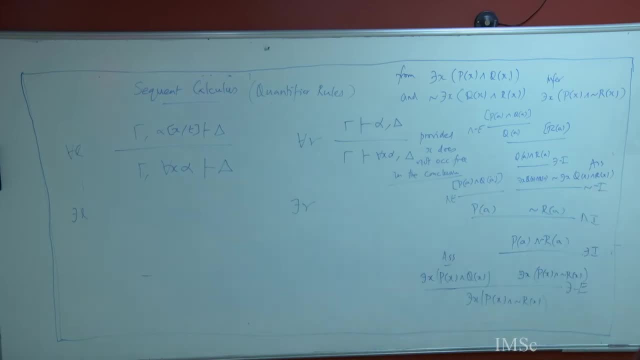 difference now? And what would be the rules for the existential quantifier? What will be? there exists L and there exists R. remember, there is no choice in the sequent calculus. it's strict duality right. it's not like natural reduction, where 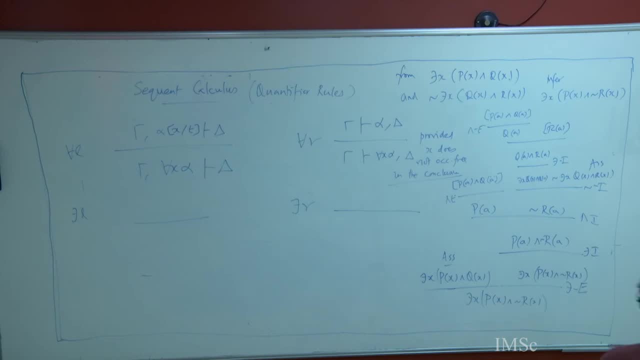 and introduction and or elimination look different. right conjunction- introduction and conjunction, disjunction, elimination look different in natural reduction in sequent calculus: whatever is the left rule for conjunction is the right rule for disjunction, whatever is the right rule for conjunction is the left rule for disjunction, and so on. 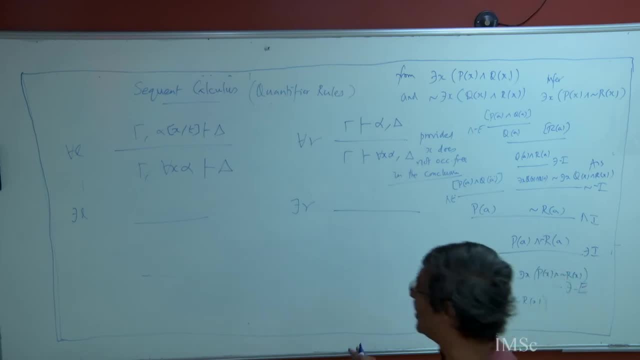 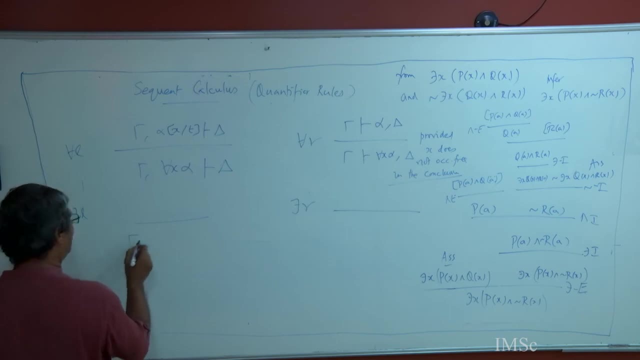 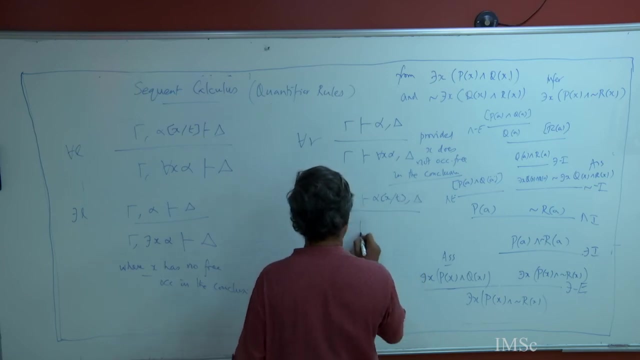 right. so there is absolutely no choice in sequent calculus. the moment you have written your for all right rule, the for all the existential left rule is has to be this: where, for all all x has no free occurrence in the conclusion, and this, yeah, if you have derived a conclusion alpha. 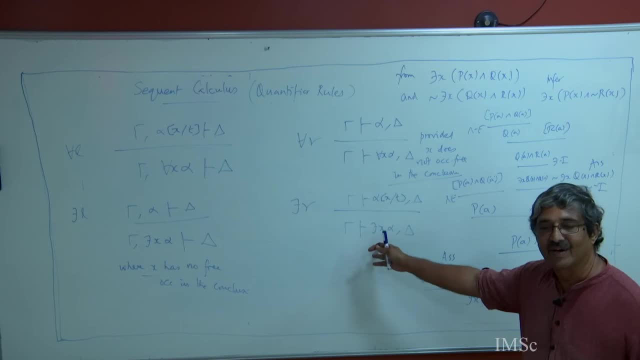 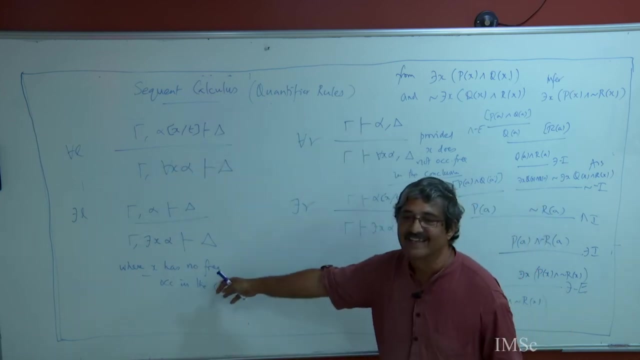 for some particular term, then you can derive the conclusion: there exists x alpha from these assumptions. so you know, this is exactly how it has to be. so this is in fact the more natural rule. this rule dictates the for all left, rule right, and this rule dictates the there. 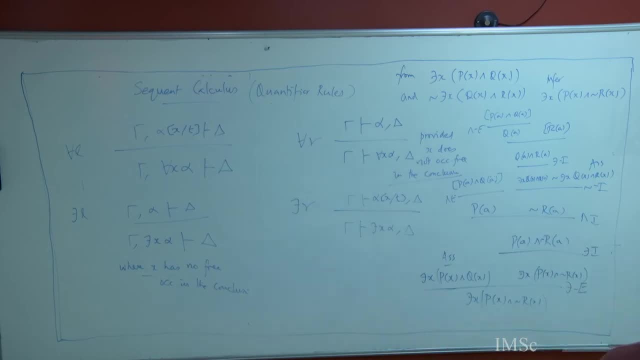 exists x left. this is how sequent calculus you know, you. I mean, it's like a technology, right, it's like a machine. there is some. one part is driven by semantics, the other part by duality. everything is structured exactly that way. that's why it's really neat once you understand how. 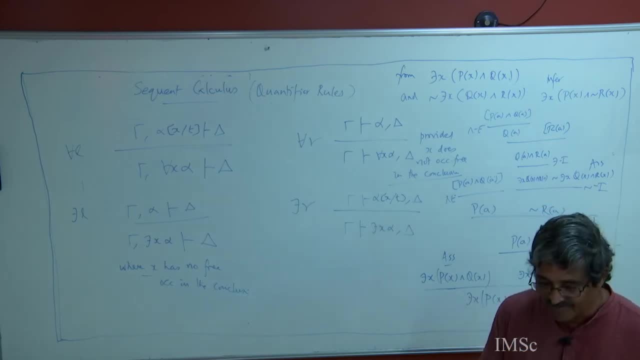 this thing is. and second, calculus you can design. if you think of a new connective, you can design the logical rules for sequent calculus for that connective. you know it flows almost right. okay, so that this is sound should be pretty straightforward, right? because the arguments for why this is sound is: 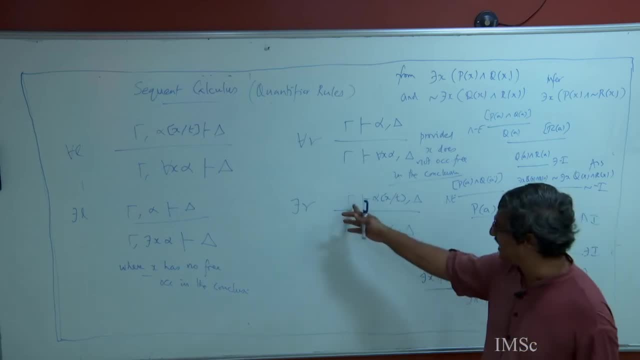 exactly like what we have talked about before, right In a sequent. what does this mean? The conjunction on the left hand side implies the disjunction on the right hand side that that is a validity right. So if the conjunction of all gamma 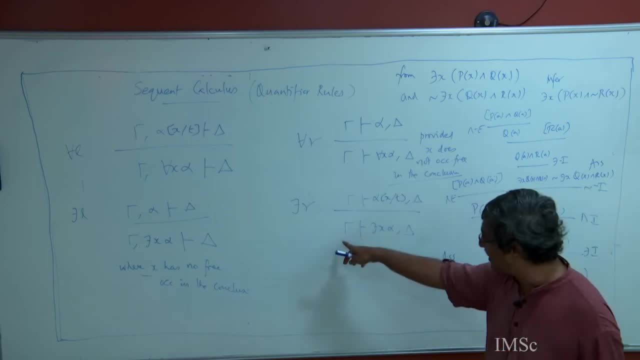 implies the disjunction of alpha or delta. you want to show that the conjunction of the gamma implies there exists x, alpha or delta. As I said, consider a model in which all of the left hand side is true. You want to show that one of the right hand side is true If 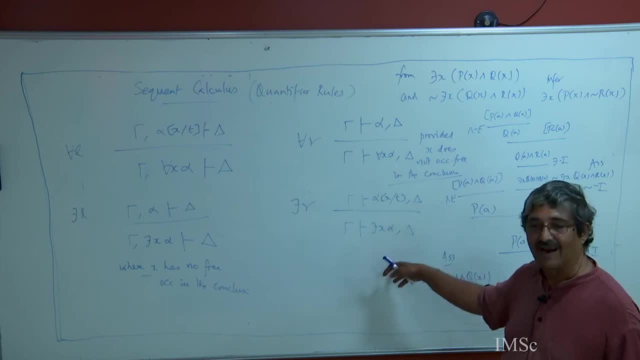 one of the delta is already true, we are done. Otherwise, you want to show that there exists x. alpha is true, But it suffices to show that alpha holds for some particular witness, and that is it right. So there exists x, alpha holds. This is pretty much the order of things. 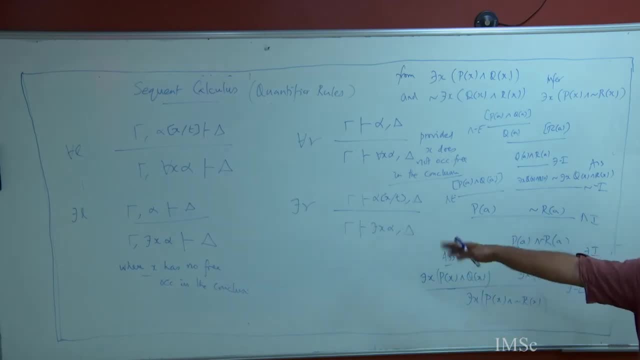 in the ok. Any question on the formula? I hope the site, The site conditions are clear, right. The site condition is: what is the site condition? It says that it should not be used. there should be no free occurrence of x anywhere. 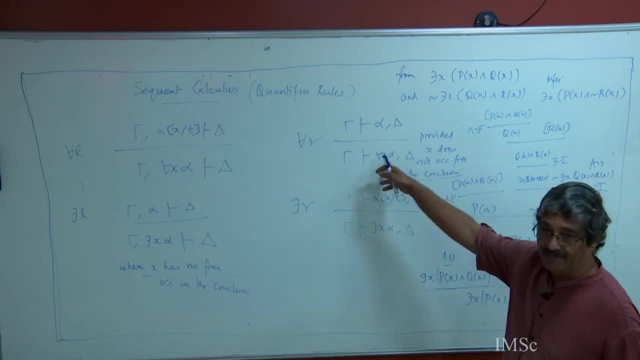 in the conclusion. This bound occurrence is ok, right. There should be no free occurrence anywhere in the conclusion. That is it, And any ok Is the idea clear. So, and the main point is that there is no business of making assumptions. 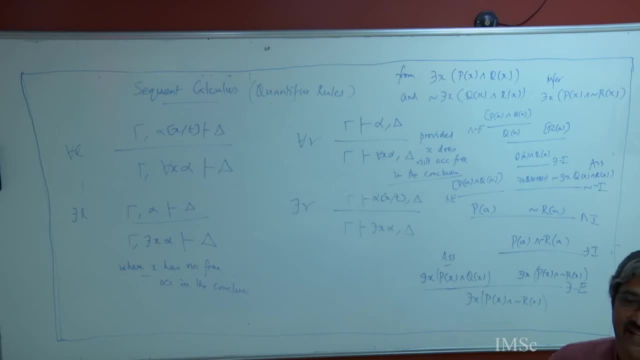 discharging them. all that nonsense is not there, right? So it is a fairly clean system that you can work with. You do not have to worry about those scoping things, right? So it is a fairly clean system that you can work with. 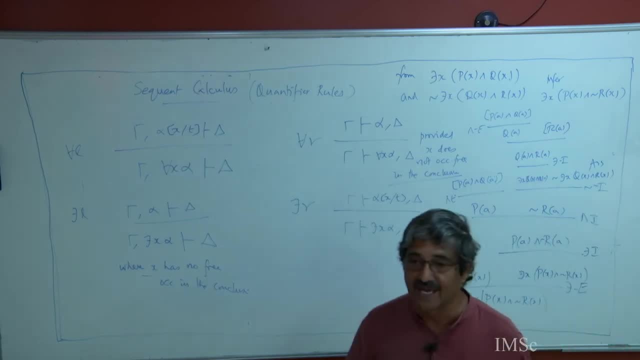 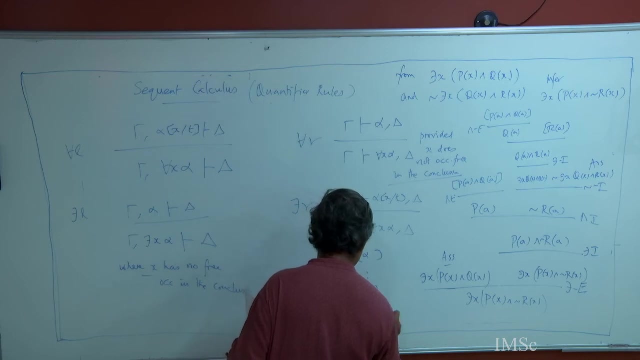 Yes, All of the things that remember. in a sequent calculus I mean natural reduction. one of the most difficult things to keep track of is right. When you make assumptions- alpha and then beta, you have to discharge beta first and then alpha, right, So it is fairly. 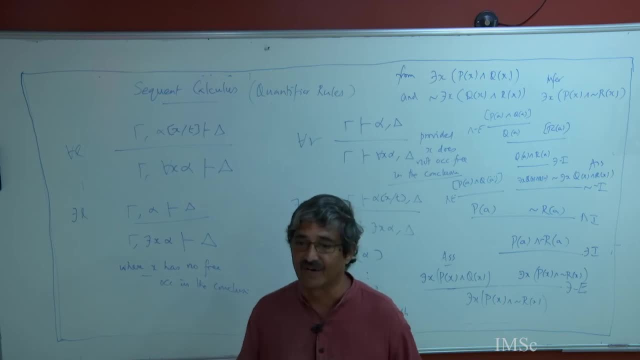 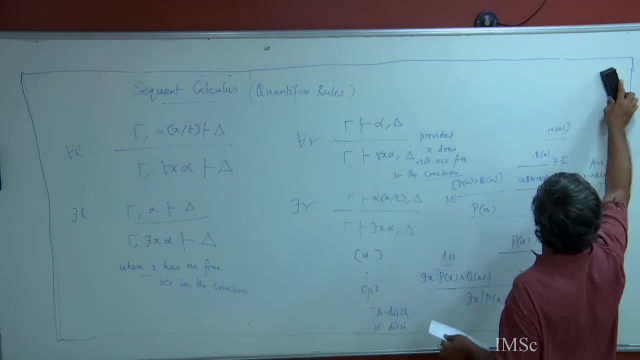 important to make sure that you, so the scope is very careful, right? You cannot cut across. Yes, Yes, Yes, Ok, And so all that is not there in the sequent calculus. you ensure that, So just leave that. 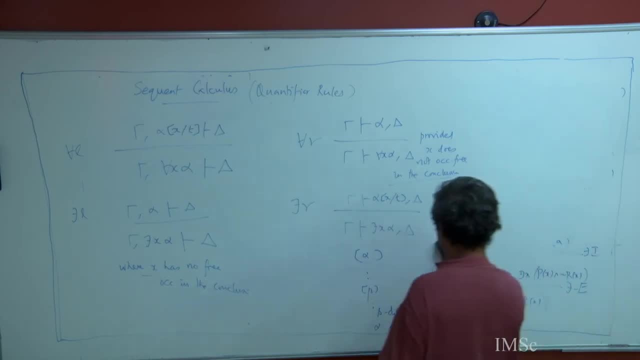 here and you can see. So let me give you a few examples again. So here is a proof: Use for the for all quantifier. So, for instance, I want to show, and something fairly obvious for all y, Yeah, So I use the. 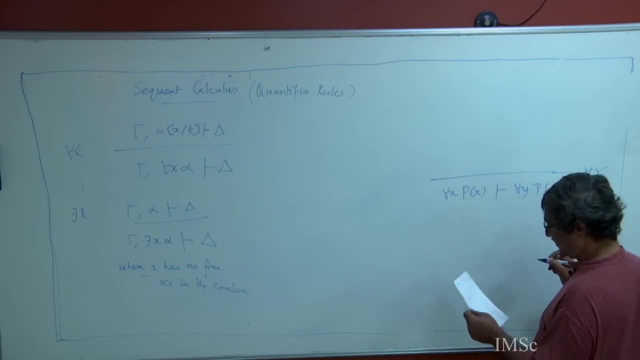 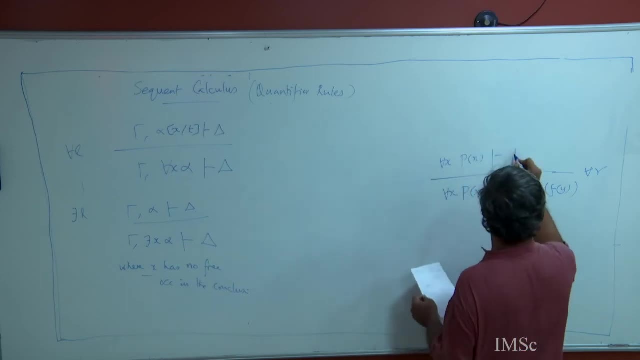 Yes, If you the for all, write rule for all: x, p, x. yeah, Remember y. I have to make sure that y has no free occurrence in the conclusion. y has no free occurrence here and y has no free occurrence here. So this is important: y will occur, bound. bound occurrence is okay, right. 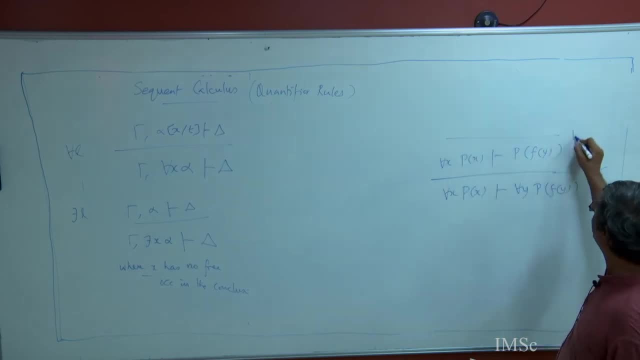 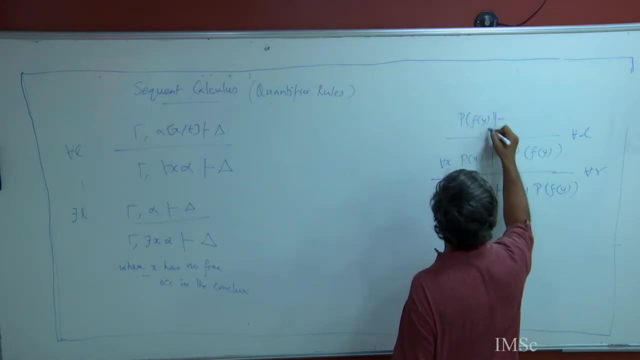 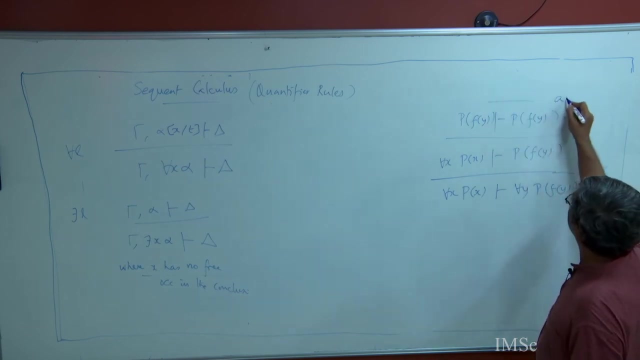 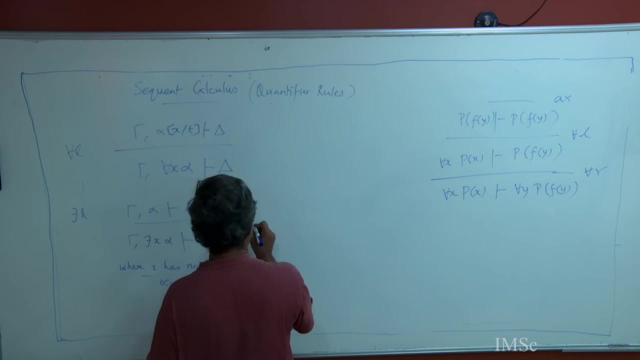 So this, the for all write rule is okay, and now I use the for all left rule, right, yeah, And, and this is okay again for so, and this is axiom, yeah, The Okay, So some more. here is one Again, I am only doing obvious inferences I want to get for. 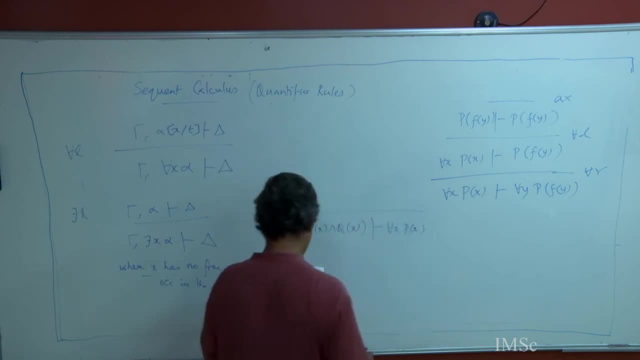 all x, p, x, So once again I can write Okay Y, because going from here to here, there is no free occurrence of x anywhere in the conclusion. yeah, Below the line there is no free occurrence and therefore I am allowed. 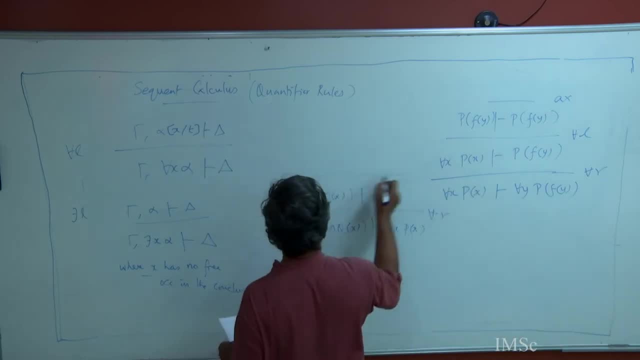 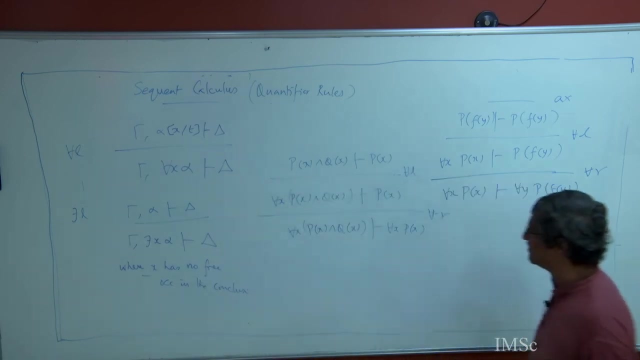 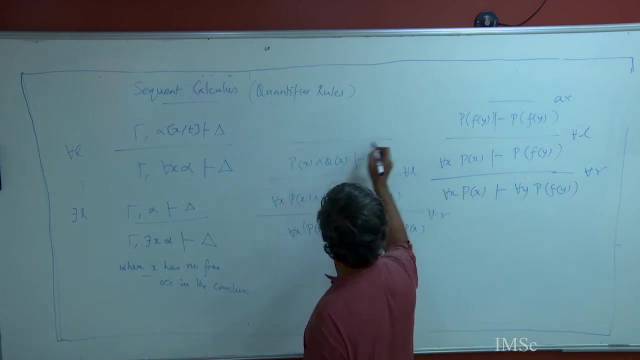 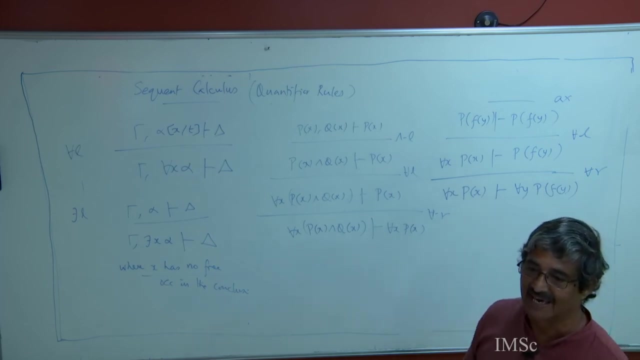 that. so I can, okay, And this one, p x and q x, Okay, Okay, I can use for all left which is: and this, this is, and left rule. Anyway, a list is the same as conjunction on the left hand side and the list is disjunction on the right hand. 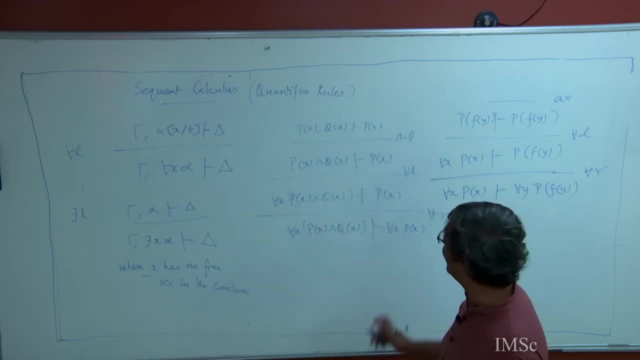 side: Okay. Similarly, you will have the for all right rule, and this is axiom. So I am also doing it to show you that how, in sequent calculus, the proof really flows. Okay, Natural reduction: for all its naturalness, the choices can be quite horrible. 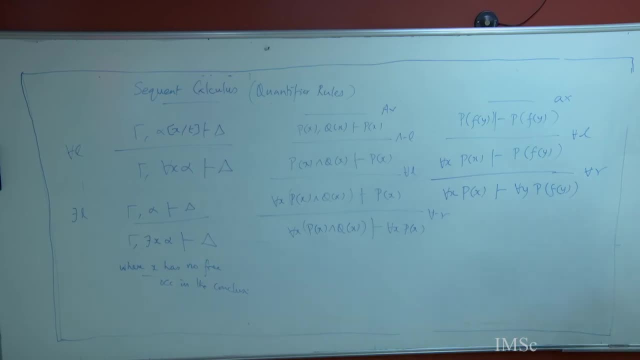 In sequent calculus. it is much, much more. okay, maybe nothing is straightforward, but yeah, I guess it is really me showing my preference for that rather than anything else. Okay, So suppose I want to derive. Okay, For all x. alpha implies beta. 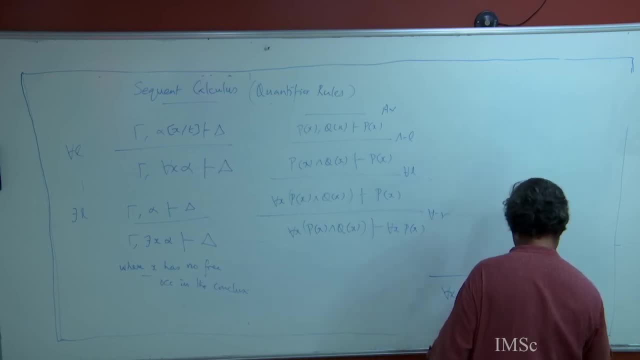 From that where Okay, Okay, And this is the validity of this is you have seen this before? I mean, this is, I think, one of the first problems that I had, given that for all x, alpha implies beta implies alpha implies for all x, beta if x does not occur free in alpha. 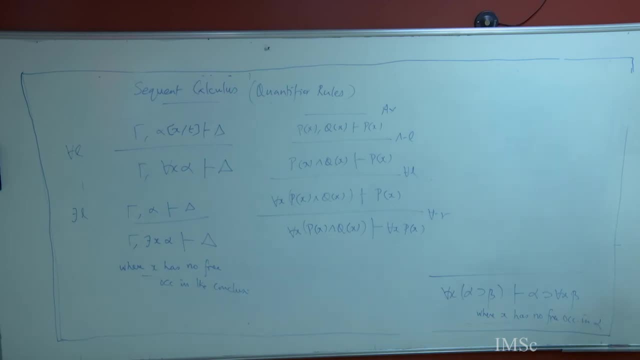 Right. So we know there is. there should be a proof of this. Let us do the proof. So once again, I am going to do implication right and implication right will come for all x alpha implies beta alpha from that, if I can get for all x beta. 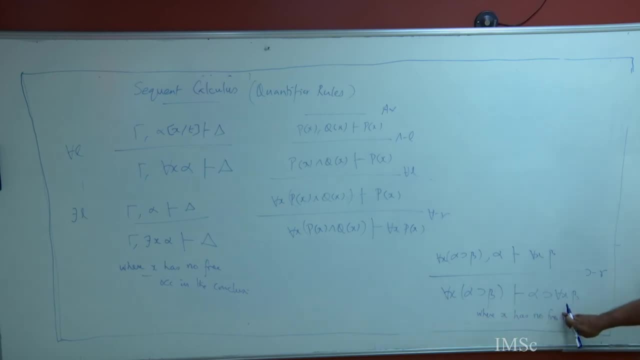 Right, How do I get an implication to the right? Assume to get alpha and beta or whatever gamma implies delta. assume gamma, show delta. Then you can. this is the implication right rule in sequent calculus. So now this is fairly straightforward. 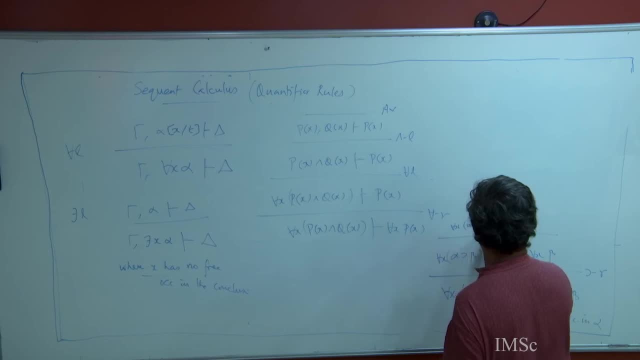 For all. x alpha implies beta alpha. I can get beta for all right And verify the condition. The condition is clear. Okay, So x has no free occurrence on the in the conclusion, And now I can do beta. this is for all left. 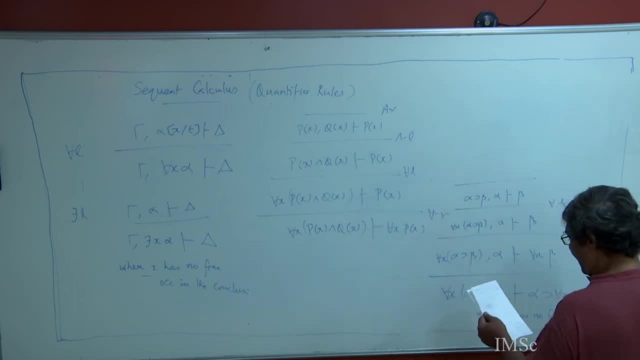 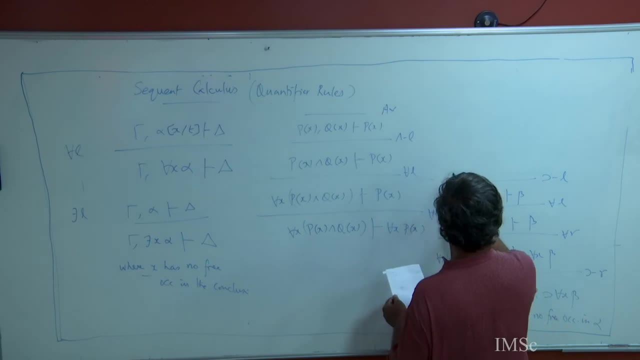 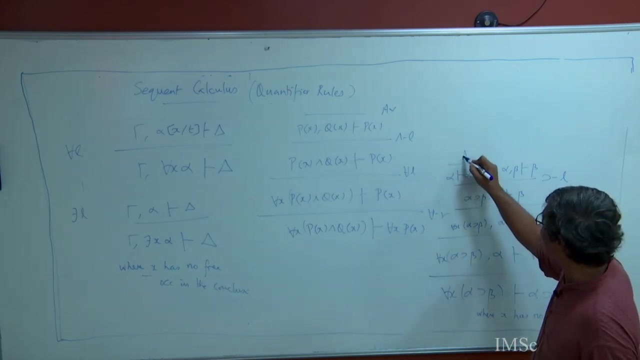 And now I want implication left, Implication left. I have to have both, both sides, Okay And yeah. And this is, both of them are x, yeah. So this is, as I said, another straightforward one. Let me maybe do one with existential quantifier. 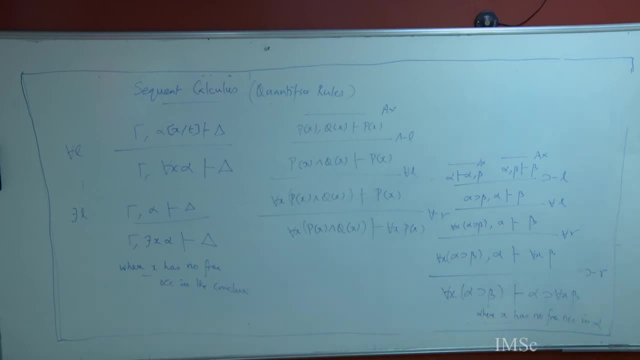 Yeah, So this is So, as I said, one okay, So I will. There exists x, Px or there exists x, Qx derives there exists x, Px or Qx. so I want R to the left. so I have. from there exists x, Px, I derive there exists x, Px or Qx and I have. 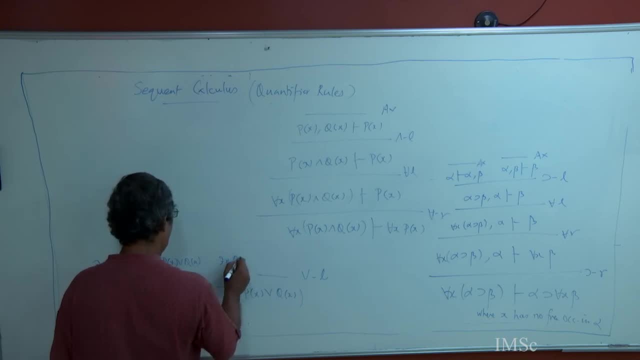 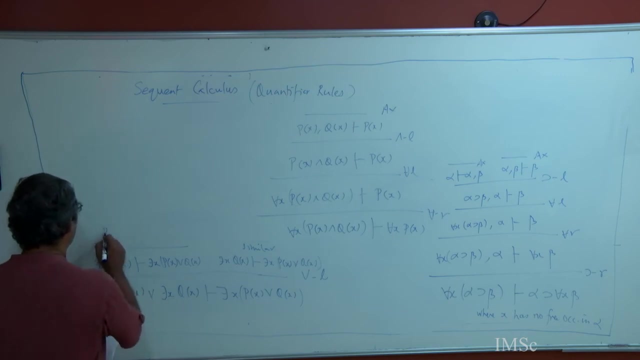 another one. there exists x, Qx and let me do this side of the proof. this one is similar. I am not going to one side of the proof, I will do and it will follow in the almost the same way. So from Px I will try to derive. there exists x, Px or Qx. this is the there. 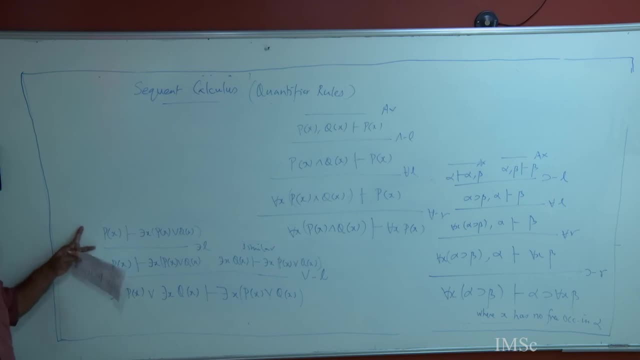 exists left rule. whenever you have got something here again, there is no free occurrence of x below for there exists L, I have to again check. so I will just write check. and now I want from Px, Px or Qx: there exists right rule. there exists right. there is no check. 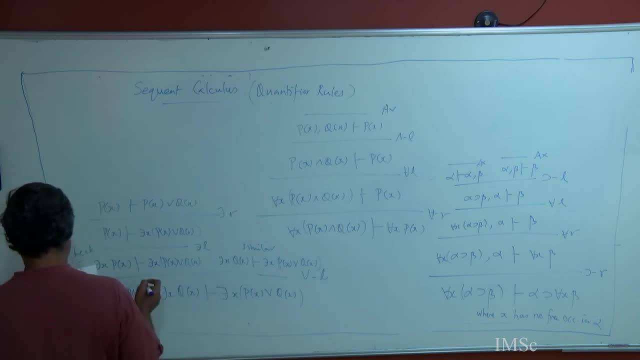 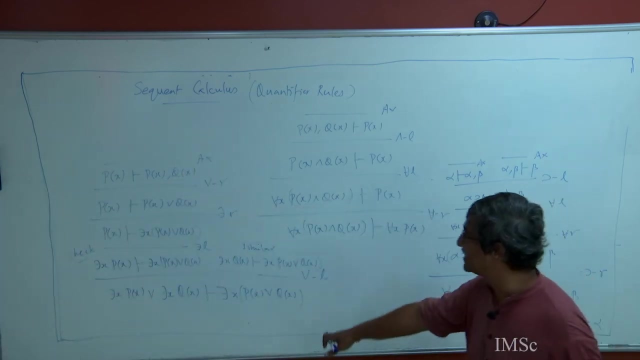 and anyway, this is true, And This is R to the right and this is x. you are going to have a pretty much the same proof structure on this side also, So the way the proof goes should be fairly clear, right? because? 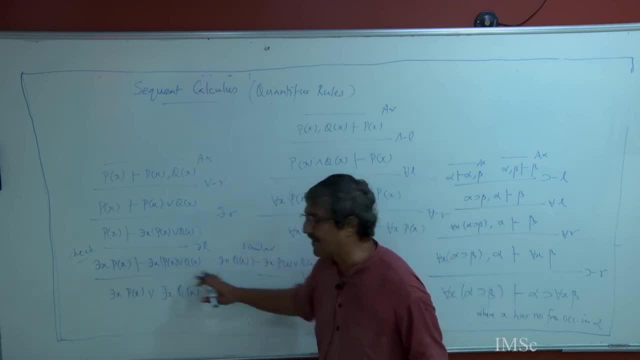 you have got a disjunction in the assumptions. you have to show this separately for each of the cases and in each of the cases you realize that there is a symmetry, whatever I do for Px or Qx. 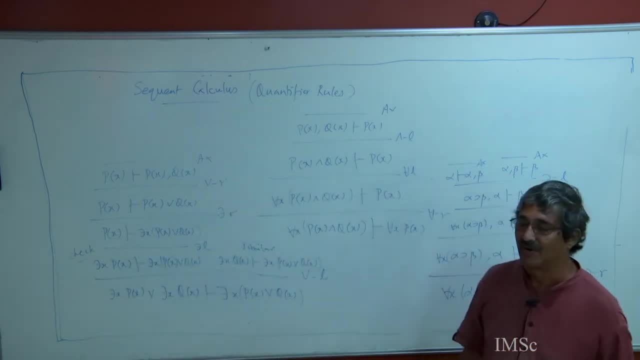 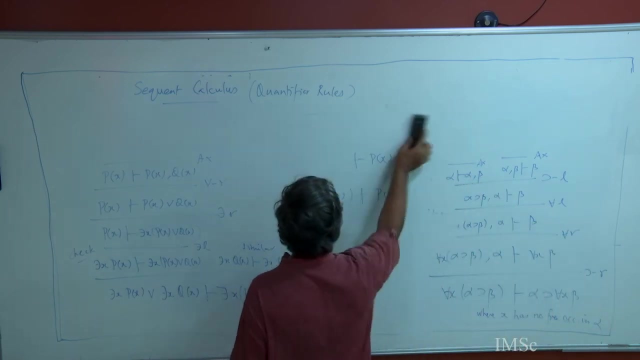 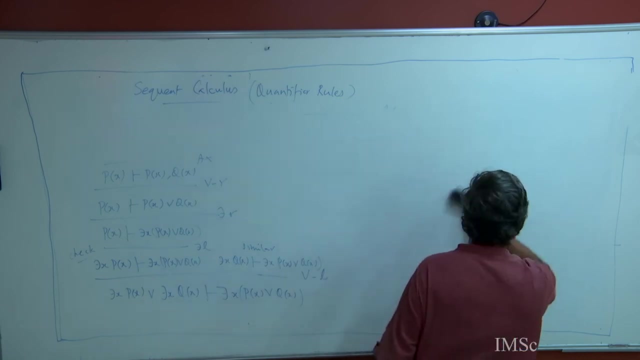 me do a slightly different kind of example, because I should have done this with natural induction also. I am sorry I forgot that, So I am going to take up one where you: the formula that you are trying to derive is not valid, So there should not be a proof, right? how do? 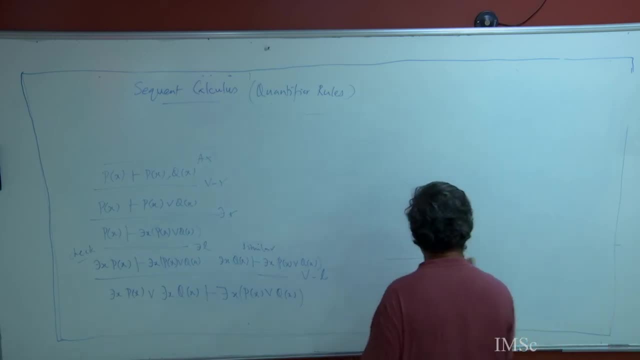 you check that that happens, right? So let me try to prove: there exists x Px and there exists x Qx. from this I will try to derive: there exists x, Px and Qx. this should not be possible, right? we know that this is not possible, right? you can always have: there exists x Px. 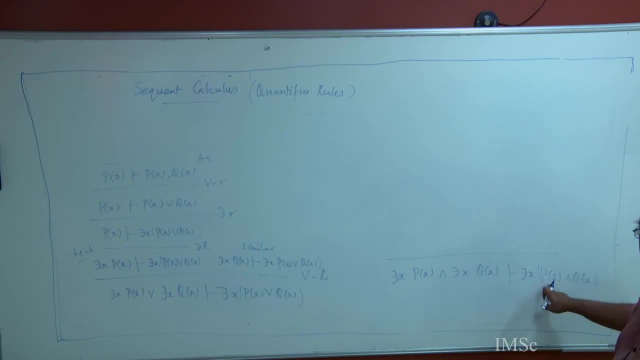 and there exists x negation Px. but you cannot have there exists x, Px and negation Px, right that You cannot have a contradiction with an existential quantifier. So this proof should not work, right? So let us see how it goes, because I am trying to tell you that there is like a 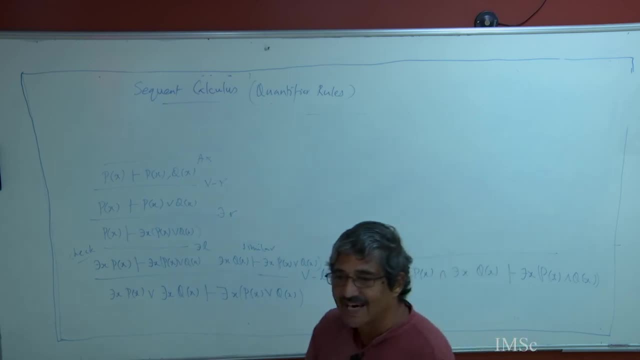 machine know in each case, you can start doing it and derive a proof. So what should happen in this? So let us check it out. So first you have an AND left right, So you must have, and this is the thing that comes for free. there exists x Px, there exists x Qx, there. 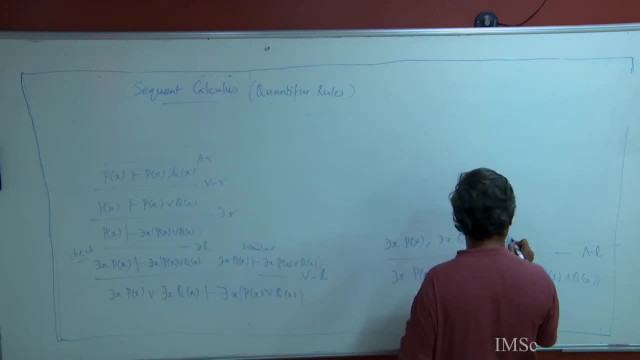 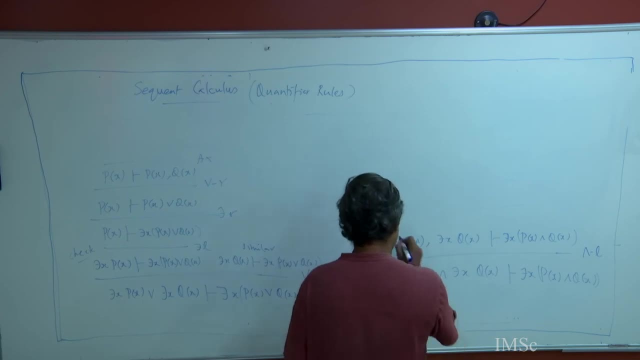 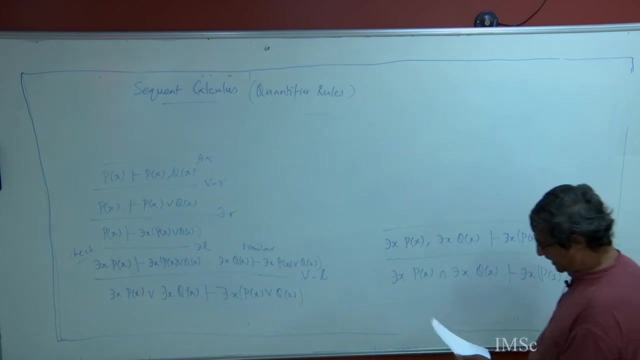 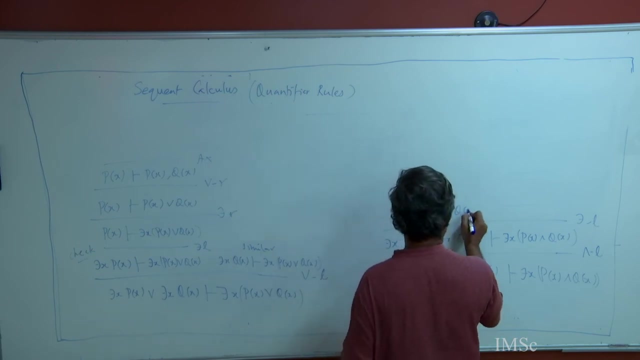 exists x, Px, there exists x, Qx From that I want. ok, Now I have a. there exists on the left hand side. it does not matter any one of them, let me pick Px. there exists x, Qx, and this is the same right hand side. So 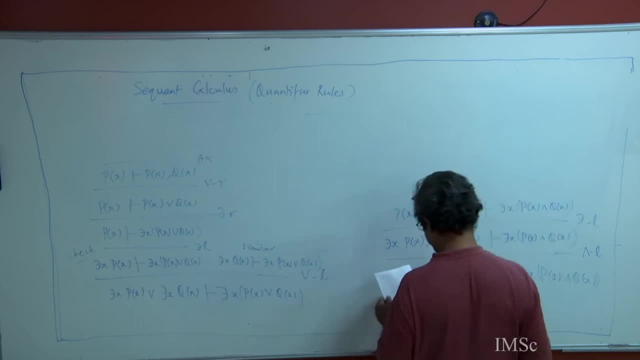 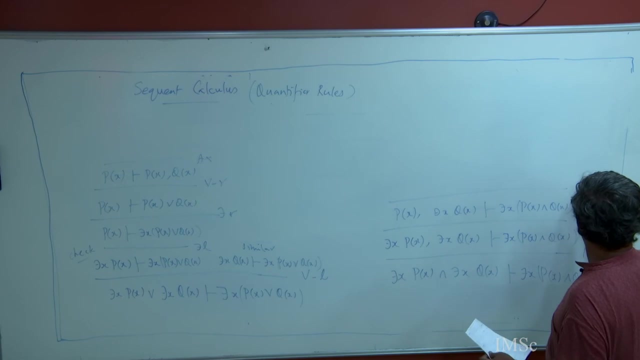 let us see how it goes. So now I have a there exists x, now I have a there exists left, and now I already have a problem. X is occurring free out here, right, So I cannot have Px, Qx and Px there exists x, Qx, right, So I cannot have some one. now let me go ahead and check. 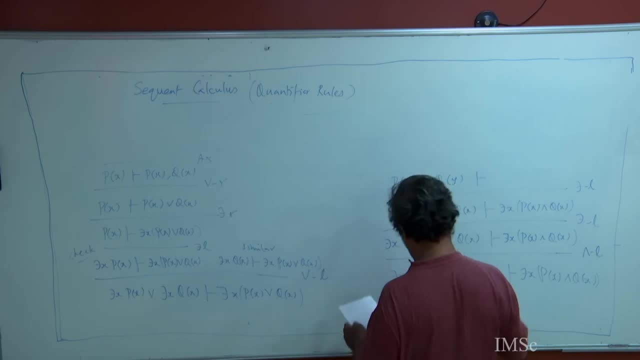 q x here, So I must have q y here, p x, q y and there exists x. Is this clear? When I am applying the there exists l rule right when I am knocking off the existential quantifier, you could knock it off once, but not twice. Second time, when you look at it, x is occurring. 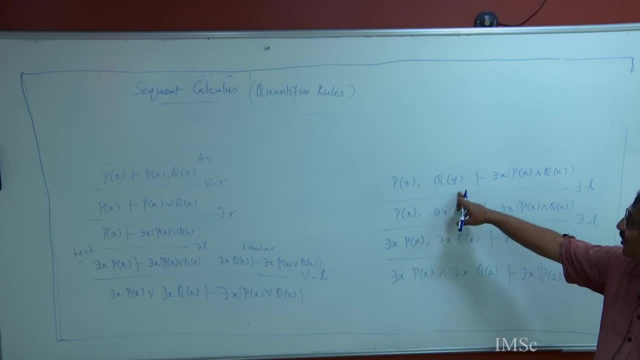 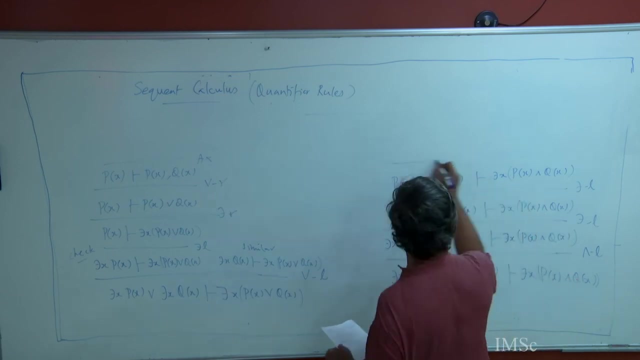 free, So you cannot have x coming here, So you can only have some y, and now you are going to have a problem because I am going to have. now, if I do, there exists, I will get p, x, q here And you would not get a single and you are stuck right. 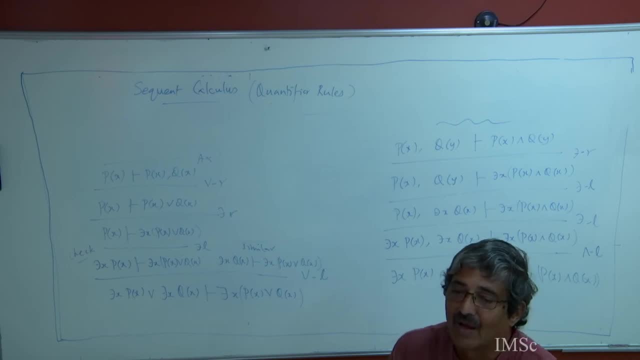 And that is, you know, for me at least, an illustration of how you are. you cannot find a common instance right, a single substitution that makes both the same, And so this is the sort of thing that you From this there is no way to get. I am sorry, you want p x and q x, and there is no hope. 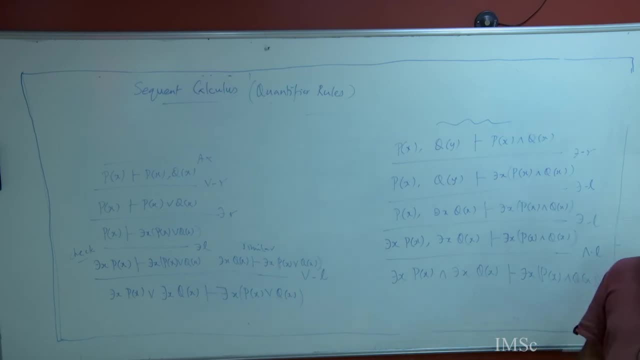 of yeah, providing here, yeah, So there is no way from p x and q y to get p x and q x, And so sequent calculus. what is very nice is that it keeps pushing, finally till you get the atomic formulas, where the axioms hold right, The, and at that level you will find 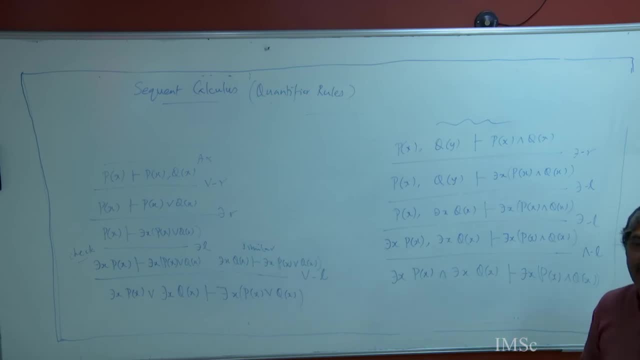 your inconsistencies. Yeah, Until then you have. you keep manufacturing lots of variables, new terms, whatever, but that is where it stops, ok. So, as I said, this is an illustration, not doing too much of proof theory, but at least one should have some insight into how these proof systems work. 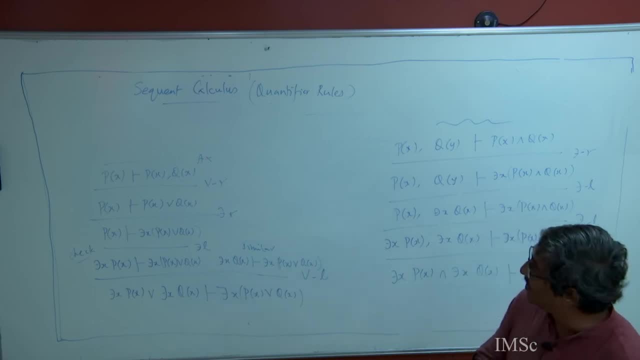 right. So last time we talked about- I mean not last time- whenever we talked about natural reduction and sequent calculus for propositional formulas, very similar ideas lift for quantifiers And The completeness we did for the Hilbert system and used the derivability of the Hilbert axioms. 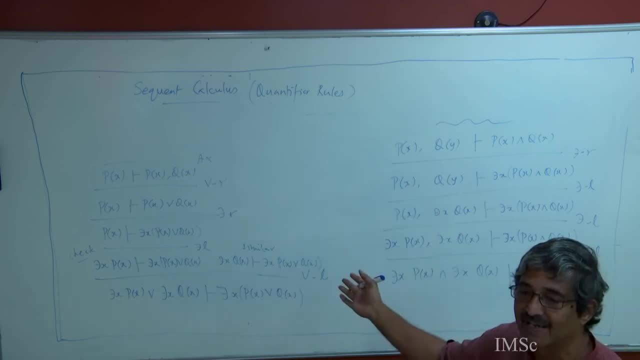 the mutual derivability right. The Hilbert axioms are derivable in the natural reduction and natural reduction one rules are derivable in the sequent calculus and the other way about and to show that they are all equivalent. But like I said, for like we did in the case, 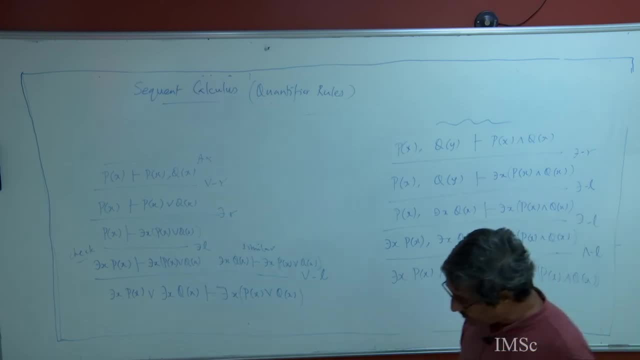 of propositional calculus. Yeah, So this is not how theorem provers work, because you know, you do not know which. there is just too much non-determinism in deciding which terms that you can make use of, and it is for this that I introduced resolution in the context of propositional calculus and I talked about 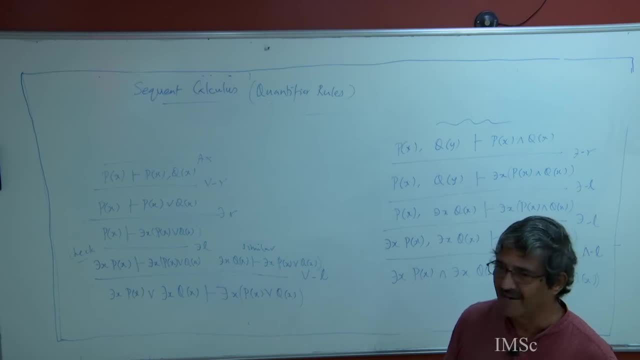 the DPLL procedure, the whatever Davis, Putnam, Loughlin, Lohmann, Yes, Yes, Yes, Yes That procedure. and then told you also how SAT solvers use those rules. Now I am not going to do a lot of resolution, but at least to get some understanding of how. 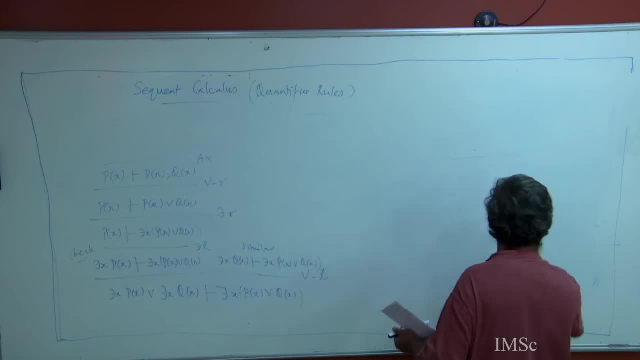 these things work. Remember Davis Putnam introduced all this for quantifiers, right. and there is also a very important you know, in the transition from going from formulas to clauses in the first order form and then doing resolution, you use a very important thing for in the 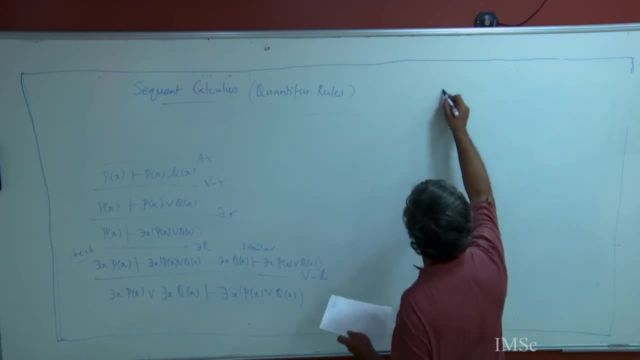 case of first order logic, and this is the idea of skolomization, And skolomization is something sufficiently important for us to learn. So I am going to talk about skolomization. So we will use these skolom functions to go from first order formulas to clauses in 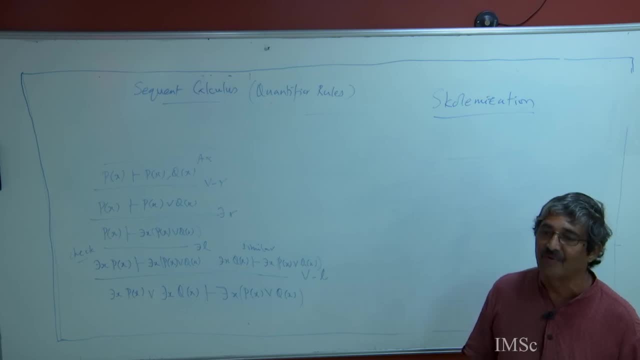 the clausal form. Okay, right, clausal form we were doing with CNF, right, the conjunctive normal form and where you have a bunch of conjunctions and each conjunct is a bunch of disjunction, right, It is a conjunction over disjunctions, right, and so that is the clausal form. 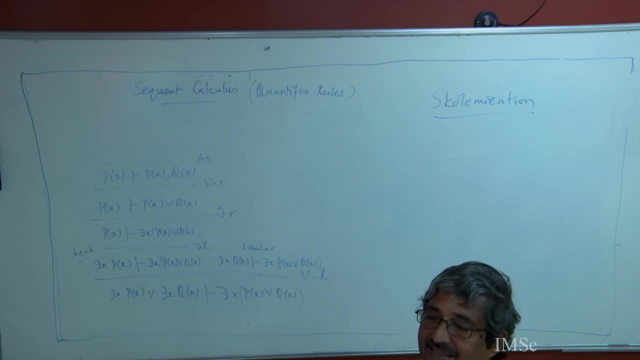 But that is a propositional form, right. and finally, you have literals. Now you are going to have literals here as well. that means you have atomic formulas or negations of atomic formulas, and you can have disjunctions of them and you take conjunctions. 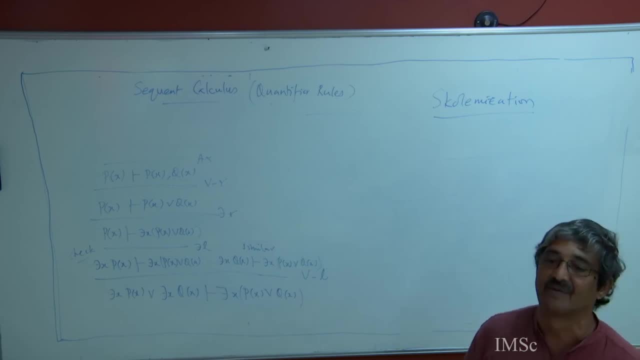 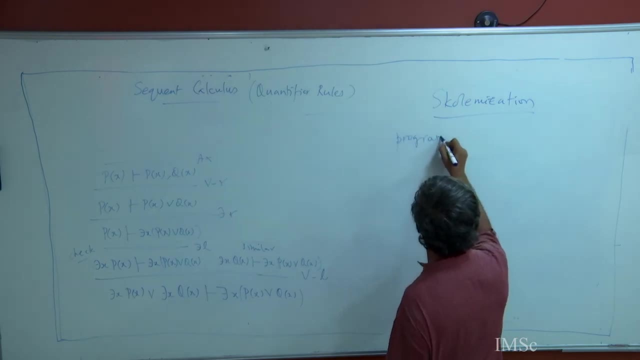 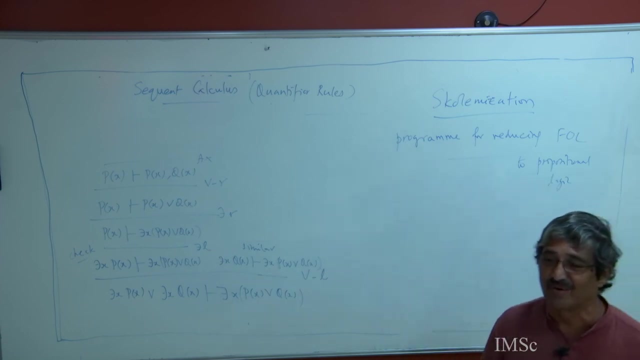 of them. But what happens to quantifiers? Scholomization is a way of getting rid of quantifiers. So scholomization, I usually call it as a program, program for reducing first order logic to propositional logic. Well, not quite propositional logic, because what do you do with all the? this is really. 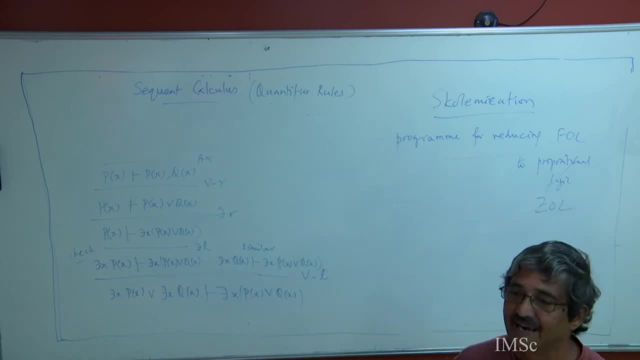 what we call Zoll, the zeroth order logic. right, where you have the syntax of constants, terms, variables, function symbols. right, predicate symbols, equality, all of these, but no quantifiers. right, you have everything else. so that is Zoll and that is what we. 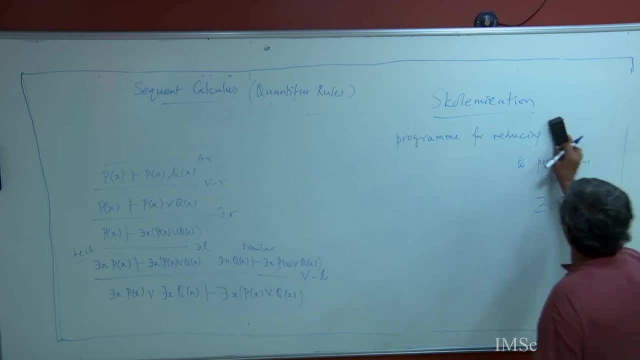 do So. scholomization is the process of doing that. How do you do this? And this is a very interesting and beautiful idea- due to scholom, of course. why else will you call it scholomization? Yeah, 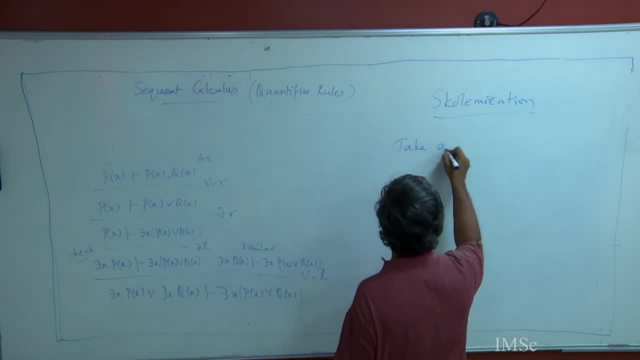 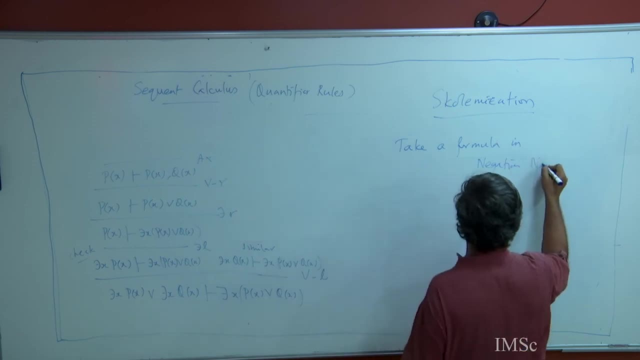 So first thing is, take a formula in negation normal form. What does negation normal form mean? Push negations all the way inside, and that is very easy to do. right, We know what is that. I mean what is not of alpha and beta, not alpha or not beta. so you, 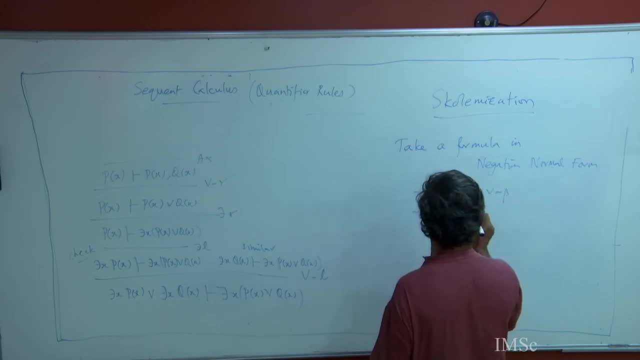 can push negation into conjunction. disjunction not of alpha implies beta is alpha and not beta, not of for all x. alpha is: there exists x, not alpha. not of there exists x. alpha is for all x, not alpha, right Ok? 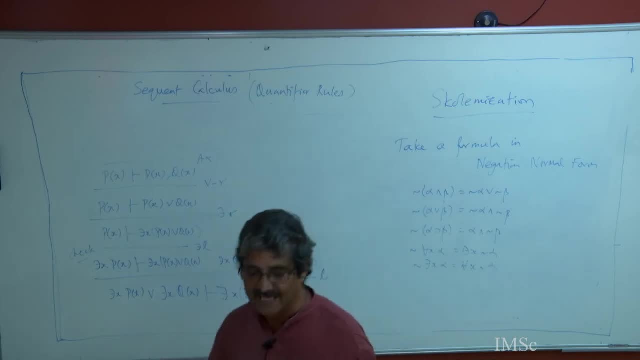 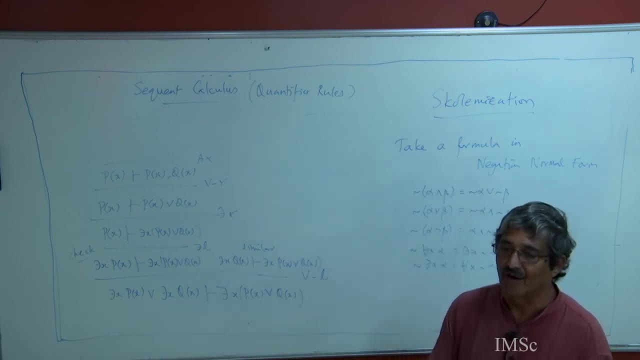 So you can always push negations inside. So let us so, by which I mean we assume that negations occur only in front of atomic formulas, right? So you have T 1 equals T 2, so the syntax is: T 1 equals T 2, T 1 not equals T 2, P T. 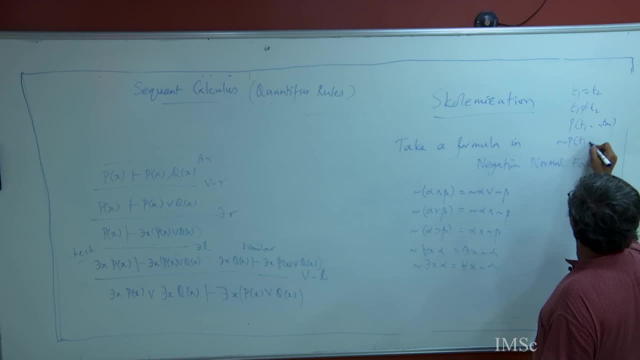 1 through T m, not P 3, 1 through T m and then disjunction, conjunction, implication, Ok, Ok, So you have implication, if you like and why you have implication. right, we want it in clausal form. so it is enough to have only conjunctions and disjunction, and then you. 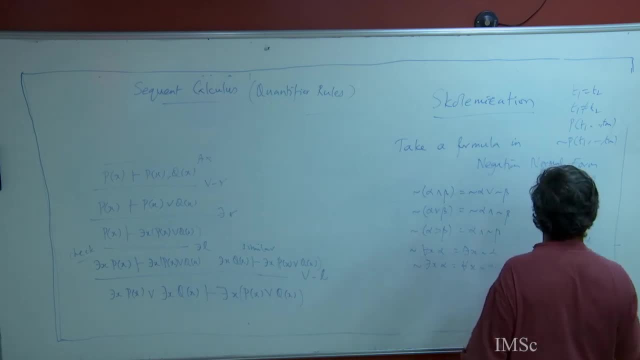 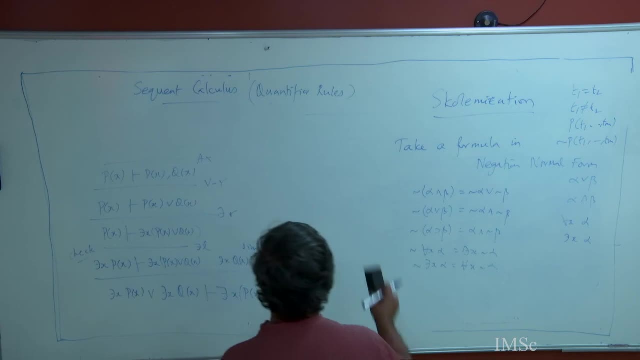 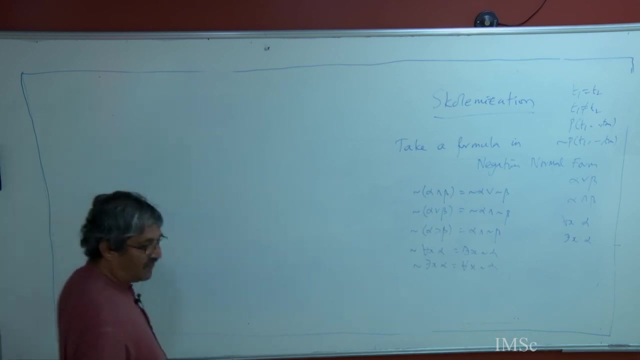 have for all x, there exists x. these are the only possibilities. Now consider any occurrence of the existential quantifier. 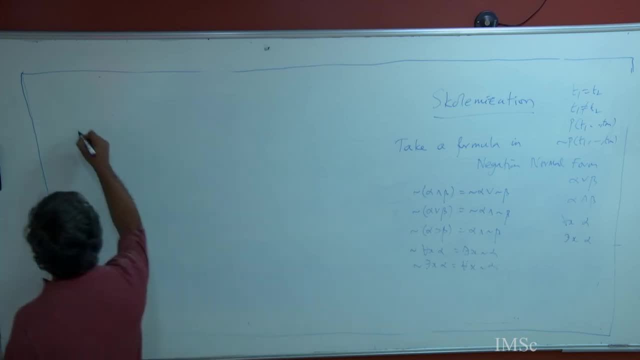 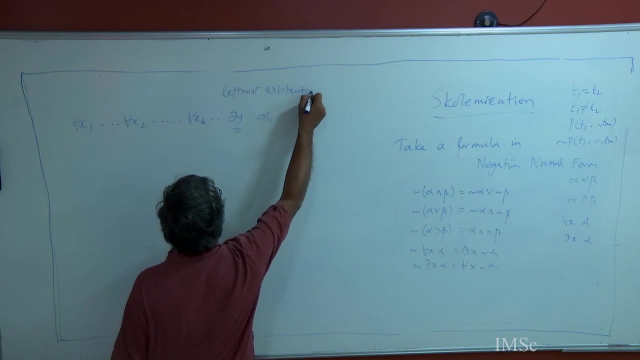 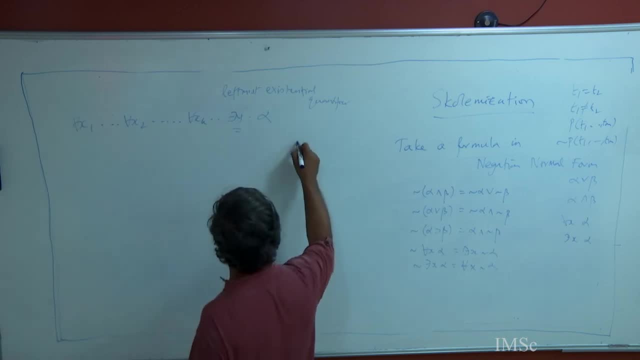 yeah, with k greater than or equal to 0.. Yeah, that means that the existential quantifier, if, if the formula has an existential quantifier at all, look at the leftmost fellow. before that, look at all the universal quantifiers there are. there may be none, right? So now the idea is: 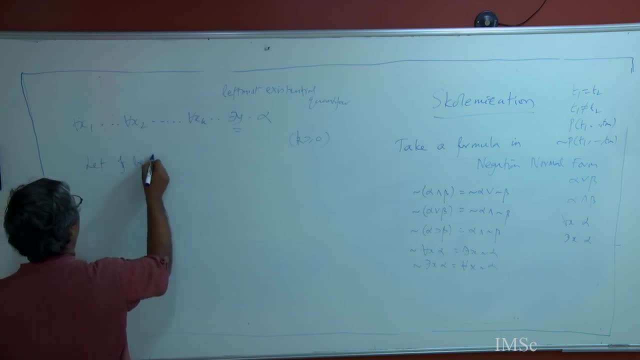 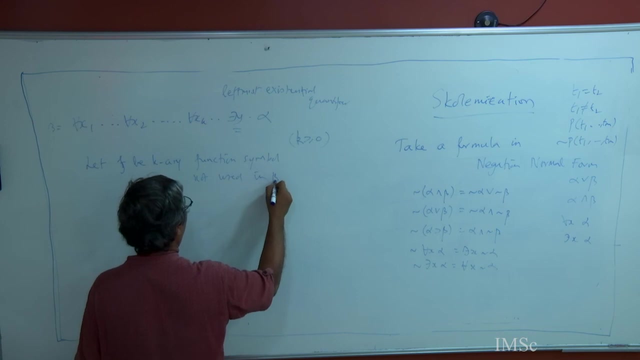 this- let f be a carey- function symbol not used in the formula. So let me call this formula beta, where we are beginning. Take a new function symbol not used anywhere in the formula and replace now. So beta prime is the formula, say in the formula. 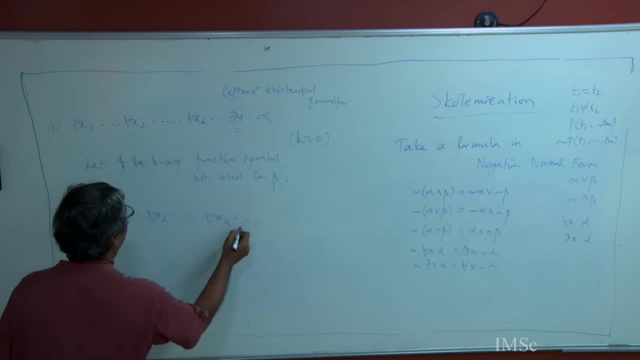 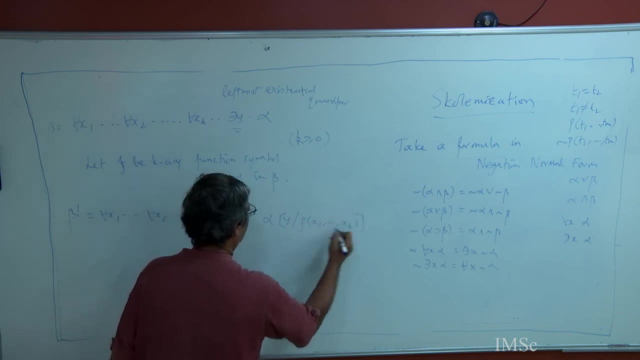 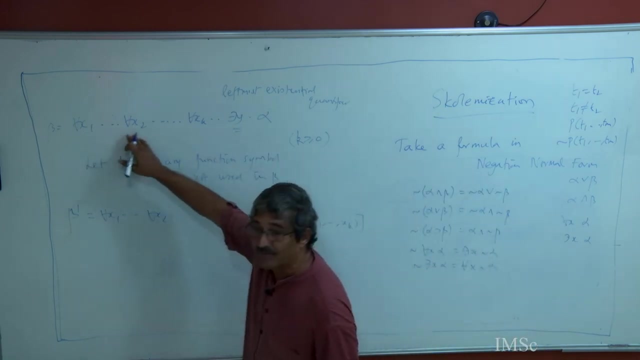 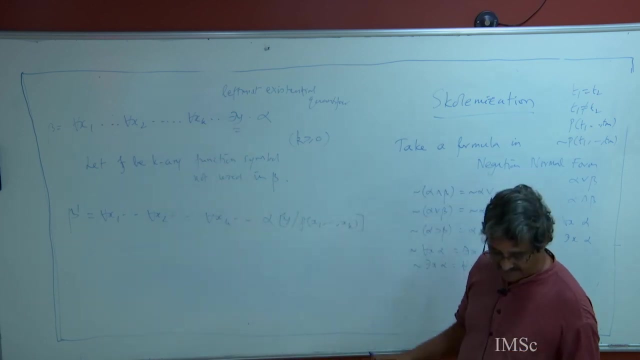 Same thing for all x 1 for all x, k and alpha, with y replaced by f of x 1 through x k. Why? Because this existential quantifier y depends presumably on all these x 1 to x k. So replace it by f of x 1 to x k. So that is the idea. So, and now? if k equal to 0,? 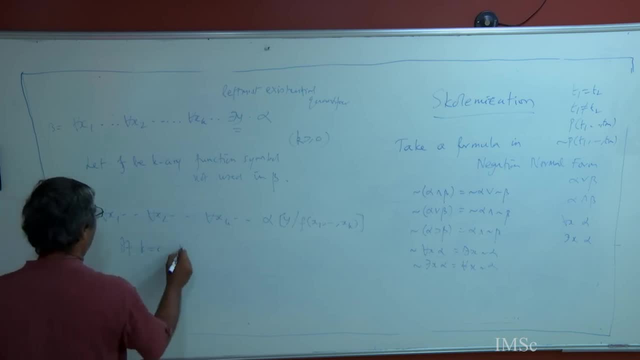 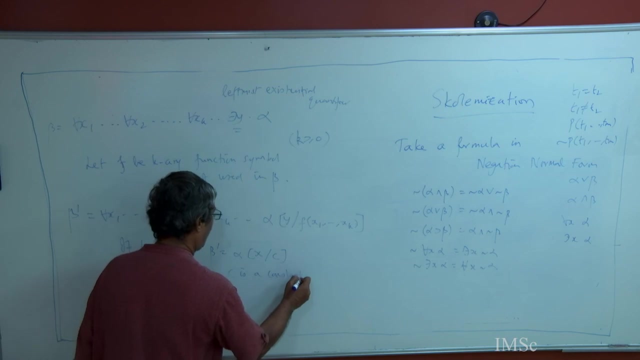 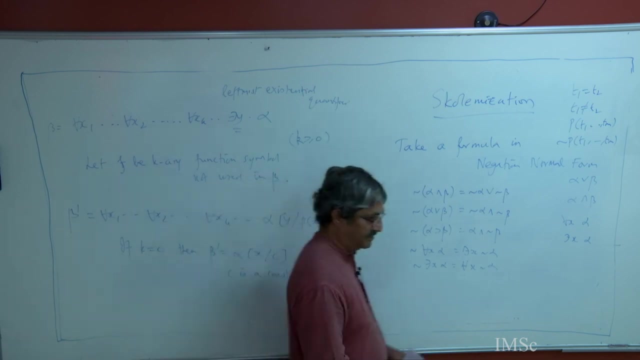 then the formula beta prime that you are looking at is simply alpha, with x replaced by some constant symbol, c. c is a constant symbol not used in alpha. Yeah, if there is nothing else to the left of the existential quantifier, there is no solution Not used in beta. 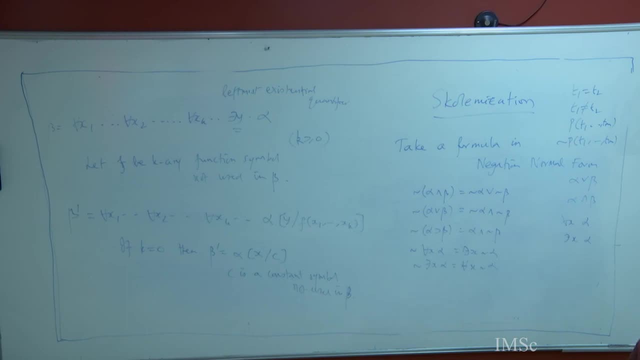 God knows what context this existential quantifier is in. Yeah, So this is the idea of skalimization. Look for the existential quantifier If it does not depend on any universal quantifier at all. replace y by some new constant symbol, c. This is the idea of witness fulfillment right. 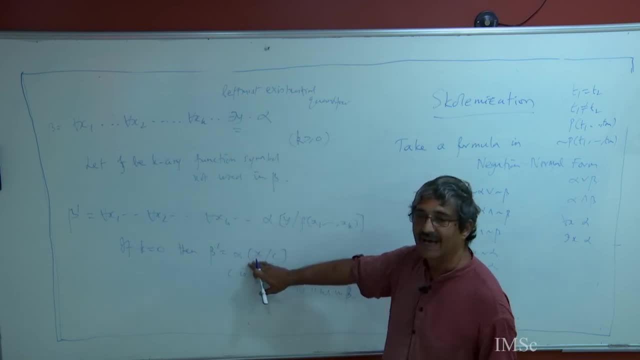 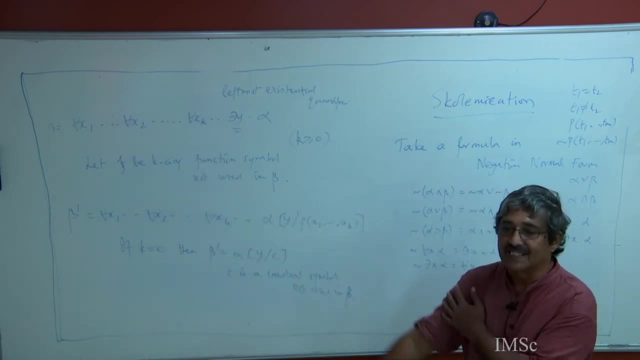 There exists y alpha. so if you have a non-existential quantifier, there exists alpha. There exists y alpha, replaced by y. this is not x. yeah, So for the existential quantifier you are providing a witness. What is the witness? Some new symbol? this is what we have been talking about, right? 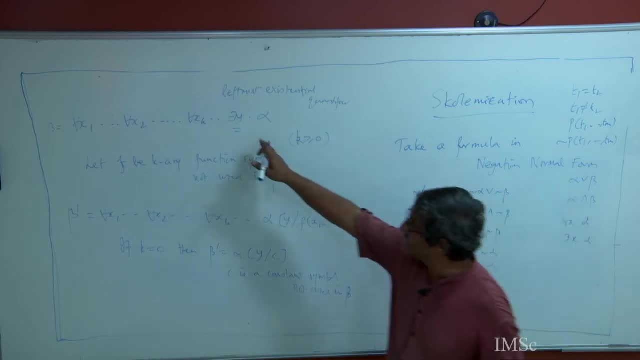 all along. You cannot do it in general because this fellow may be dependent on whatever is the universal quantifiers that you have seen before. in that case you choose a function symbol, So existential quantifiers are eliminated using constants and function symbols that. 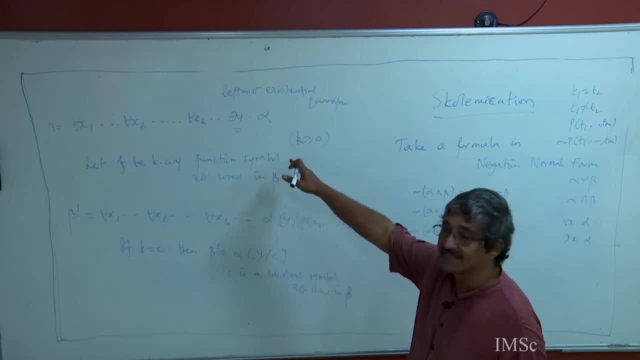 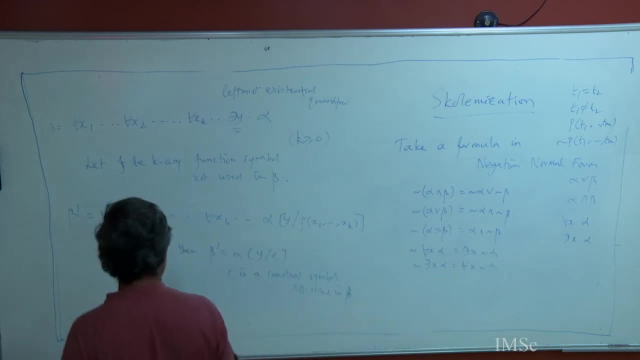 is the deal right? Well, you got rid of one existential quantifier. apply repeatedly. What will happen At the end of this exercise? you do all of this and you will get a universal formula. I have written for all x bar to say that you will have only universal quantifiers. 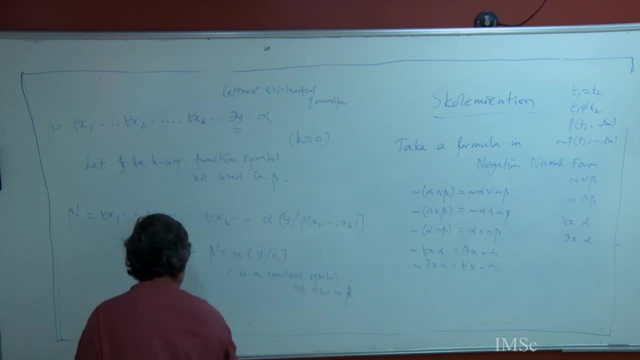 in the formula right, Then drop the universal quantifiers. So after repeat until all their exists are eliminated. By this process you can eliminate all the existential quantifiers. Now you have only universal quantifiers in the formula. So you can only drop the universal quantifiers. Now you will have a Zoll formula right. So 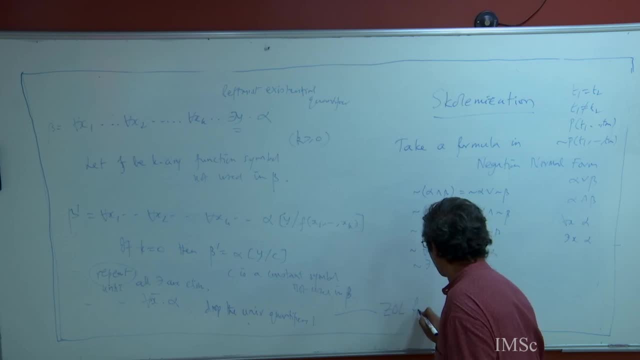 this is a Zoll formula because it will have free variables. it will have. all free variables are now implicitly, universally quantified. that is the idea, right, and that is it. It is a very simple and beautiful process and by which you can, But what have you done? 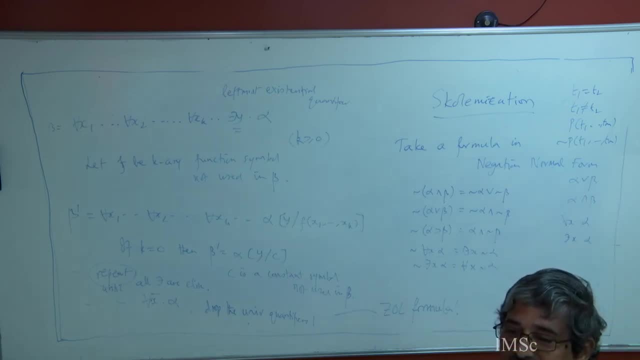 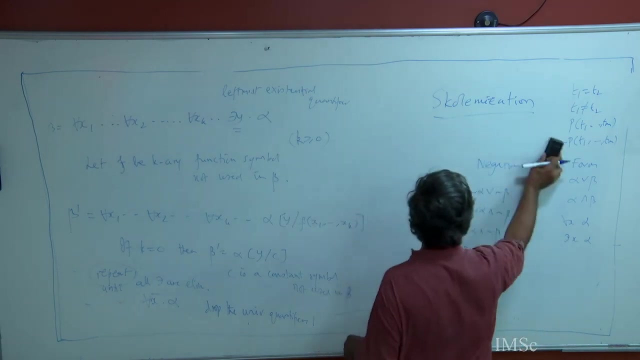 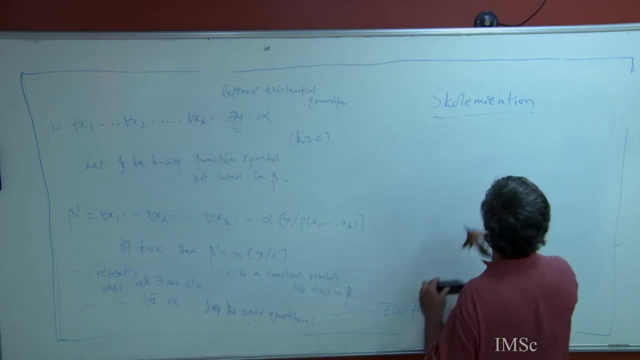 You have done in the process right. You started with the formula beta and you have come up with the formula beta prime. What is the relation between the two? Well, take a very simple formula. 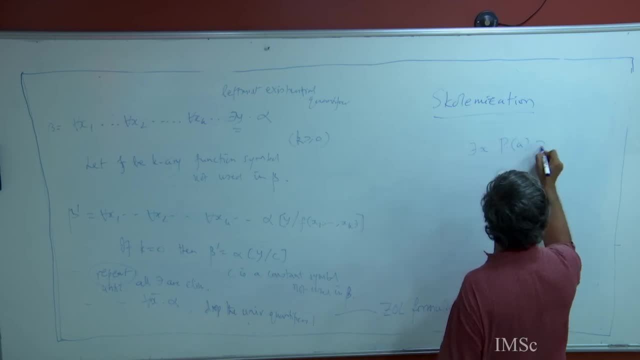 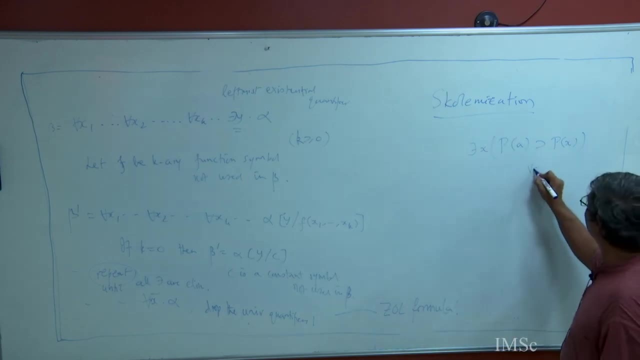 Now, this is a valid formula. Can you see that it is valid? There exists x, pa implies p x. I mean, I am going to assume that I will only know an empty domain. so so that from now, 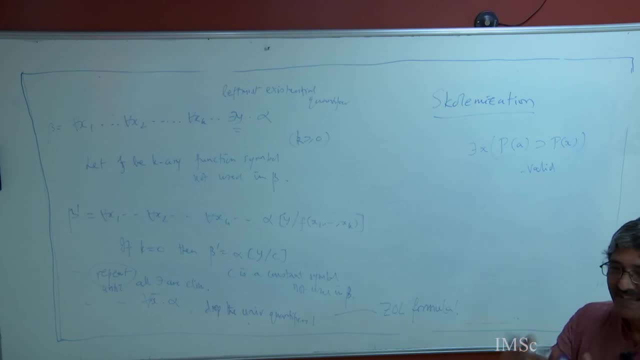 on create some hassle in. by the way, in natural reduction, second calculus, when I am doing proofs or when I am doing resolution, you always assume non-empty domain. Empty domain is a pain that needs to be taken care of separately, So let us just make that assumption. yeah, 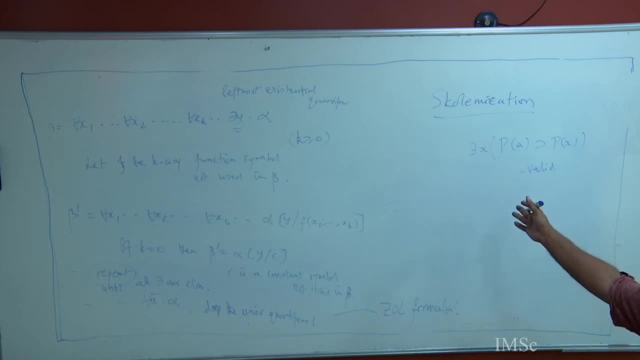 So now this one is perfectly fine, right, You have some element once you have A is true, of course. you know there is Px is also true, right Now, what I do scolomize, what will I get? I will get Pa implies Pb. this is of course, not valid right, Just because 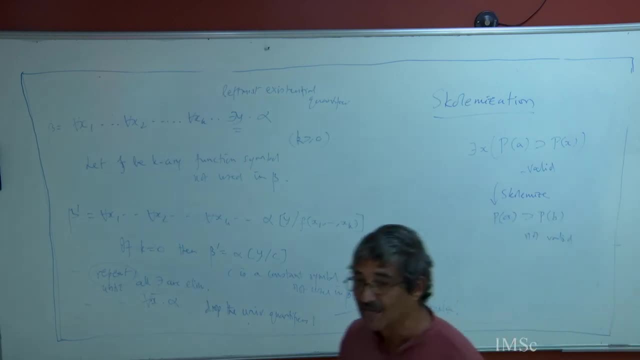 you know, P is true for A, it does not mean that P is true for B as well, right? So scolomization does not preserve Pb. What it does, It preserves satisfiability, and this is very important to keep in mind. 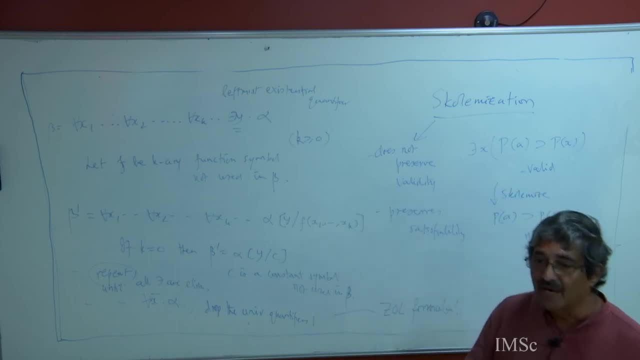 Scolomization is a very natural process. What it preserves is not validity, but consistency. This is how you would say satisfiability, yeah. So what it means is that if you start with the formula beta and applies scolomization, 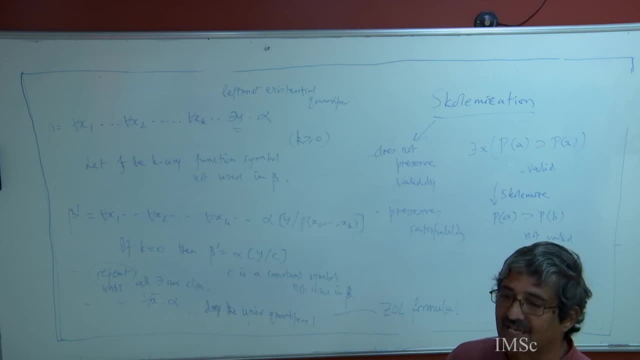 you get a formula- beta prime- such that beta is satisfiable if and only beta prime is satisfiable, right? But it is not about truth in all models, in about a particular model, And that it preserves satisfiability should be obvious, right? Why Suppose there is? 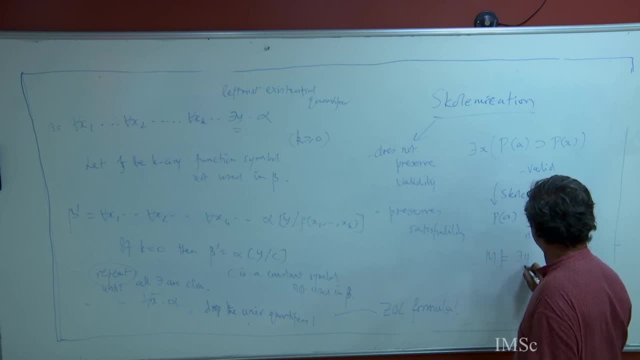 a model M, it satisfies there exists. Suppose it satisfies there exists. suppose it satisfies for all x there exists y, alpha. Then what does it mean Then? for every element of the domain right, such that you choose right, x is assigned. 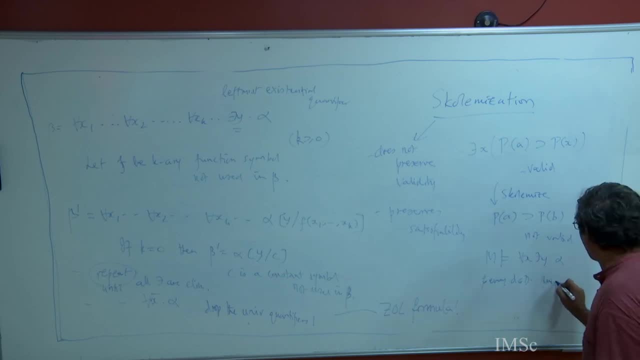 D. There exists some d prime belonging to D, such that M with x assigned to d, y assigned to d prime satisfy alpha. And of course, therefore, this if and only if, for some function d from d to d, for some f function f, d to d, if and d belonging 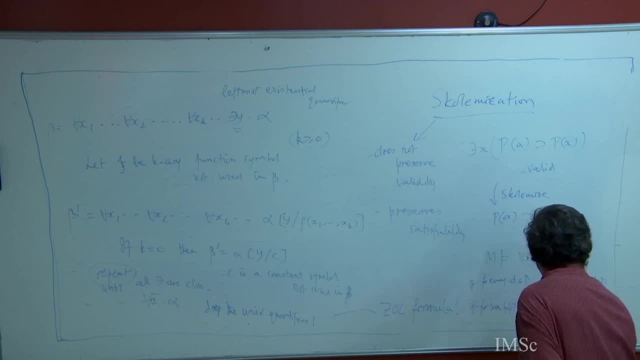 to d, m with x, y with f, d satisfies alpha. So that is why, if for all x there exist, y alpha is satisfied, then this column form, alpha prime, is satisfied as well. So this is the idea. So it preserves satisfiability, but it does. 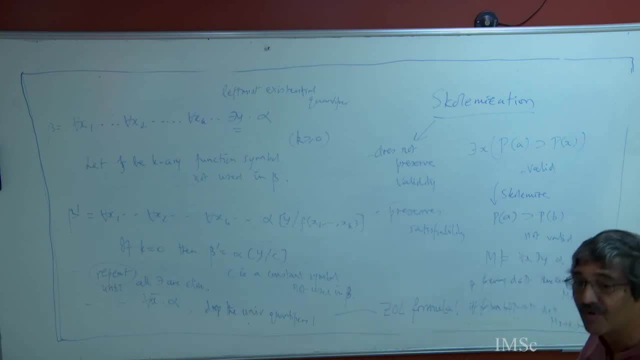 not preserve value. To move over, you may have to go to a different model, right, because remember that there are all kinds of functions possible. This is that for some function, right Now that function, you can choose many, many different functions. that from d to d, that will make this true. 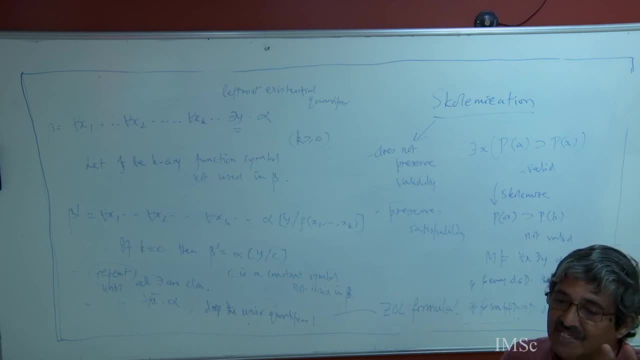 and each of this will give you one model right. So, from the original model that you have gone to, you have gone to different. that is exactly what happens here. This is from the model that made it true. you moved it to a different model.